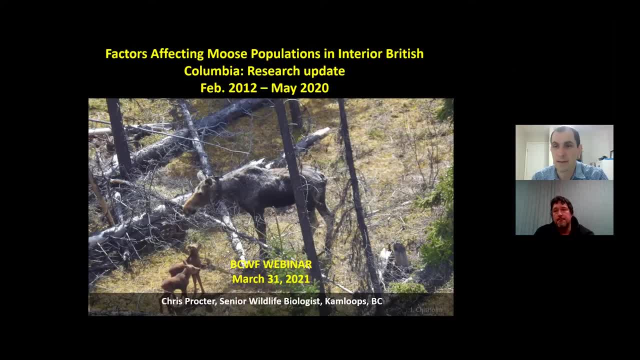 to an hour. We will have some question and answer after that. We won't go past 8: 30. An hour and a half is plenty long to be on Zoom staring at a screen. You can ask questions in the Q&A function on your toolbar. 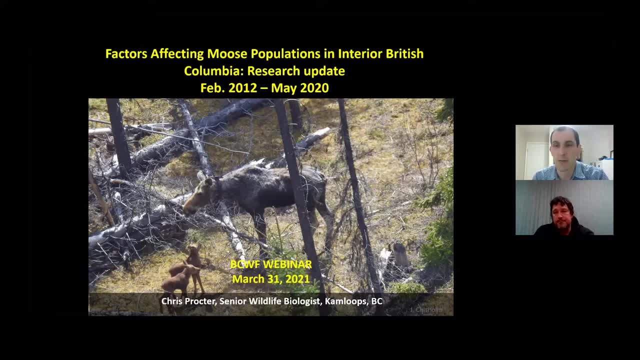 We'll be able to track those. as Chris is presenting, There will be questions that overlap with other questions that we get from Facebook or on this platform, So we'll be aggregating them if there's a lot of overlap. Keep in mind that Chris is a biologist and not a policy maker, So if you feel, 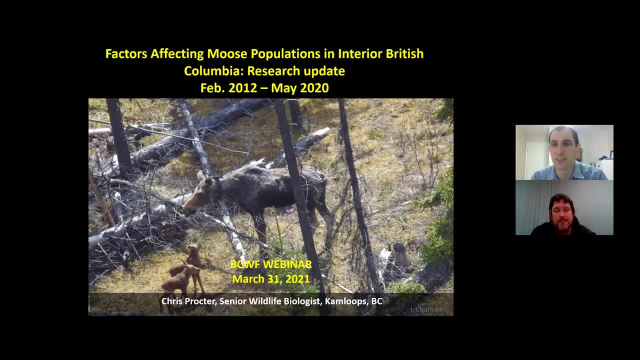 like your blood pressure is rising and you really think that something should be done to change the trajectory of moose or that can be done to help moose. Chris can't make those changes necessarily to give us the evidence. So if you feel your blood pressure rising, keep in mind that it's the 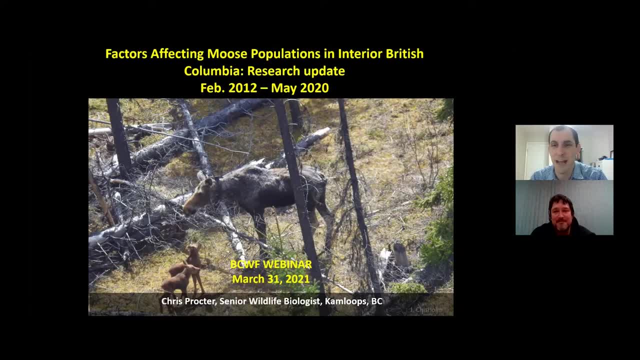 provincial government that makes most of these decisions and that. so, again, this is to give you evidence in terms of what's happening. Chris will outline this, but there's going to be a lot of questions, or maybe some questions that he can't answer. There's a whole bunch of data and papers. 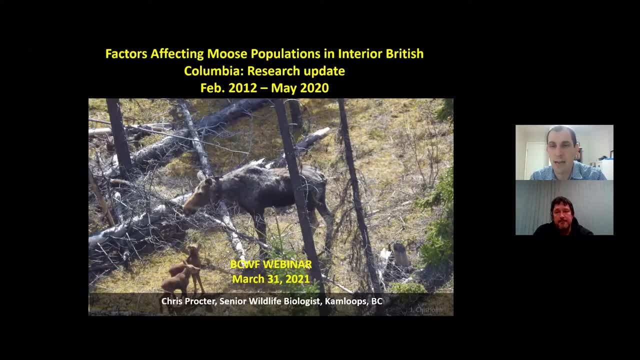 that will be coming out here. So we're kind of at the front end of the results of the moose project. maybe for an update again a year or less from now when a lot of the papers have been published. So about Chris? Chris Proctor is a senior wildlife biologist with the Fish and Wildlife section of 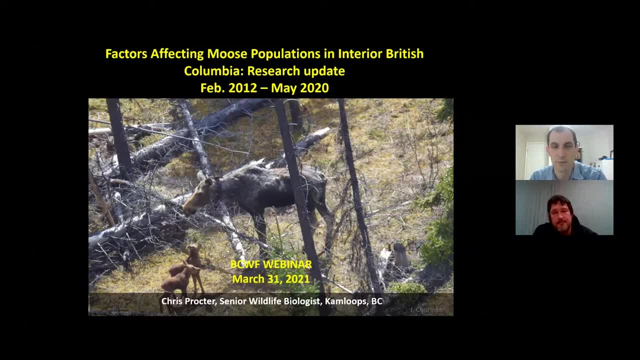 the Ministry of Forest Lands, Natural Resource Operations and Rural Development in the Thompson Okanagan Region. He has more than 15 years of wildlife related field management experience, including 15 years with the Ministry. He has been based in Region 3 for the last 13 years. 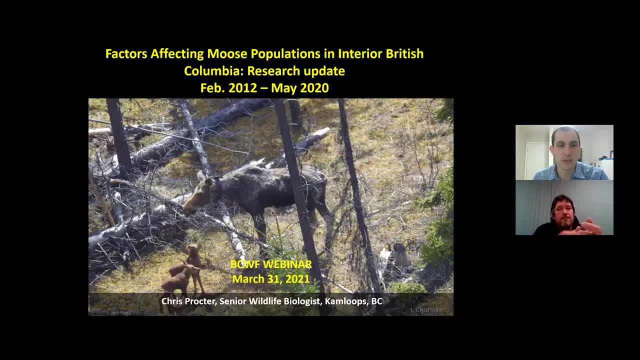 The majority of his work focuses on the conservation of wildlife. His work focuses on ungulate harvests and population management and research. I'm going to turn things over to Chris and, as stated, if you have a question, feel free to put it in the Q&A or in the chat box, if you're. 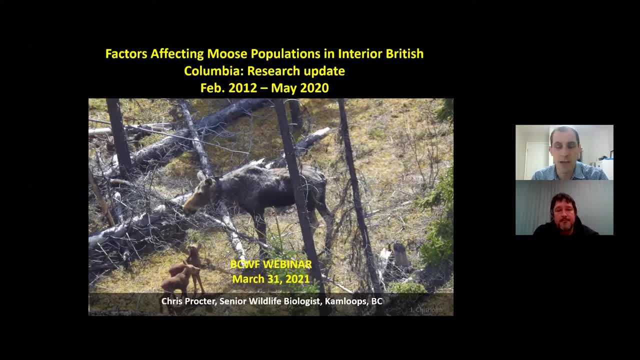 coming in from Facebook live and I will do my best to aggregate everything and then get to that at the end of Chris's presentation. So thanks, Chris, for giving us some of your time on a evening and again, thanks, Martina, for all the work you do. Thanks. 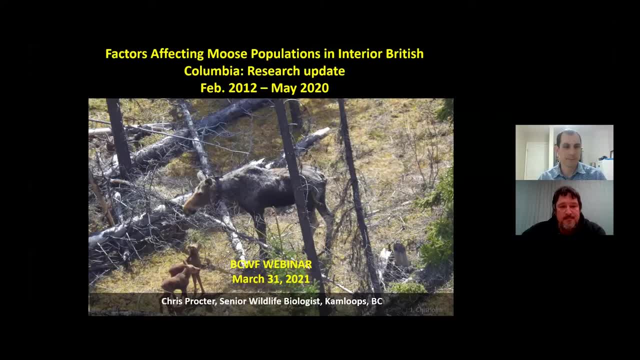 So, Chris, over to you. Thanks, Jesse. Hey everybody, thanks for tuning in tonight. I'm here tonight, as Jesse said, to provide an update preliminary results from ongoing moose research in interior British Columbia. I've been involved in this project since it started back in 2012, mostly as the study area lead for the Bonaparte study area north of Kamloops. 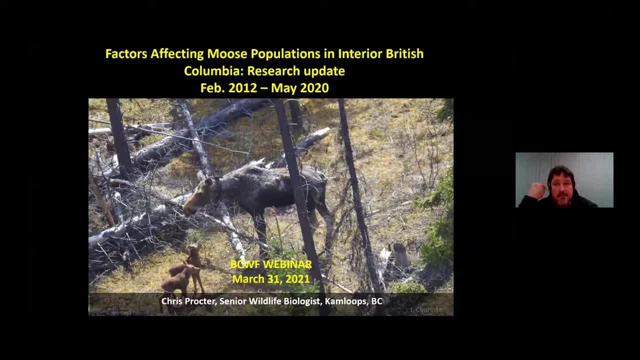 I've kept the presentation focused on what we've done and learned so far in our pursuit to examine the effects of landscape change or intensive forest development on moose populations. There is associated work going on in some of these study areas, namely the John Prince Research Forest in association with UNBC, that I will not be talking. 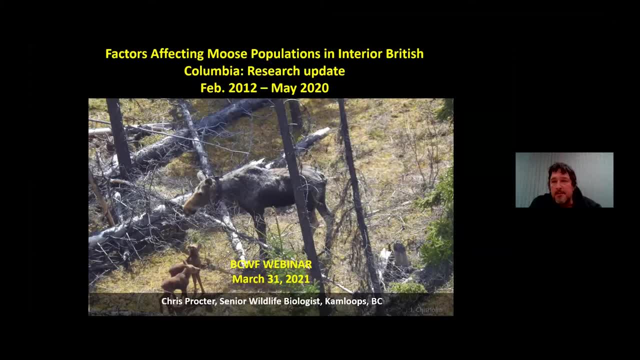 about tonight, So mostly capital. I'm here to talk about some of the things that we've done to answer those original questions that we set out to answer. Again, as Jesse mentioned, a lot of the results are currently being written up so I'm not going to speak to those much tonight. 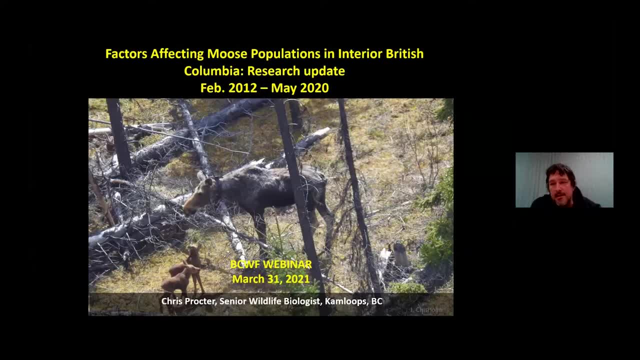 And finally, a lot of the data presented here is preliminary in nature. Analyses are still ongoing, Data are still coming in And conclusions are subjective. They're still ongoing, So we're going to keep that in mind. Please, A bit of an outline here. 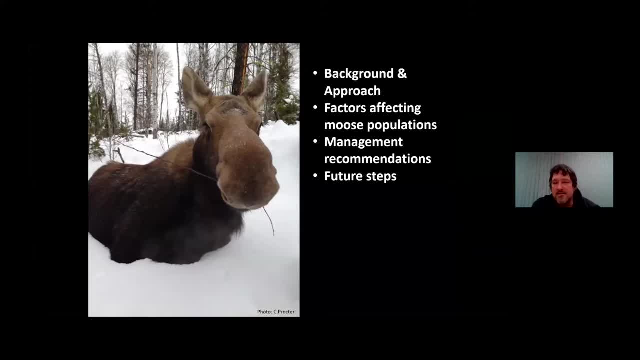 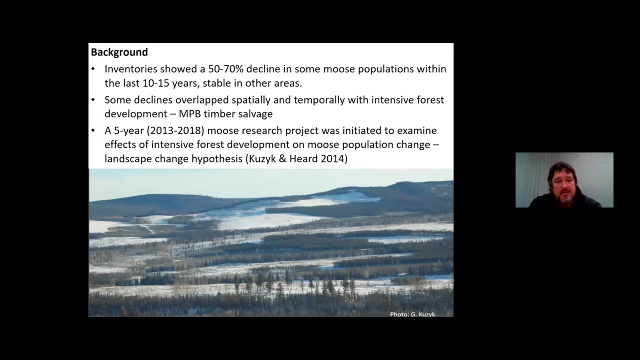 I'm going to talk about the background that led us to this project, Our approach, our methods, some results, the management recommendations that have been published to date, And I'm going to talk a little bit about our future. So, background: as you know, and as Jesse mentioned, we've seen some pretty significant moose. 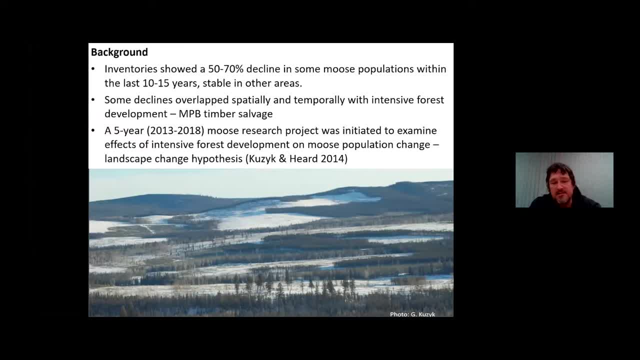 population declines in the province up to 70% in some areas. A lot of those declines seem to overlap, both in time and space, with landscape change associated with pine beetle timber salvage over the last decade or more. I'm going to talk a little bit about that. 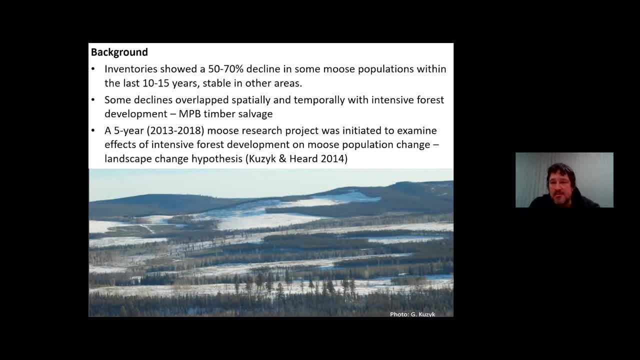 I'm going to talk a little bit about that. I'm going to talk a little bit about that. You know, back when that was starting, we had a ton of concern from First Nations, our stakeholders, even to the point that legal injunctions were granted to stop logging in some places, for example, 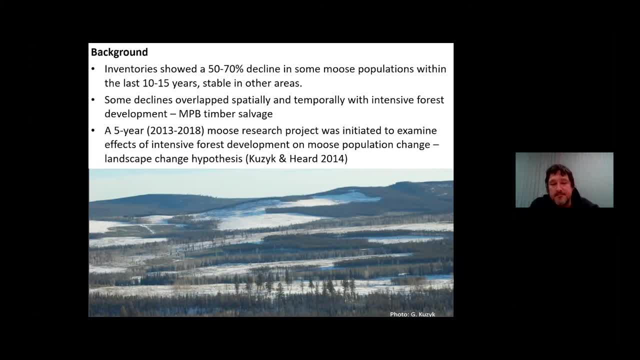 We implemented this research in response to those concerns in 2012 in the Bonaparte study area and a year or two later in the other study areas across the province. The focus of the research, as I've mentioned already, was to examine the effects of that intensive forest development on moose populations. 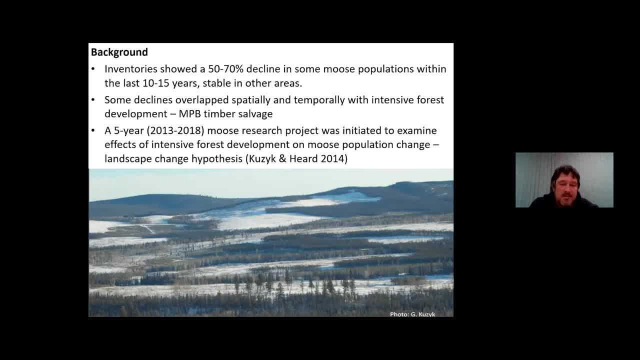 Up until that point we had generally thought that logging wasn't necessarily a bad thing, for moose tends to open up the landscape, provides forage for moose and certainly in the past we had seen moose populations respond favorably to logging. 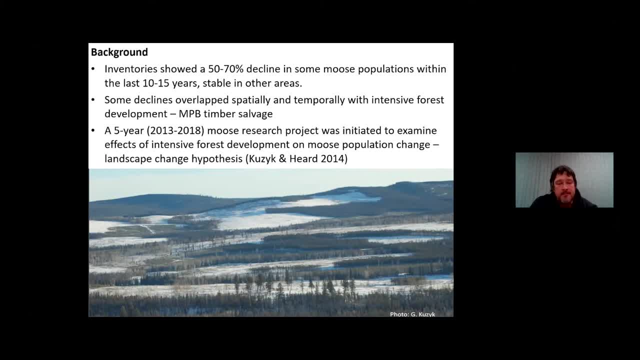 This logging was a little different, As you know, much more intensive than anything we'd seen in the past, And in looking at it, it wasn't hard to imagine that it could affect moose differently. So that's what we set out to answer. 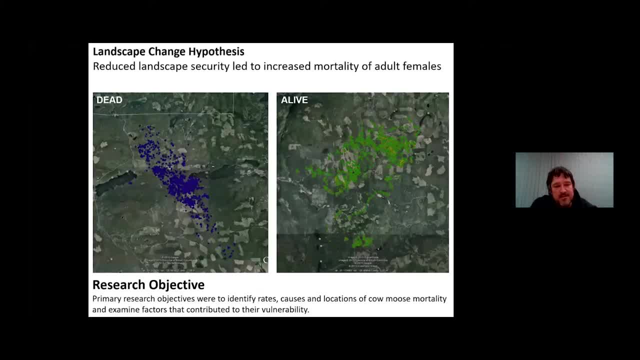 We developed a landscape change hypothesis to test. That. hypothesis suggests that reduced landscape security due to the presence of roads, Cut blocks, The primary infrastructure associated with logging, increased moose vulnerability and mortality. Given the potential mechanisms involved, both roads and cut blocks, we predicted predation and hunting would be the dominant mortality factors. 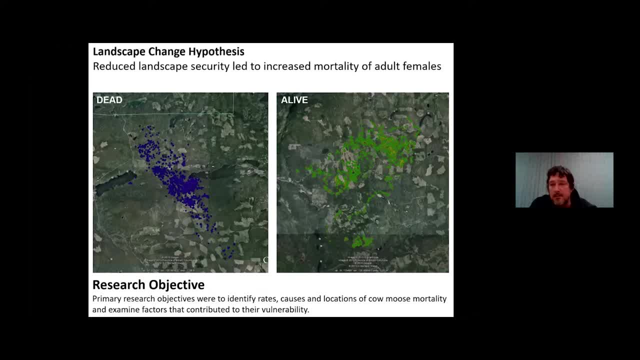 Those are also the two mortality factors that we hear a lot about from people out on the land. We focused on Female moose- adult female moose- initially, largely because we didn't have the resources to include calves at the time, but also because we reasoned that female survival was likely involved, given how rapid some of these moose populations declined. 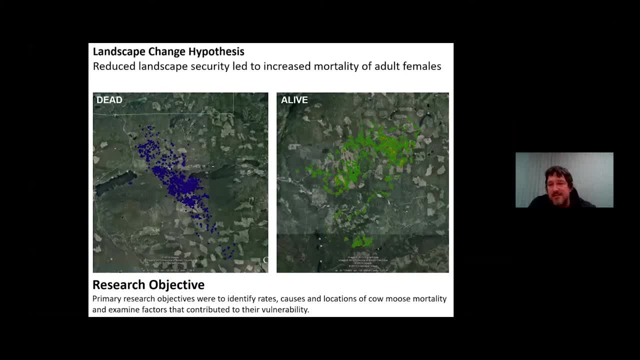 Also given our hypothesized mechanisms specifically around hunting, Because most antlerless hunting seasons are focused on adults as opposed to cows. Our primary approach was to monitor the rates and causes of moose mortality, locations of mortality and examine the factors that contributed to that mortality, particularly in the context of landscape change. 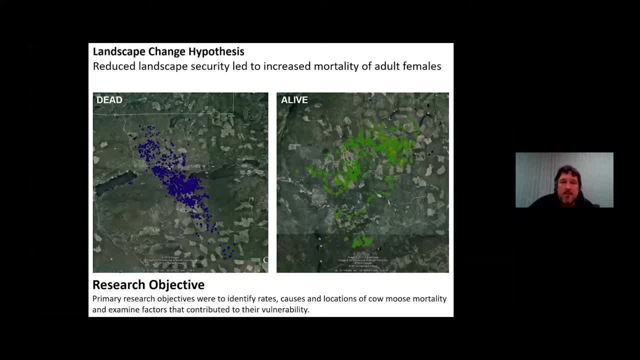 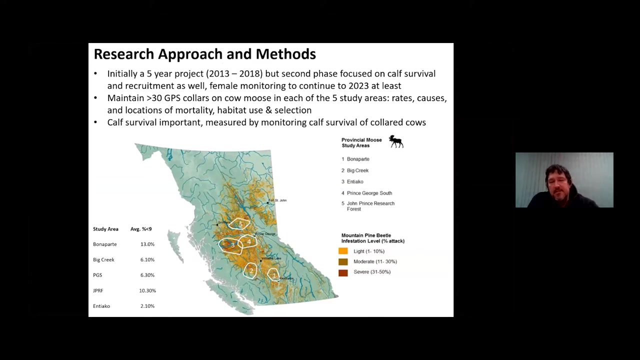 Just an example in the image that you see there. we were interested in understanding How moose use these landscapes And how these landscape disturbance features might contribute to their mortality and causes of death. We selected five study areas across the interior portion of the province, trying to capture that variation in. 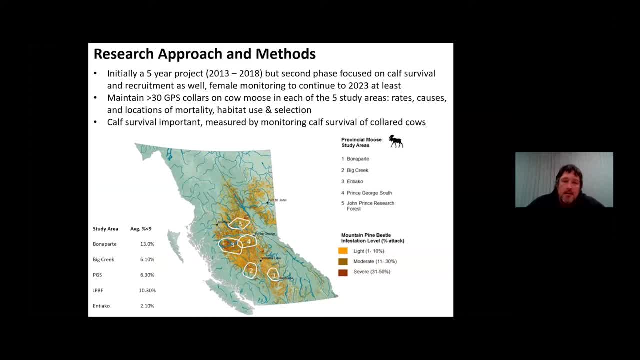 Landscape change. They are the Bonaparte Plateau northwest of Kamloops, The Big Creek Study Area west of there and southwest of Williams Lake, Prince George South, southwest of Prince George, The Antiochus Study Area west of that one, south of Smithers. 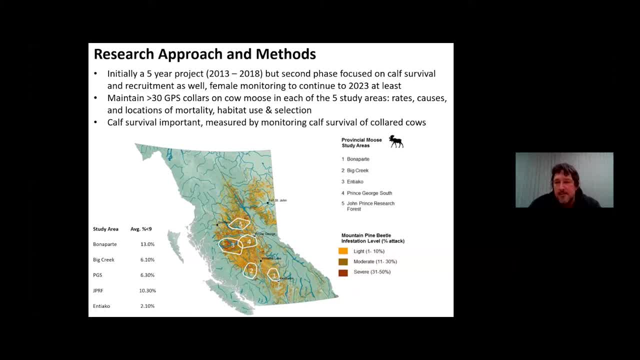 And then finally, the John Prince Research Forest northwest of PG. That table you see on the left Is one metric of land use. And then finally, the John Prince Research Forest northwest of PG, The. We attempted to maintain a minimum of 30 cows. Radio collared and monitored in each of the study areas and we also tried to do a practical study, of which was one in which a lot of the data was in Lenscape change. It is the proportion of those study areas that is in early serial condition, less than nine years of age, fairly variable, varying from 2% in the Antiochus Study Area to 13% in the Bonaparte Study Area. 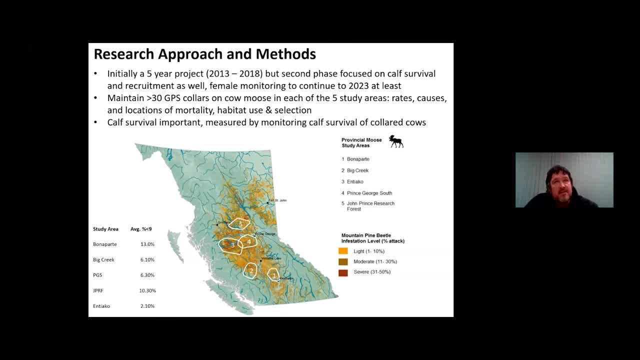 these study areas. um, often, in some years, we had uh 50 or 60 on the air. um, i think we pretty much achieved that in all years. um, and then the approach was, like i already said, to monitor rates, causes and locations of mortality. um, we recognize that, calf recruitment being the other half of the 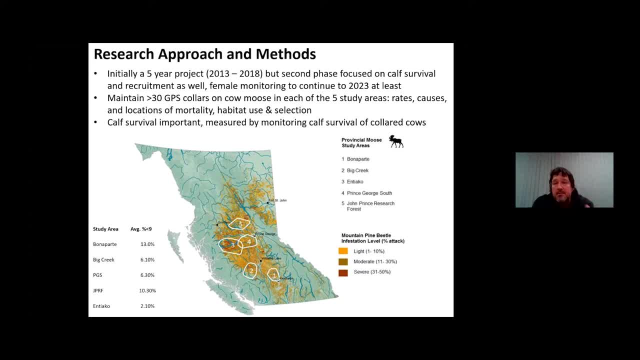 equation that may contribute to how moose populations are changing. um was important. we did not have the resources, as i mentioned, to monitor calves at the outset, um, and instead we focused on monitoring survival of calves from collared females and later, which, which i'll talk about later- um, we did actually start putting collars on older cows. 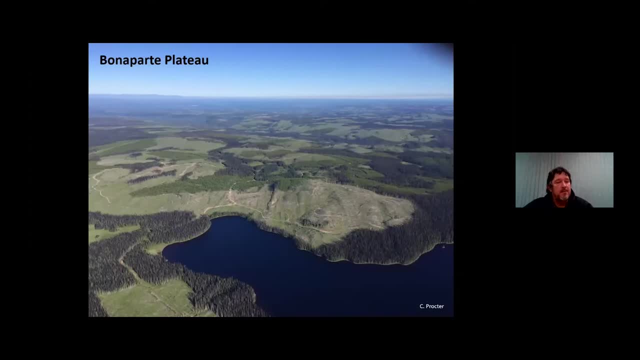 um. um, for those that might be unfamiliar with the uh status of these landscapes or haven't have never been to these study areas, i have a few aerial shots, um, just to give you an idea of what these landscapes look like. um, they vary quite a bit, not only in their? um level of forest development, but also in other factors. um climate predator communities. 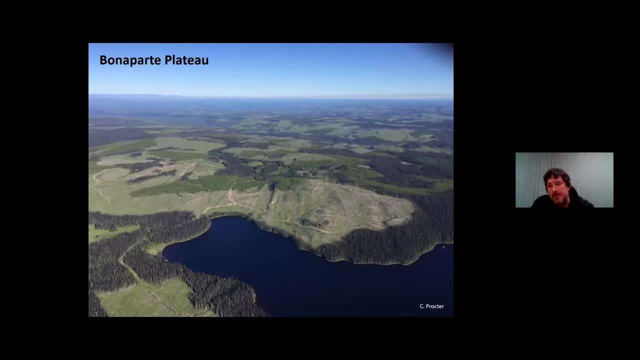 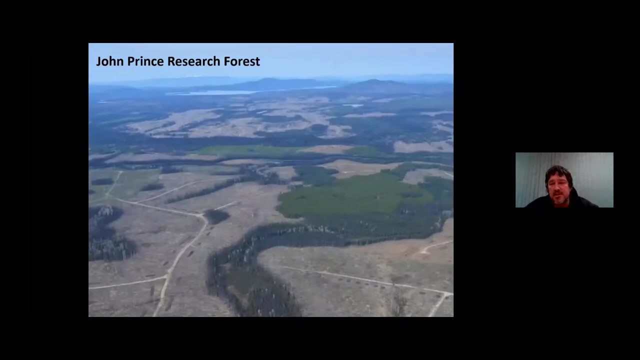 wildfire, um that kind of stuff. anybody interested in the specific details on how these study areas differ um can get that information from our progress reports. so first one here: bonaparte plateau? um north of kamloops. john prince research forest northwest of pg. um prince george south, um southwest of pg. 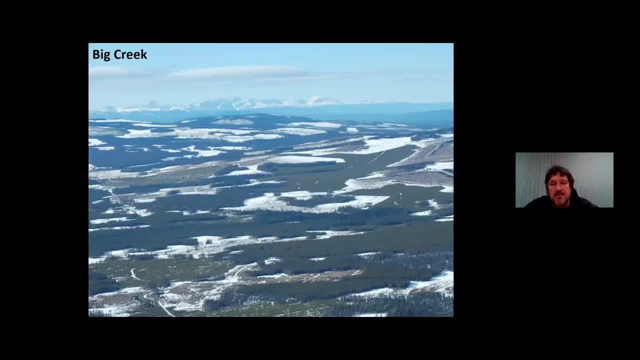 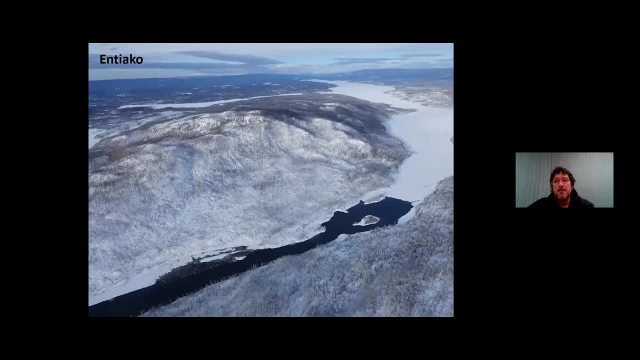 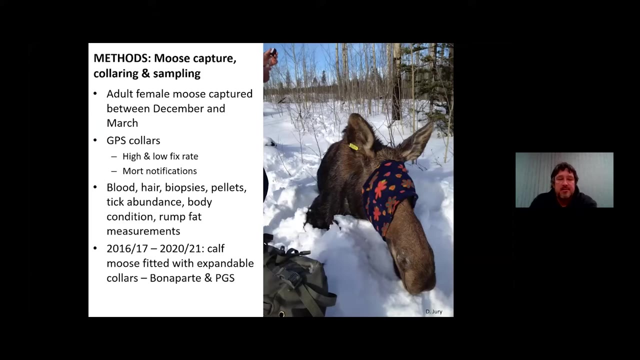 um the antioch study area, south middle east, um big creek study area, uh west southwest of williams lake and the antiocho study area. uh, a little bit on our methods um moose captures. we we captured, we attempted to capture moose randomly on the landscape during the winter months, um by either neck gunning or aerial darting. 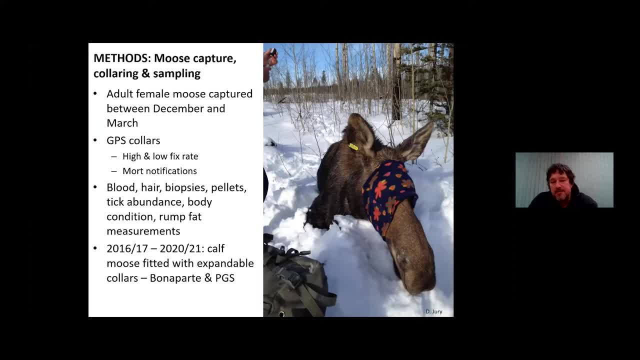 We deployed GPS callers on every moose we captured. Some were high fix rates, some were low fix rates. All callers were able to give instant mortality notifications via cell phone email, so we knew when these callers stopped moving and then we could check those sites out. We collected a bunch of samples at time of capture. 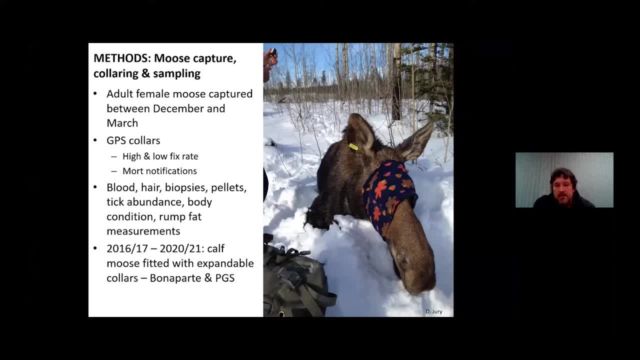 to give us an indication on the health and general condition of moose. These included blood, hair, ear biopsies, fecal samples or pellet samples. We counted winter ticks as a measure of their abundance on individual moose and we did various assessments of their body condition, including actually measuring how fat moose were. 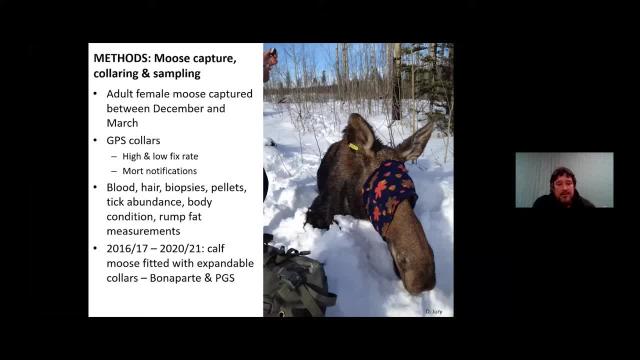 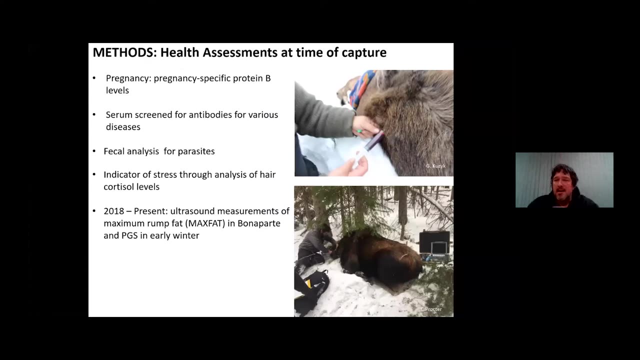 Directly with an ultrasound. In later years, which I'm going to get to, we did put callers on moose calves and monitored their survival rates through the winter From these samples at time of capture. we've analyzed a range of things From the blood samples. 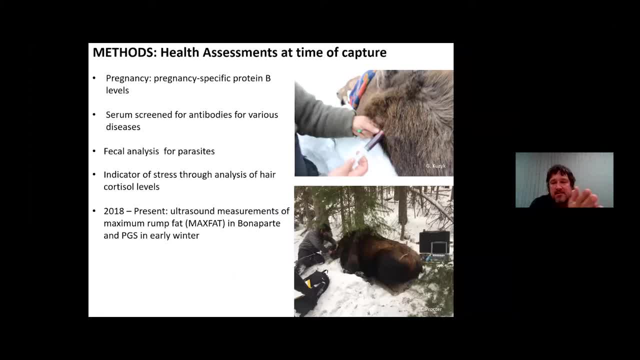 we've analyzed pregnancy rates via pregnancy specific protein B levels in the blood serum. We screened serum for a whole range of diseases that moose may get. We analyzed those pellet collections for parasite burdens, hair samples. We analyzed cortisol levels as an indicator of stress those animals are experiencing. 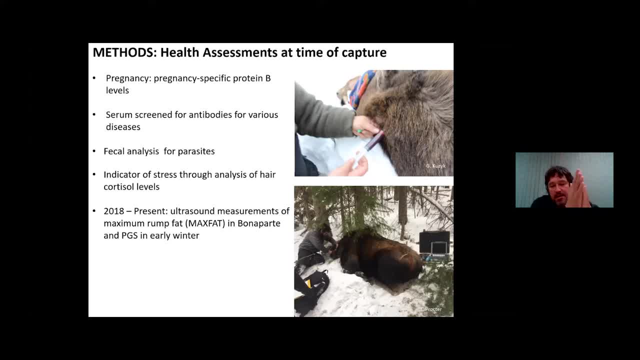 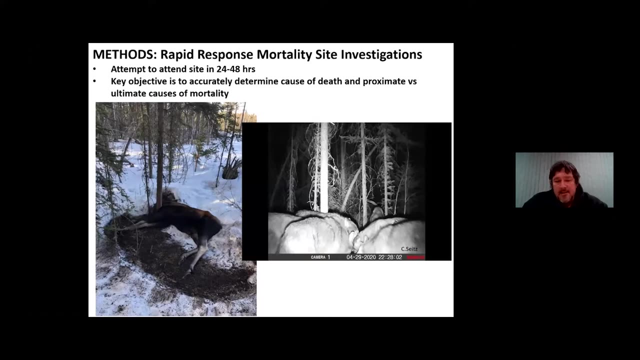 And, as I mentioned, we've in the last three years we've been measuring rum fat on these cows directly. in two study years, Bonaparte and Prince George cell, We attempted to attend mortality sites as fast as we could, ideally within 24 hours. 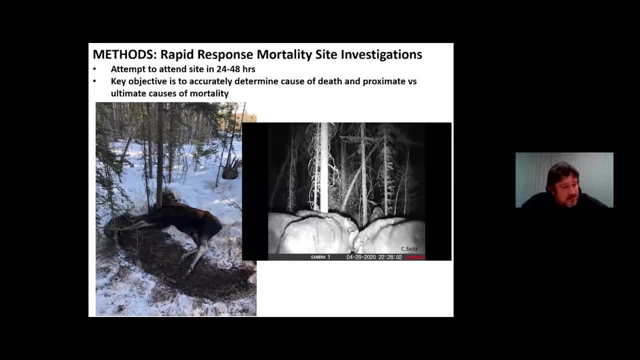 maximum 48 hours kind of thing. Our objective in doing these mortality investigations was to both accurately record how those moose died. You know, if you're not there, quick you may, you may not see the evidence of exactly how that moose died. 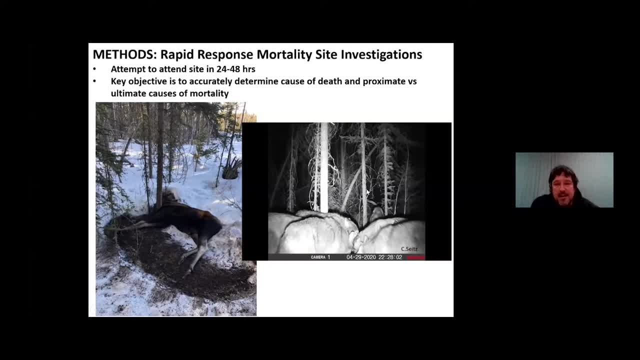 These pictures here are a good example: a moose that died from health related causes and then days later being scavenged by wolves. If you showed up later you might have missed out on the real cause of death. as an example, our other objective- that with those mortality site investigations- is to collect. 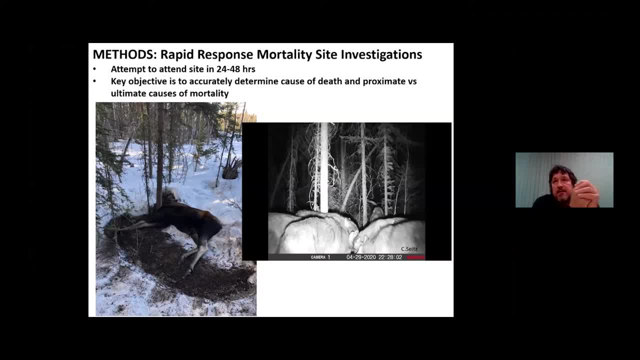 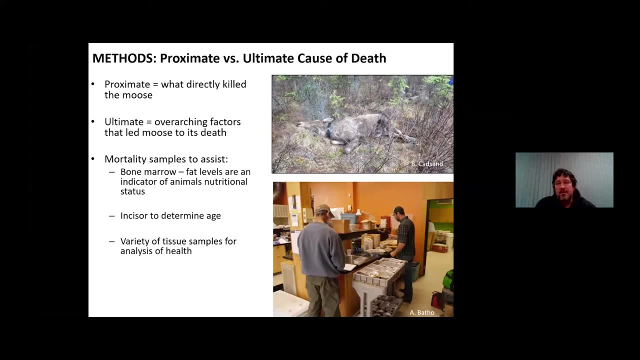 samples that would help us differentiate the proximate versus ultimate causes of death. i'm going to speak to that a bit more on the next slide here. um, so the proximate cause of death. um to evaluate the importance of various mortality factors. um we've been collecting information both on the thing that actually killed a moose- 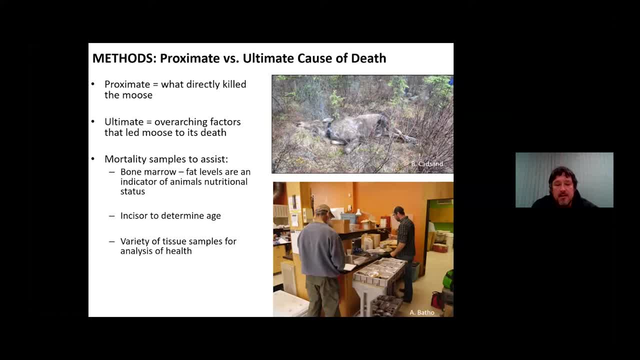 which we term as the proximate cause, or those factors that may contribute to a moose dying, though they're over the top, overarching factors that may predispose moose to to dying, and we term those the ultimate factors as another. another example: um, if predation, for example, was focused on moose that were going to. 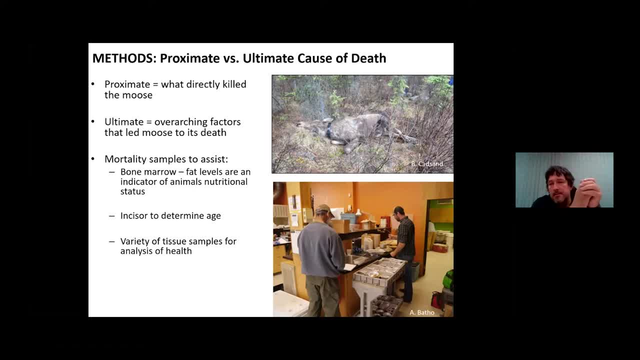 die anyway. um predation wouldn't really be the important factor. it would be the underlying causes that are predisposing moose to to predation. we collect information, um we collect information that may contribute to a moose dying at those sites on three different of those factors: um bone marrow, fat, an indicator of their 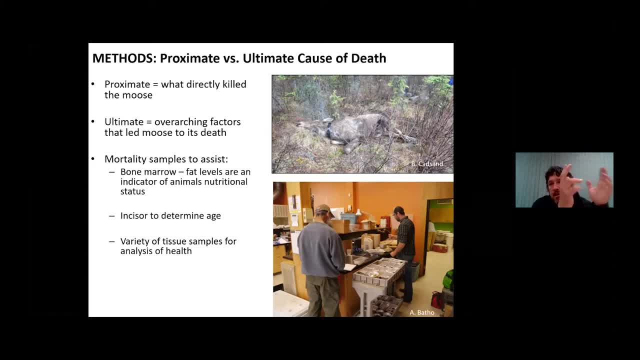 condition at time of death which we get through analyzing bone marrow fat in long bones. um, we collect those uh an incisor to determine age. obviously older moose are more prone to mortality from a range of causes. um, and then we're trying to be on site quick to really look at the 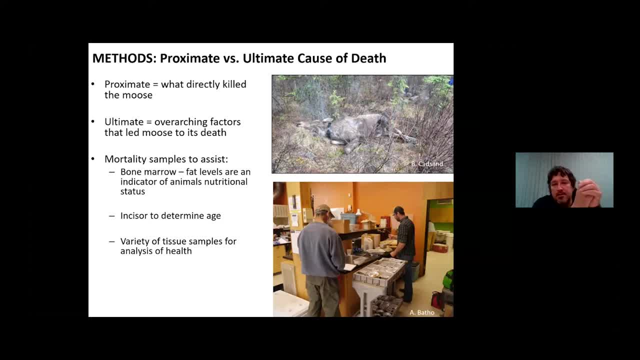 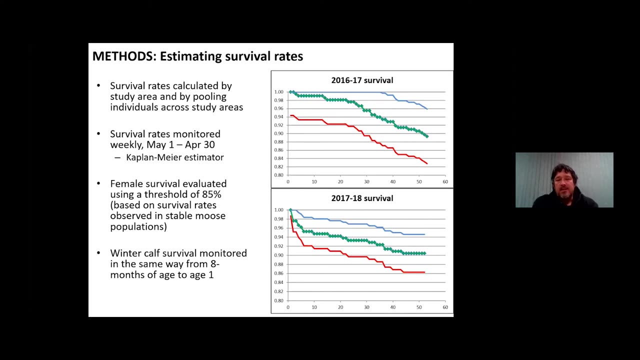 자신s um so that we go a little more down the faith. but we talked to our researchers���car um offer that recommendation. okay, we get at those tissue samples before they compost so that we can gain any information on the health of moose um that may contribute to their mortality. 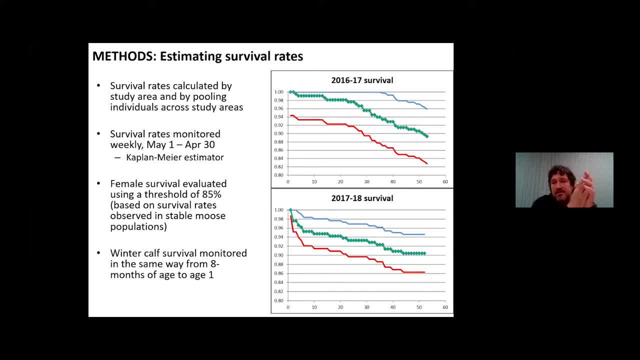 estimated survival rates. we calculated survival rates over the years on a weekly basis by study area and pulled across study areas. at the most, we have гораздо more more. So we established a threshold to help us evaluate what these survival rates mean And, at the most basic level, there are two key parameters important for population change. 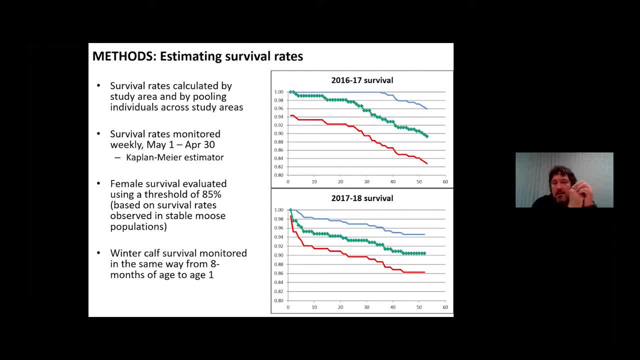 Adult female survival. calf recruitment. how those two interact defines whether populations will increase or stay stable or decrease. We established a threshold of 85% based on values in the literature from other stable moose populations, above which we assume other parameters. namely, calf recruitment would be the more important factor to focus on. 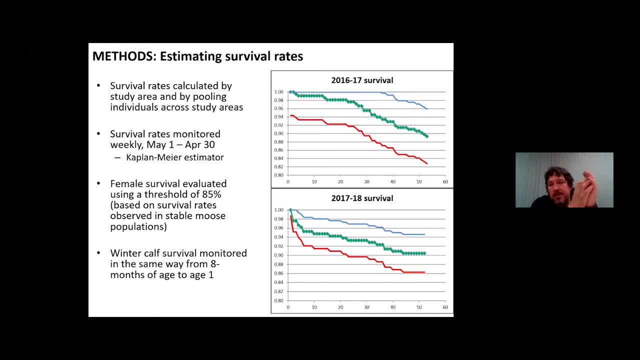 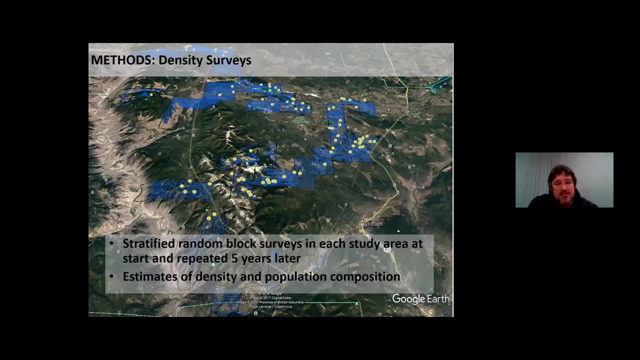 and below which we would consider adult female survival to be contributing to population change. The other piece of information we collected through this research period was estimates of moose density both at the start, when we first put collars on, and again five years later. 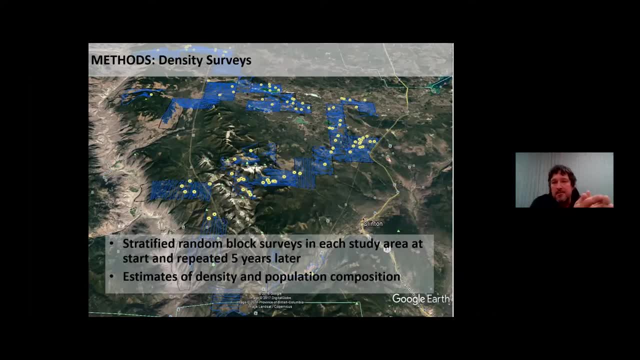 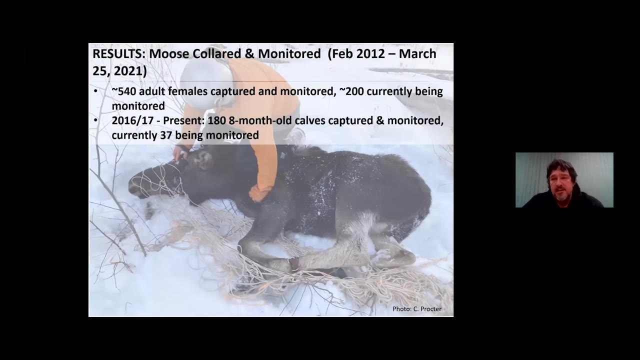 just so we had information on how these moose population changes changed as we monitored them, and it provided information to help us interpret survival rates that we measured, Thank you. So on to some results. To date, we've captured and monitored approximately 540 cow moose across these five study areas. 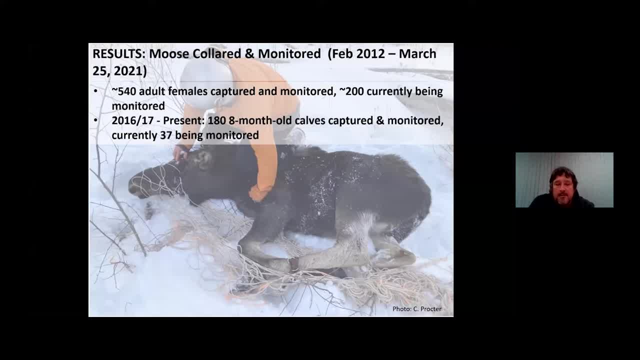 Currently there are about 200 on the air, A lot of moose. we had a bunch die, which I'm going to talk about, obviously, But we've also monitored a lot of moose through the life of the collars. 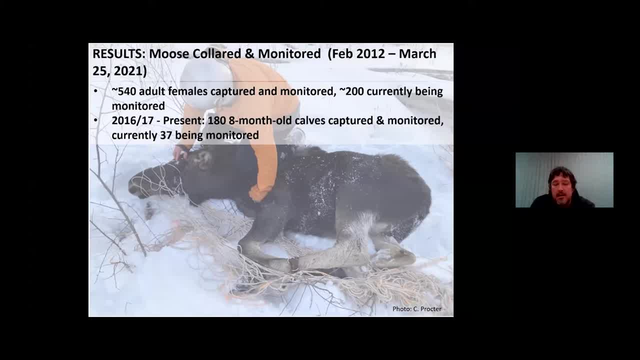 So they have failed and we are no longer monitoring those individuals, which are why those two numbers are so different. We've actually captured a lot of these females multiple times to measure how fat they are, So the actual number of captures is quite a bit higher. 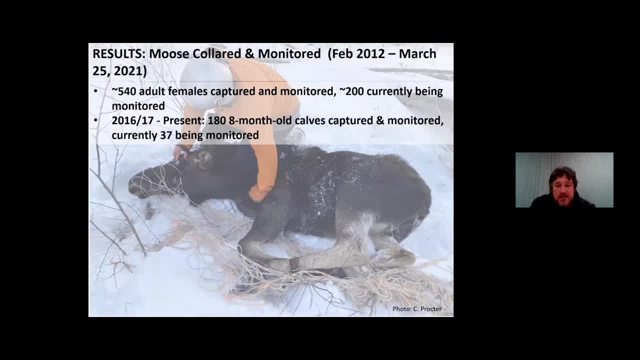 The last five years we've also been putting collars on moose calves And between in two study areas, in the Bonaparte Plateau study area and the Prince George South study area, And we have captured and monitored 180 moose calves. 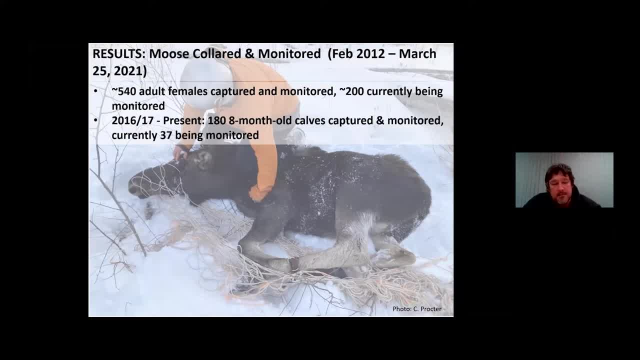 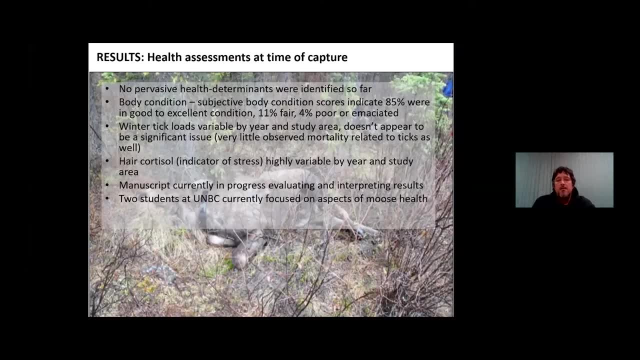 Currently. we just captured another 40 here a couple months ago and 37 of those are on the air. Some results about what we've seen from a moose health perspective, That time of capture, as you can imagine, with probably 800 moose captures through this project so far. 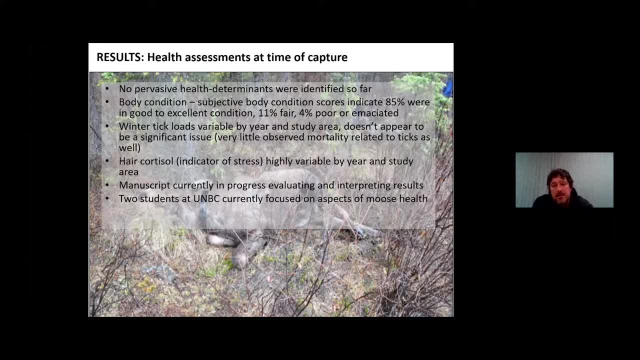 there's a ton of data to go through and interpret. It's an ongoing process. I'm not going to talk about the details much here tonight. I will say though: so far we have not identified any wide-reaching or pervasive health determinants. 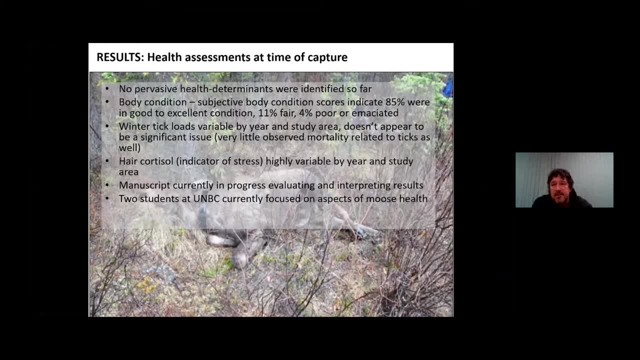 We have seen some variation between study areas. Generally, health has been a bigger thing in a couple of those study areas- Bonaparte, Plateau and Prince George South- But nothing like what we see, you know, with unhealthy moose populations elsewhere. 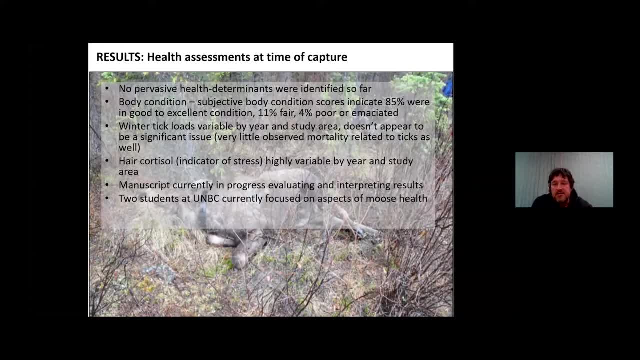 such as Minnesota in recent years. So you know it's a lot of different things. We've seen some variation, Some broad results. Most moose that we've captured were considered to be in good to excellent condition- about 85%. 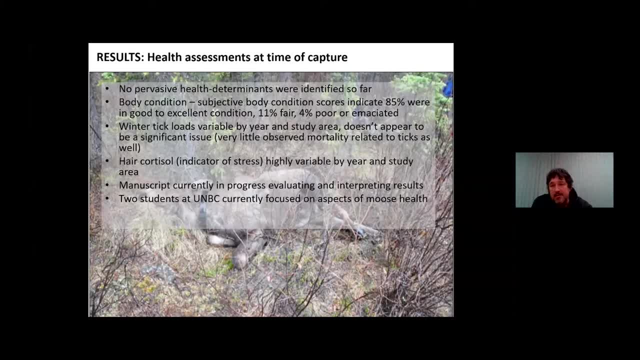 11% were classified as being in fair condition And 4% were classified as being in poor or emaciated condition. Winter tick loads, you know a big issue for moose In some places. We saw some variation by year by study area. 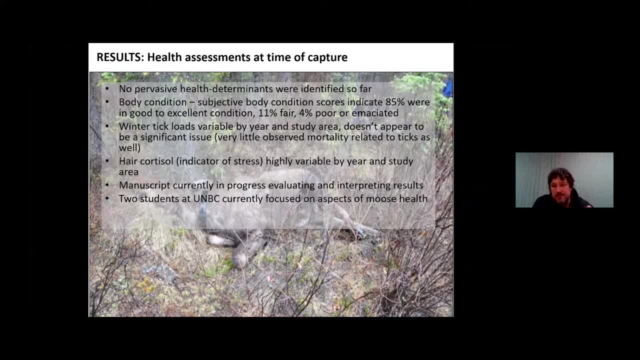 But overall we haven't seen winter tick. loading Doesn't appear to be a significant issue in these study areas. We've observed very little mortality associated with winter ticks And the overall abundance of ticks that we count on moose is relatively low compared to other places. 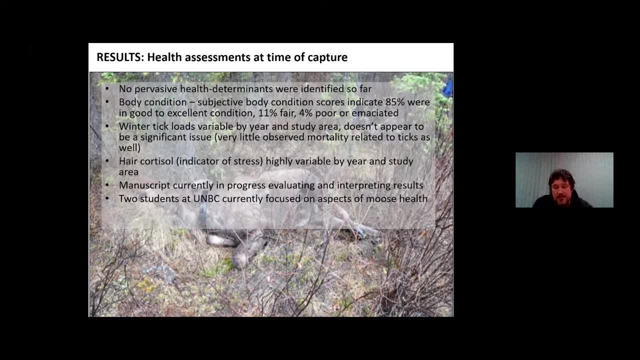 Stress levels as indicated by hair cortisol analysis again indicates that variation across years and study areas And more results to come. We currently have a manuscript being written right now summarizing and interpreting these data. We also have two new students working on aspects of moose health. 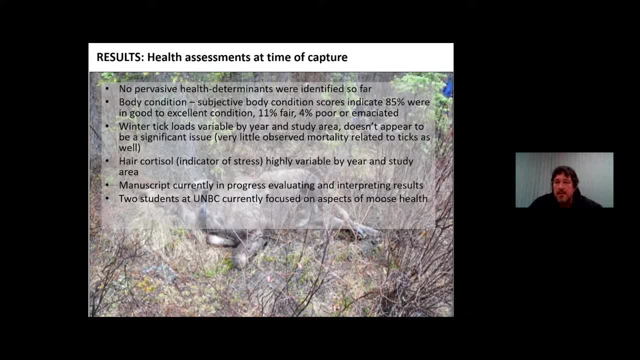 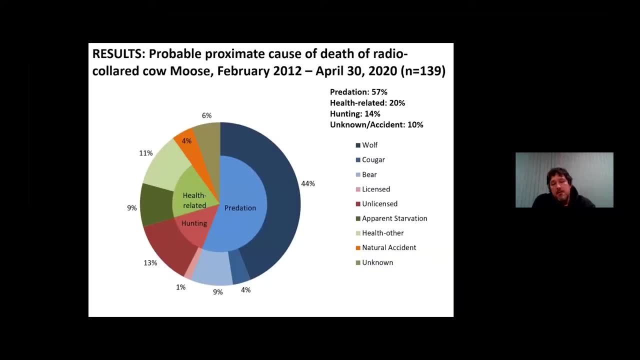 with Heather Bryan at UMBC. That work has just begun. so more to come down the road In terms of causes of mortality that we've observed over those eight years current. up until last May, we observed 139 moose mortalities. 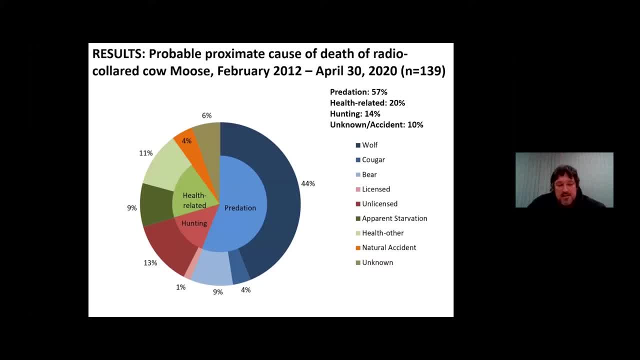 cow moose mortalities, We saw a variety of causes: 57% were due to predation, mostly wolves. 44%- 20% were health-related And approximately 50% of those we termed apparent starvation- 11%- were other health-related factors. 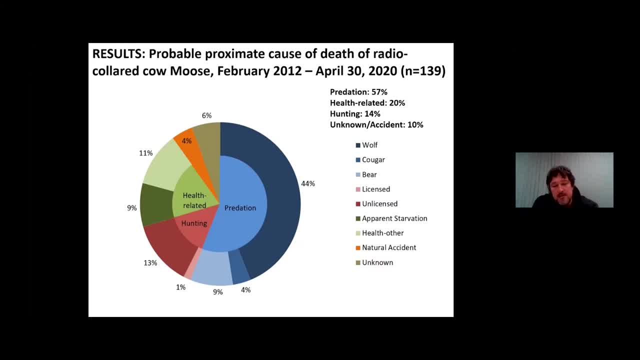 14% of those mortalities were due to hunting Broken down: 13% unlicensed, 1% licensed- 4% were due to accidents. These are moose getting stuck in the mud, hit by vehicles, that kind of stuff. 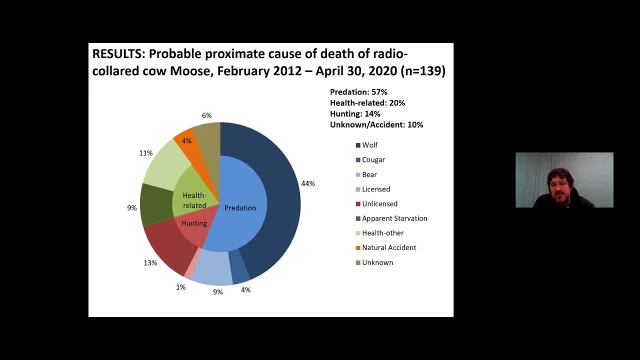 And then 6% were unknown because we couldn't attend those sites quick enough. A couple of things I want to note here. That term apparent starvation. we call it apparent starvation because the term starvation infers a lack of forage And we recognize that there could be other reasons underlying health reasons such as disease. 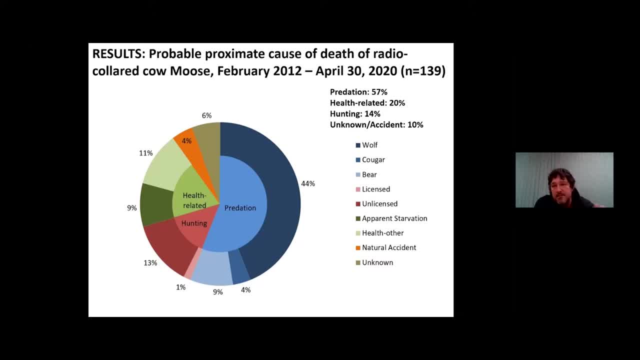 or some other related health factor that can cause moose to appear to have died of starvation. And then on the hunting side, I just want to mention that any kill outside of a legal hunting season was termed unlicensed. Often we can differentiate whether those were sustenance harvests or illegal harvests. 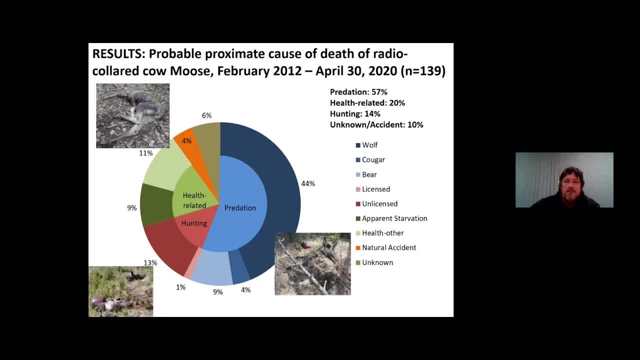 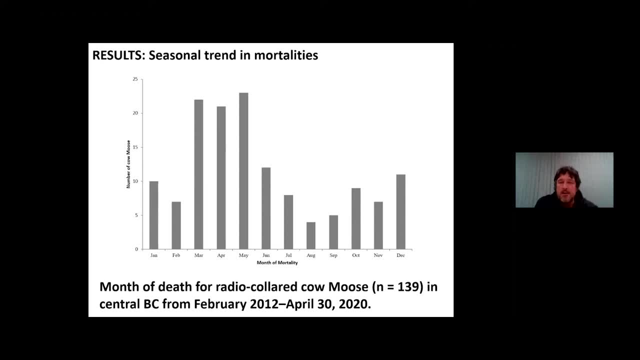 We saw a definite trend in mortalities across the year. We recorded moose dying in every month. nearly 50% of the moose that died died in that late winter, early spring period, March through May. If we look at the dominant cause of death- predation, the same trend holds true. And again you know, nearly 50% of those mortalities were March through May. There's likely a couple of reasons for that. One, snow conditions In that late winter period, when it's firmed up, often a crust, tends to favor predation. 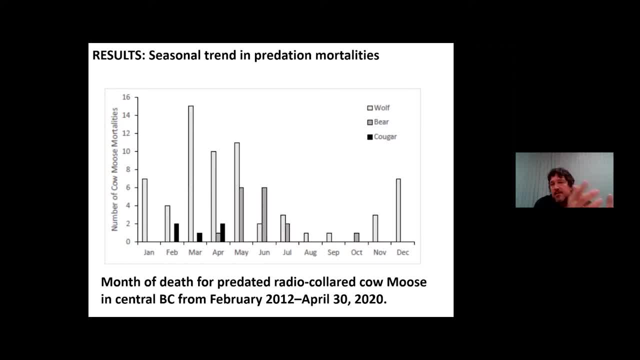 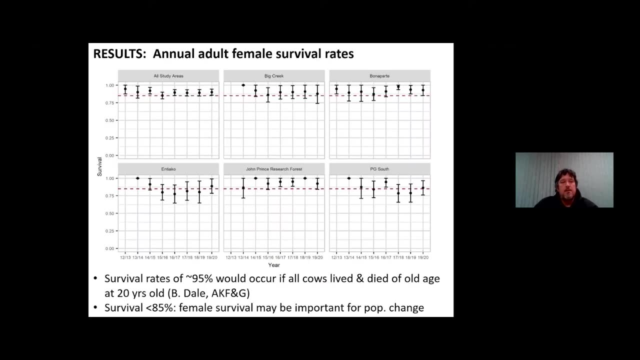 And two moose are naturally in poor condition at that time of year, You know, having gone through winter relying on their stored fat reserves, likely in a weakened state at that time. So we're going to move on to the next slide. 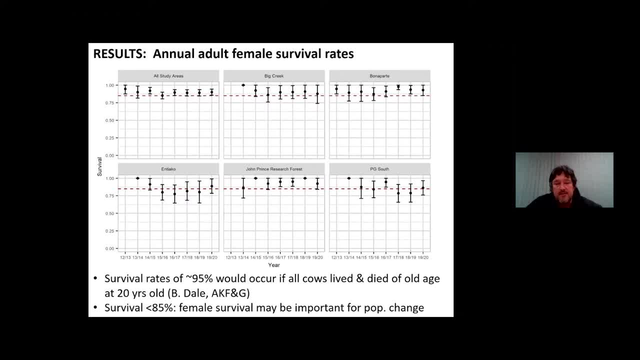 So here's the data. Here's the female survival rates, Generally higher than we expected, Not consistent with our initial predictions or assumptions. Here's the data, combined by study area on the upper left and then by individual study area on the right and lower panels. 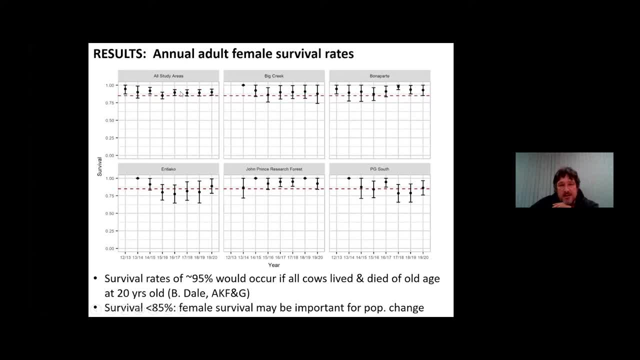 The red line on these graphs is that 85% threshold. The red line on these graphs is that 85% threshold That I talked about earlier Pooled data. In all years the estimated survival was above that threshold. When you drill down to study areas, in most of them 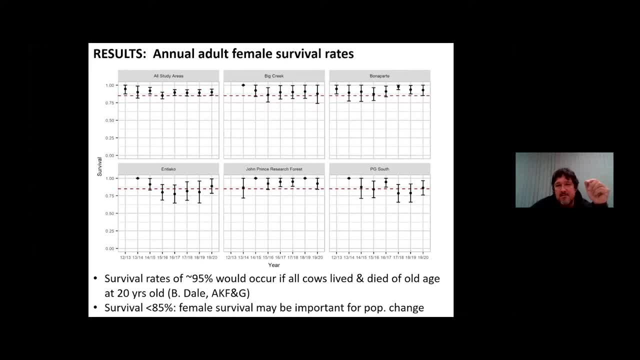 the estimate that data is a little less precise just because the sample size is smaller when you drill down to that study area level, But nonetheless those estimates in most study areas are over that threshold, which indicate that likely calf recruitment is a bigger thing to focus on. 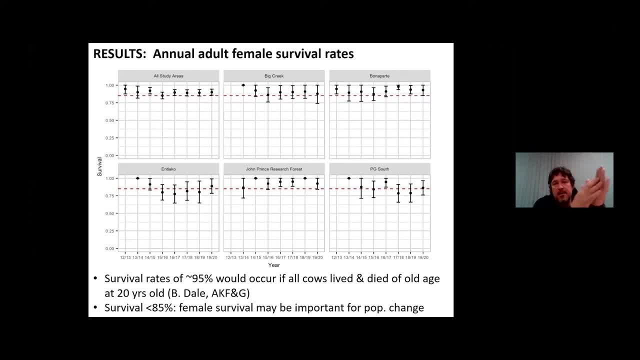 In two study areas we did see some variation. Antiaco, for a bunch of years was consistently below that threshold And PG South. we had a few estimates right near that threshold and a couple years just below. To help you interpret these numbers, rough rule of thumb at the bottom here: 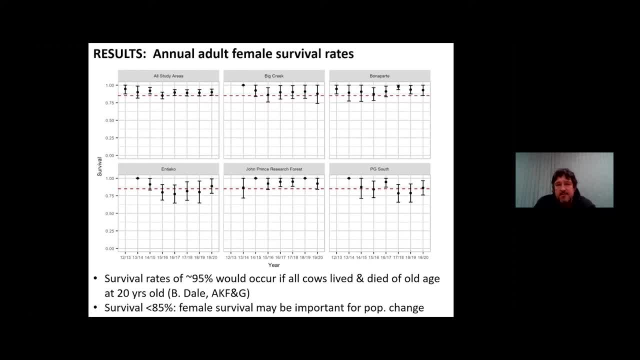 if you had a moose population of cows that all lived and died of old age at 20 years of age, the estimated survival would be about 95%. We certainly saw survival rates in some of these study areas approaching that on a pretty regular basis. 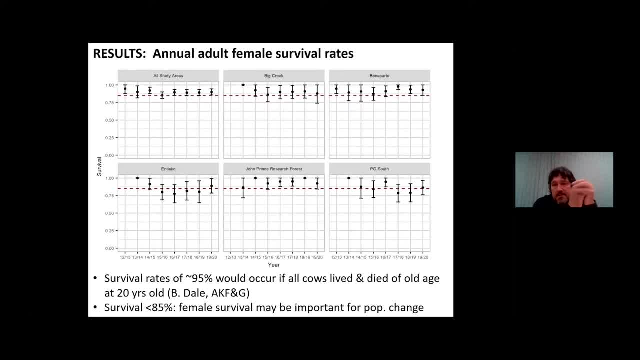 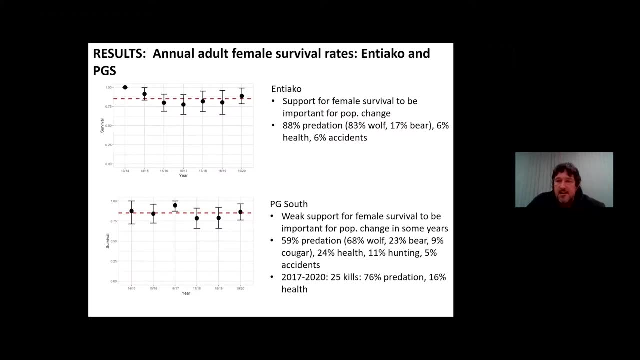 which indicates that adult female survival is highly likely. not the thing driving moose trends in those study areas. Just drill down into those two study areas I mentioned. look at the causes of mortality, Antiaco, which I mentioned. there appears to be support for female survival to be implicated in moose population change there. 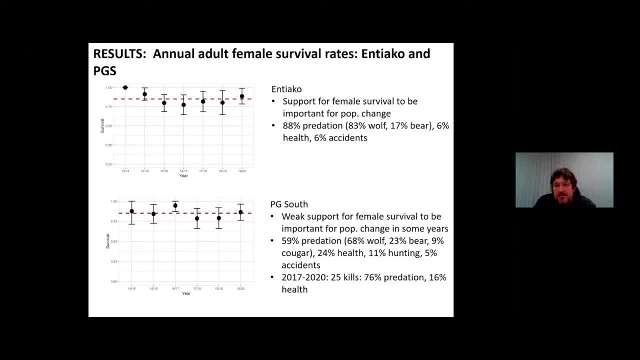 Pretty much dominated by predation: 88% of those mortalities, mostly wolves. We saw very few other moose die from other causes: 6% health, 6% accidents, Which suggests that predation is likely a factor limiting moose in that study area. 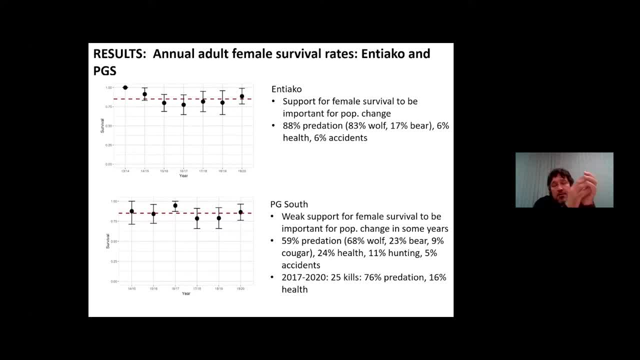 especially when you consider that most of these mortality factors are harder on juveniles than females. If you see an issue with adults it's likely higher on juveniles. So the combined effect of lower recruitment and lower adult female survival highly likely explains change in that study area. 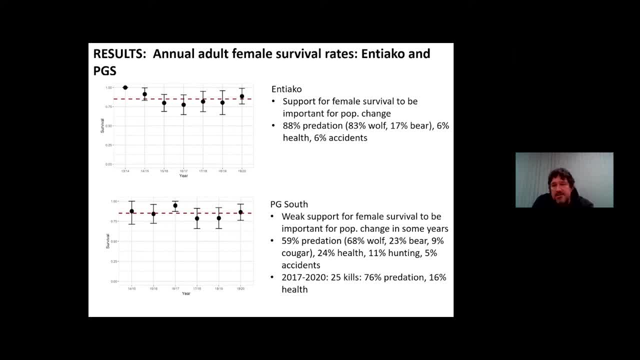 Things are a little different If you look to the next study area, PG South. you know, again we saw predation the dominant factor, but we did see the addition of other mortality factors that are important to think about, Namely those health related mortalities. So 24% of the moose that died in that study area were due to health related causes And if we drill down a little further into those years where survival was, the estimates were below that threshold. Again, it was a dominance of predation and health related causes secondary. 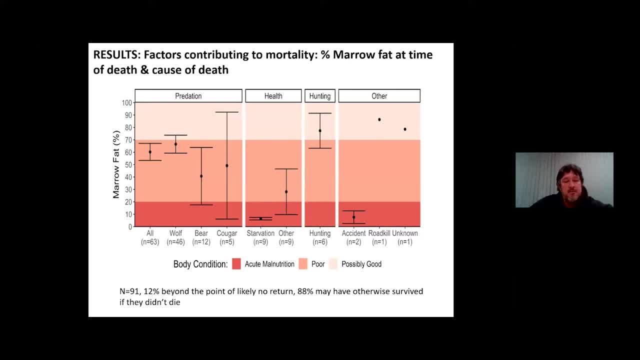 So factors contributing to mortality. These are the three factors that I mentioned earlier when we were attempting to define the ultimate causes of death. One of those was bone marrow fat. The data here is the bone marrow fat estimates by cause of death. The level of bone marrow fat is a useful indicator of a moose's condition. 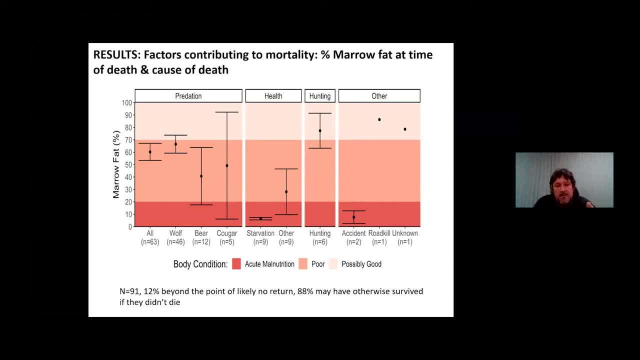 or any other ungulate for that matter, at time of death. A couple of things to keep in mind when looking at that data. It is the last reserve used when an animal is using its stored fat reserves. Therefore, it does a reasonable job of indicating an animal in poor condition. 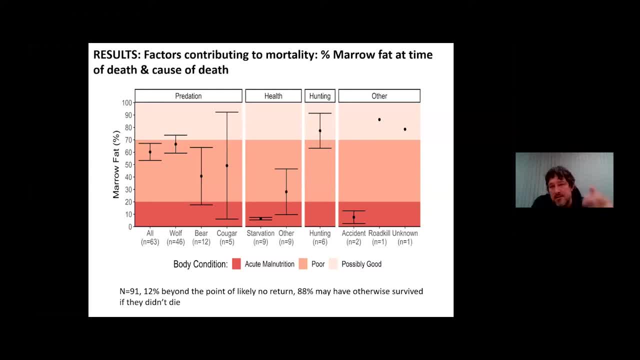 but it may not indicate reliably an animal in good condition, because you can have the situation where a moose has depleted all of its body fat but it still has high levels of bone marrow fat. And if we saw a moose, for example, that had depleted all of its body fat. in the fall when we expect them to be the fattest, that's obviously a problem. So the other thing to keep in mind: the natural cycle of body fat on moose, most other ungulates. they're generally in peak condition in the fall, early winter period. They rely on those fats to survive. So they're naturally in lower body condition late winter, early spring, before the green up occurs and they can recover that lost fat. We defined it. 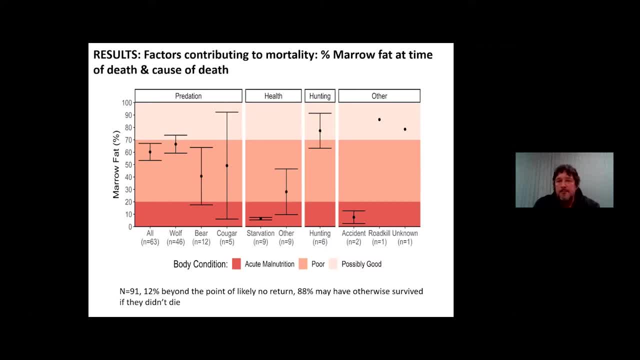 I'm going to show you guys a graph of these data by month next. Overall, we've classified these moose into three different categories, Based on the level of bone fat- bone marrow fat- we saw. we consider a moose with less than 20% bone marrow fat to be on the point of no return. 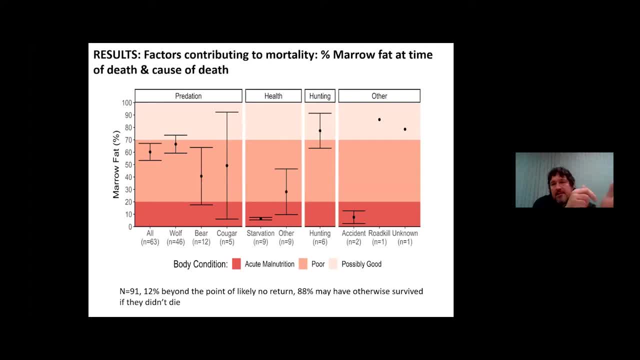 Regardless of how those animals died. if they had less than 20% bone marrow fat, that is likely the thing that caused them to die. Between 20 and 70%, we classified those moose in poor condition And beyond 70%. 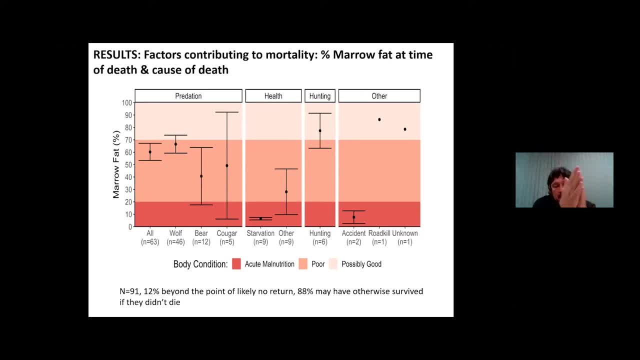 moose in better condition or possibly good condition. The moose that we saw dying in very poor condition or below that 20% threshold were generally related to health. All of the starvation mortalities were classified as moose in that condition. Some of the other health-related mortality were of moose in that condition. Accidents. so a couple of those moose that got stuck in mud holes were in very poor condition, probably played a role in their inability to get out of that situation, And then a few of the predation kills, namely by bears and cougars. 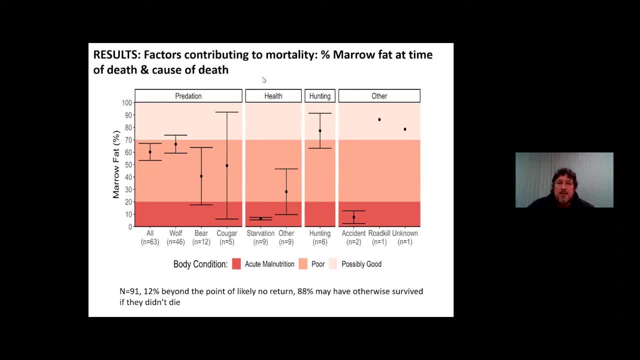 were of moose in very poor condition, Um. in contrast, if you look at the condition of moose that were killed by hunters, um, they tended to be moose that were in better condition, likely reflecting the time of year that those moose were died. 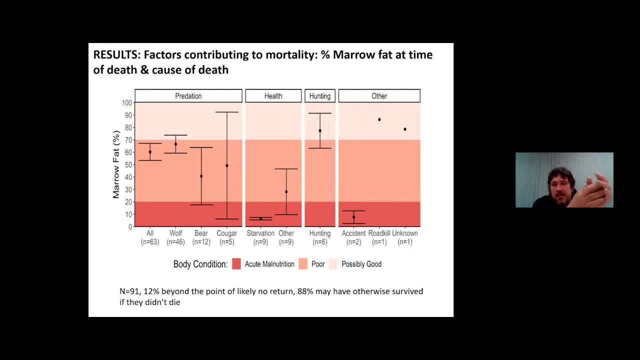 as most moose hunting, mortality occurs in the fall or early winter. Overall, these data suggest that um about 12% of the 91 moose that we've assessed um were probably beyond the point of no return, And 88% of these individuals. 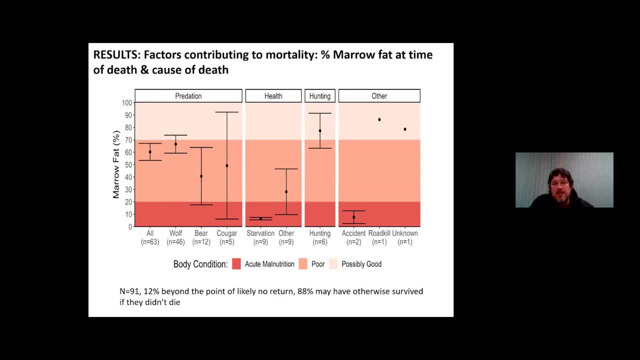 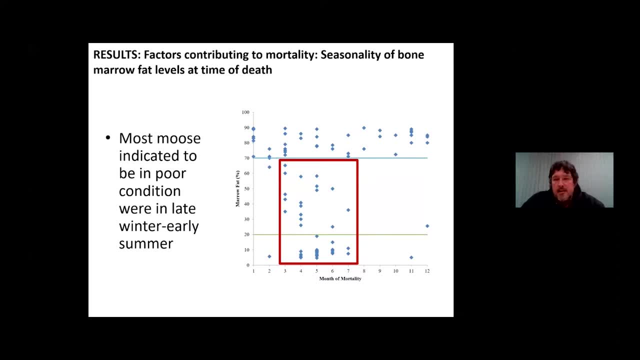 likely would have survived, um had they not died. So the seasonality that I that I just spoke about here is a graph of that information. Um, and as you can see in this um, late winter, early spring to very early summer period is when we saw. 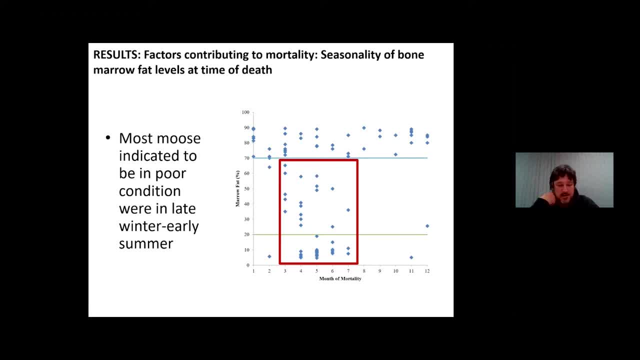 most of those moose that were in poor condition die. Um, interestingly, a bunch of moose at that time of the year are in better condition And, um, that's something that we may look at in the future, trying to understand what those moose do differently than these other moose. 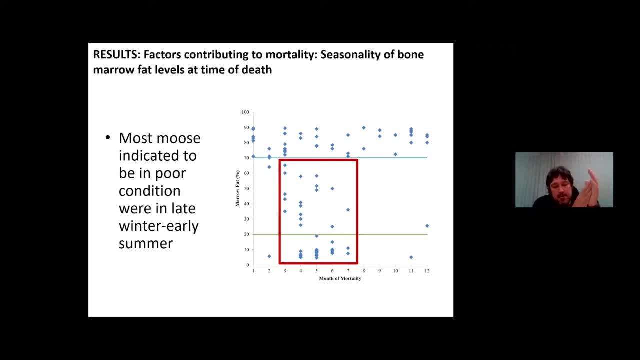 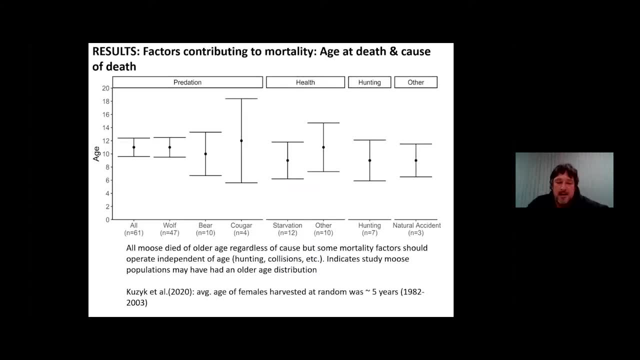 that led to that condition. Okay, Um, age age is another factor um look to to evaluate. um, obviously a moose, uh, an old moose, is more prone to dying from a range of different causes. Um, 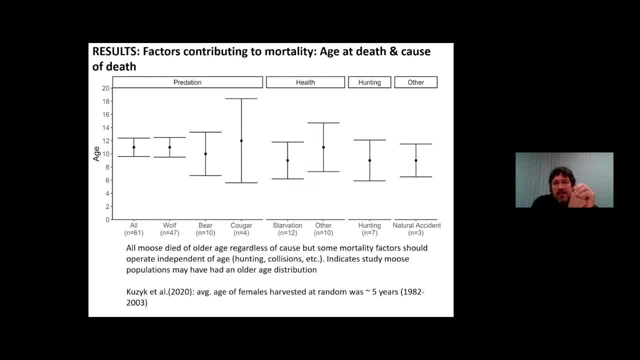 from those incisors that we collected at mortality sites um we've aged, I think, about almost nearly a hundred of those moose Um and, as you can see here, um the age at which they died tended to be older and did not change by cause of. 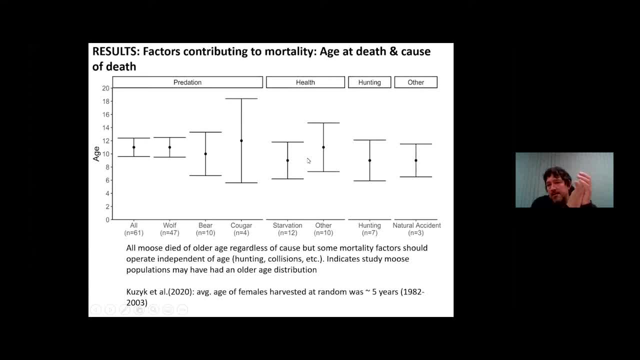 death, which is not what you'd expect. Um, you would expect some of those mortality factors to operate independent of age or randomly on the landscape- hunting, for example, or other things like vehicle collisions. We tend to have- we tend to have fewer data from hunter kills. 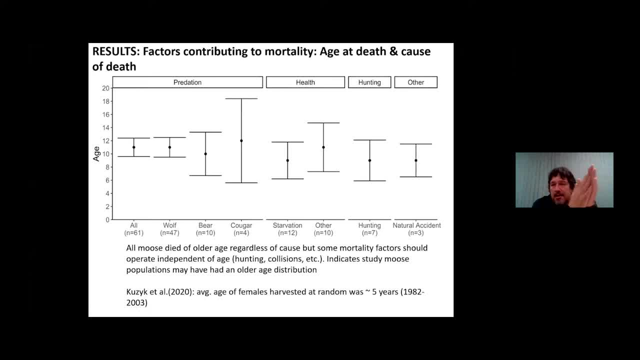 um, just because those heads or teeth are not left at sites in lots of cases, Um, but yeah, we uh a little bit different than what we expected, um, and likely indicates that we simply monitored older moose. Um. 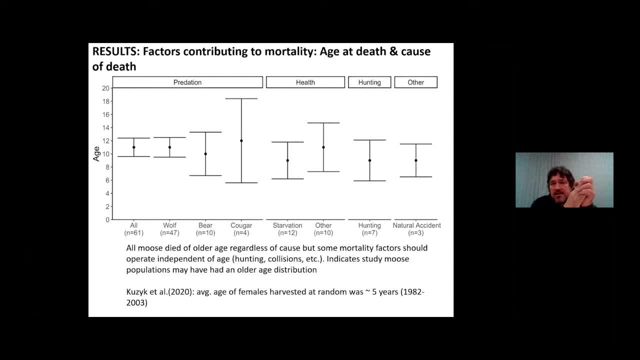 we did another analysis last year comparing these ages to ages that we estimated at harvest from the old tooth for truth program that lots of you are probably familiar with, um through the eighties up until the early two thousands, And at that time we estimated the average age of females in these study. 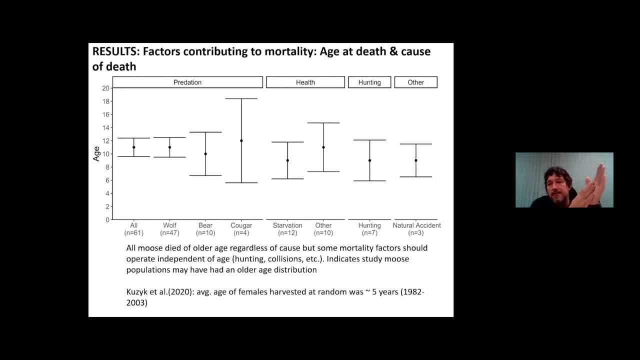 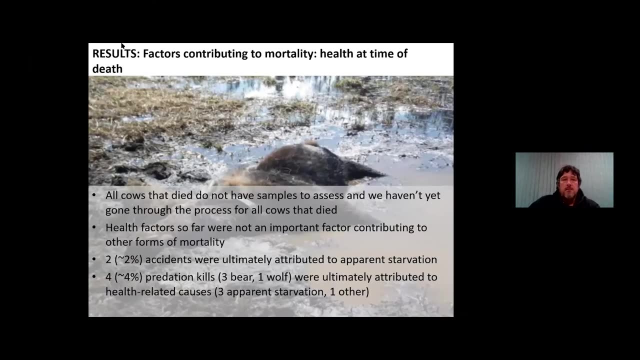 areas or areas overlapping these study areas to be about five Um, so quite different than what appears to be the eight current age distribution on the landscape. Health would be the third um overarching factor that may contribute to mortality. Um, we have not yet gone through all the data for all these cows. 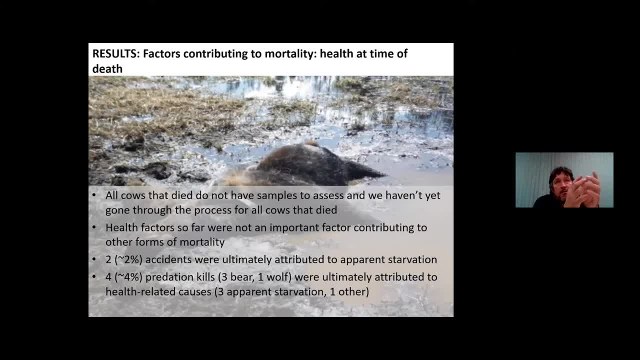 I think we've gone through the process for maybe about a hundred, maybe about a hundred of them, Um, I think there's about 40 that we haven't. we do not get this data from all females that died. Um, this is particularly true for predation kills, where all the tissue samples 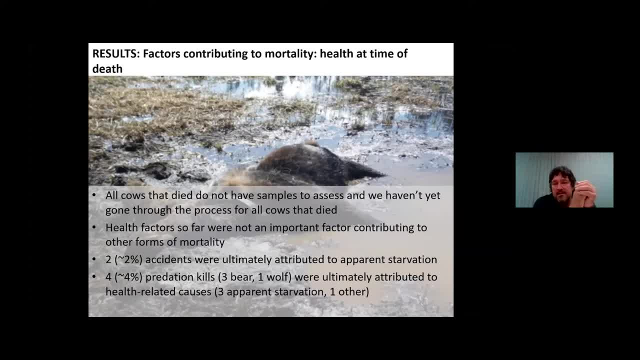 are eaten. Um, there's nothing available at the site to collect, but nonetheless we have not detected health factors to be an important factor explaining um other observed causes of mortality, with exception of a couple of cases, as I've already mentioned to. 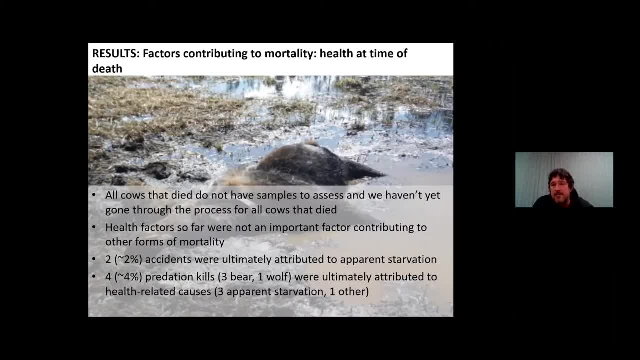 um two of those moose that died accidentally, um, we're both ultimately attributed to apparent starvation. And then a couple of the predation kills, mostly by bears, were also ultimately attributed to health related causes, And three of the four were apparent starvation. 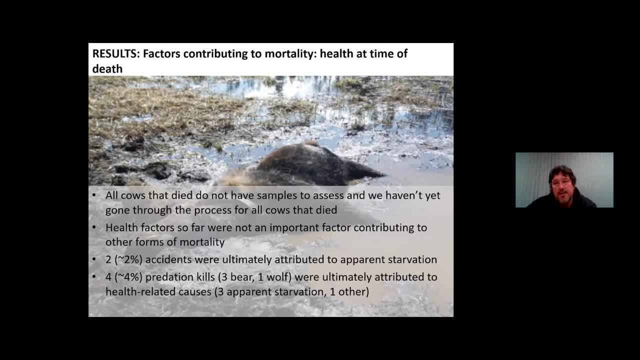 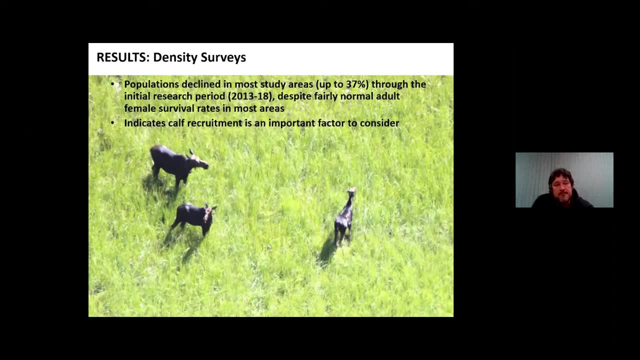 More to come on um. more to come on on this. results from density surveys: Um. moose populations continued to decline through this research period um by up to 37% in some study areas, which provides further support for that idea that 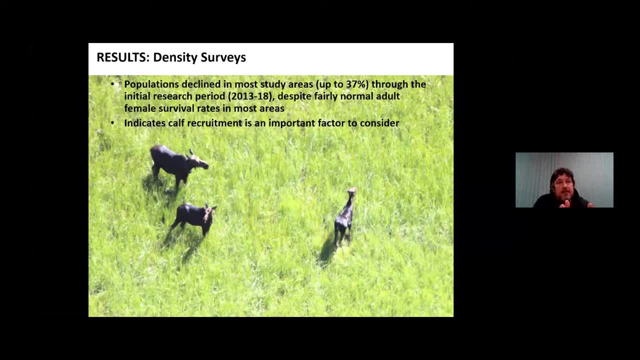 um there may be other in light of of fairly good survival rates in some of those study areas, that calf recruitment um calf survival and recruitment is probably the the most important factor explaining moose population change in most study areas. So to that end, 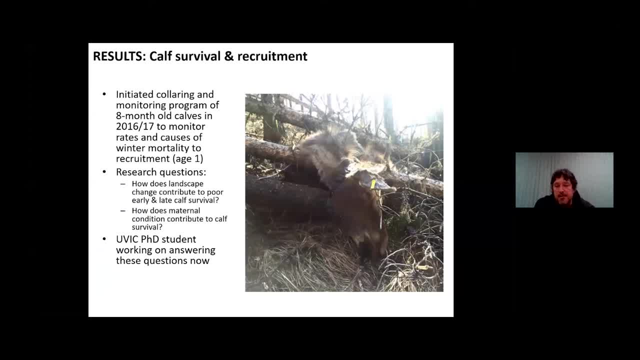 um calf survival and recruitment. we've been putting collars on cows as I read calves. As I've mentioned the last five years, we were interested in evaluating the rates and causes of mortality and causes of mortality through the winter period until those calves are considered recruited at age one or their first birthday. 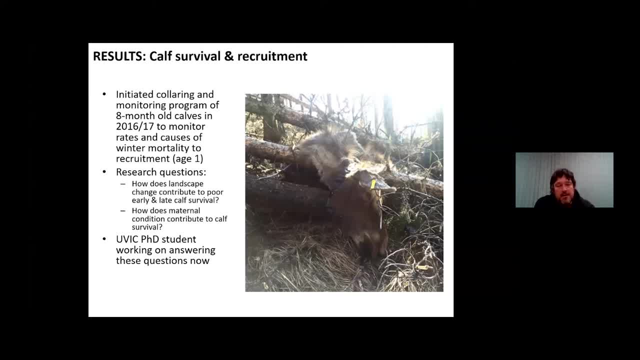 in late May Um. with this aspect of the research we were also particularly interested in understanding some of the drivers of calf survival and recruitment, namely how landscape change might contribute to that. So very similar to what we started out doing with um. 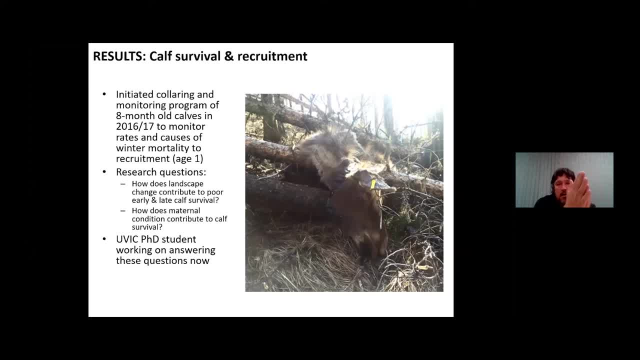 calves. Um similar questions there. Um. secondarily, we were also interested in understanding how the condition of an adult female might contribute to um their calf's survival. We have a student working on this stuff right now, um through UVic. And so more results coming here too. In terms of mortality causes for um calves, approximately 30% of those calves we've captured in midwinter died before age one. Again, predation was a dominant factor um in 79% of those mortalities, and mostly wolves. 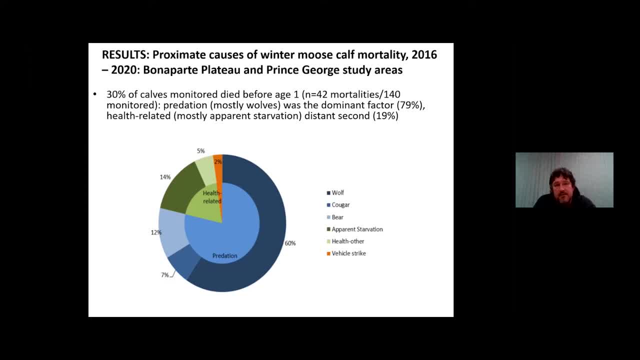 Again, although we did see higher rates of um, bear and cougar predation on calves as relative to females, And then 19% um were health related, And I believe we had one struck by a vehicle. Um, yeah, the accident there. These are the survival rates that we estimated winter survival rates. They range from 45 to 85% across years and across study areas: Um. interestingly, the um true recruitment rate at age one was consistently lower than anything any midwinter recruitment index that we would measure through a survey like a. 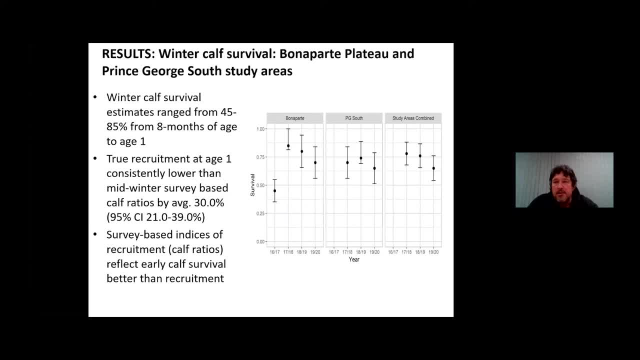 cow calf ratio: Um, the true recruitment rates were, on average, about 30% below um midwinter recruitment rates. um, which suggests: uh, it's an important number to helps us interpret, um that midwinter survey data that we do collect. 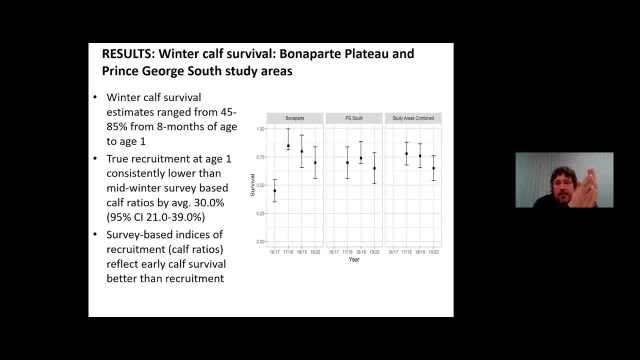 Um gives us a way to correct um those midwinter ratios. And then the other important um point here is that, given that mortality later following when we would normally measure those ratios, um those midwinter ratios are likely more reflective of early calf survival. 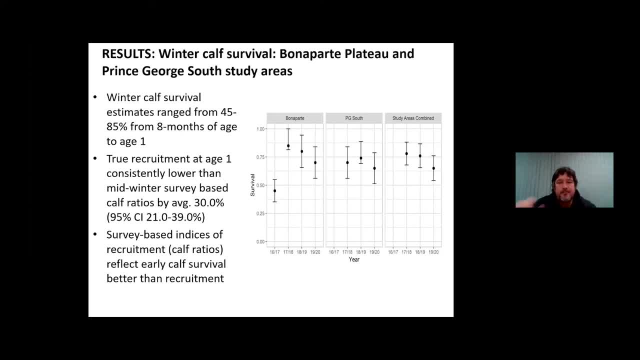 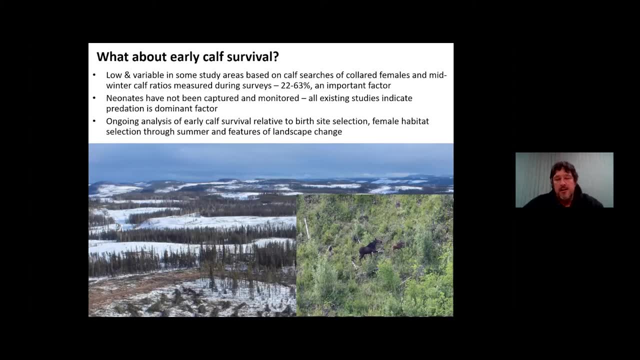 than recruitment. Um. what about early calf survival? Um, we have not yet monitored neonate moose in this research. Um certainly seems to be an important factor, um through monitoring the survival of moose calves, of these colored females. 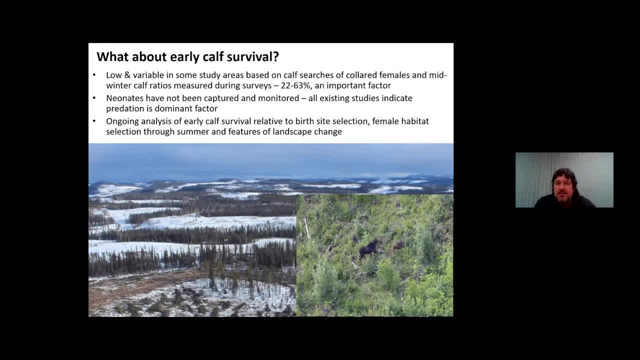 We've estimated summer um survival rates ranging from 22 to 63%. Those are uh, uh, uh. those are optimistic estimates of survival because we did not know, um how many, what the twinning rate was Um. 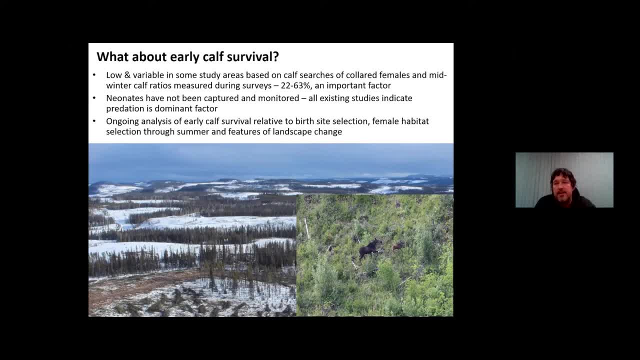 those estimates of survival assume that every female only had one calf, And we know that that's not accurate. Um we've seen evidence that in years where early calf survival is is low, combined with low late winter calf survival, um and those two combined can have a pretty significant effect on moose population. 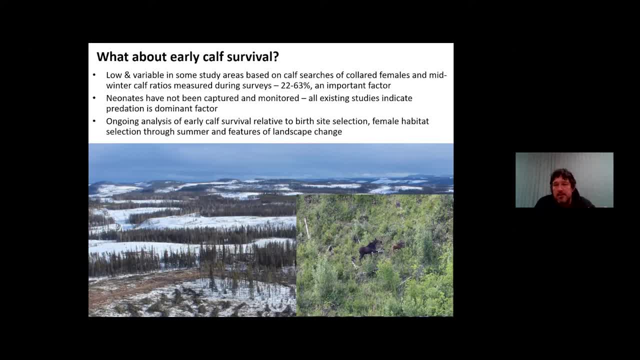 change Our approach. um, you know, we're still considering whether whether we might monitor neonates directly. Um, our approach right now is to try and get as much information on on their survival and the things that we can do to. 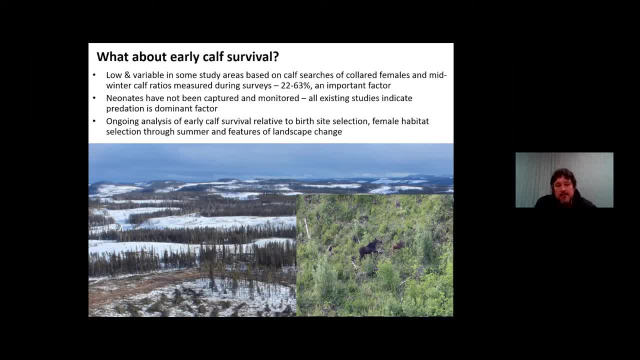 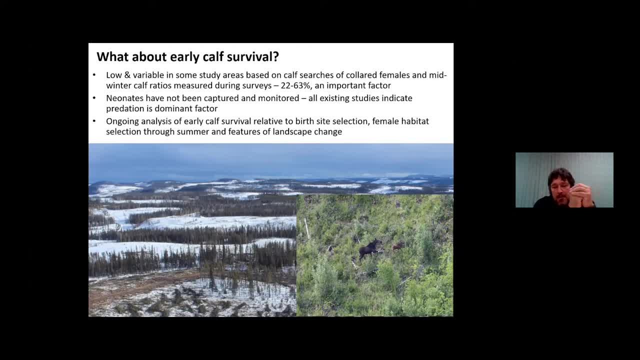 can without actually coloring them um directly. So a couple of things that are ongoing. Um, We have an analysis ongoing right now On to whether their calf is alive or dead at the end of that time period. so that's ongoing right now. 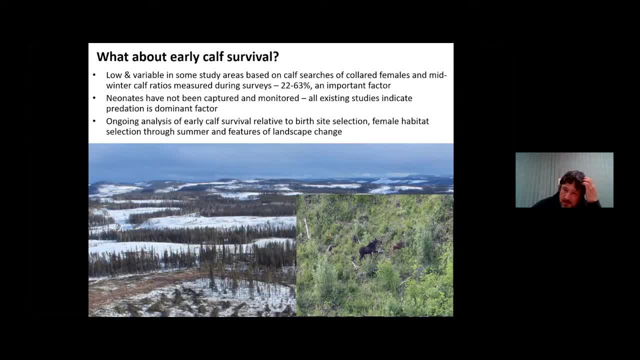 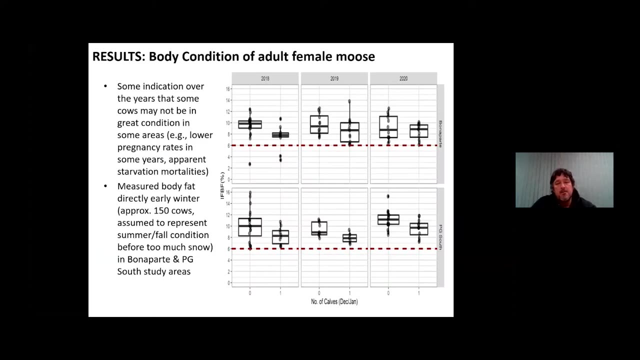 and we do have a bunch of information on moose body condition and we are looking at how that might affect early calf survival too and i'm going to show you some of that data. these are the data: body fat data for moose in the bonaparte and prince george south study areas over 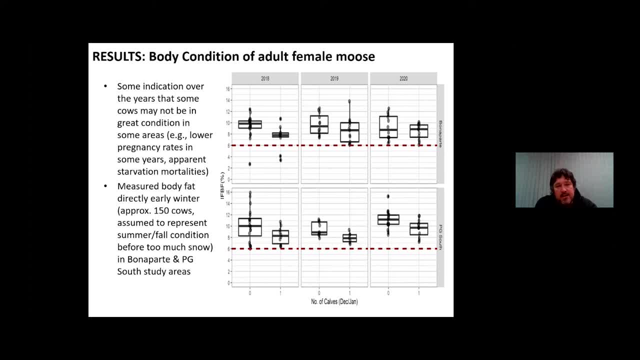 the last three years we've tried to monitor or catch these moose in the early winter period- december, early january- before they really lose body fat to deeper snow, that kind of thing- and it's been pretty consistent across years. this graph here is broken down by those cows that 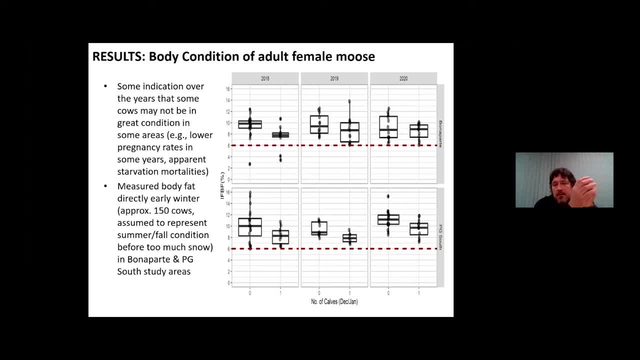 had calves and those cows that did not. obviously, a moose that lactates through the summer, they tend to be skinnier than a moose that does not, which is why we break it down that way. um, the red line that you see on that graph is a threshold. 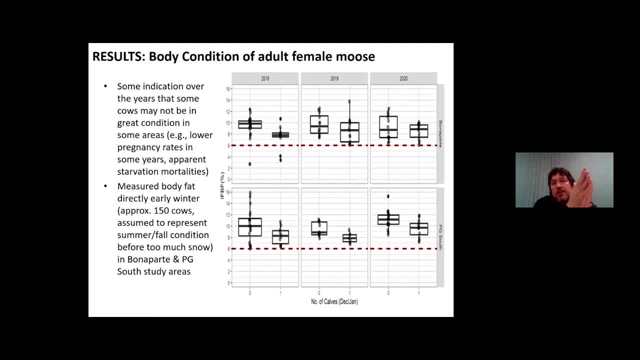 identified in the literature, beyond which pregnancy rates did not change due to changes in body fat. that is an important threshold to think about and generally, if, as body condition declines, the pregnancy rates are the first indicator of that, following that, you're going to see lower tom's out and not a single moose is actually on the landing sea near birth. 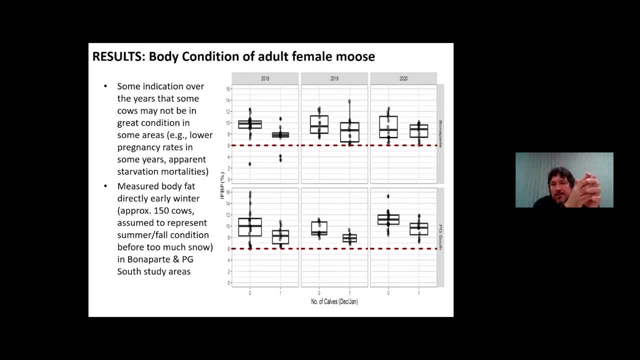 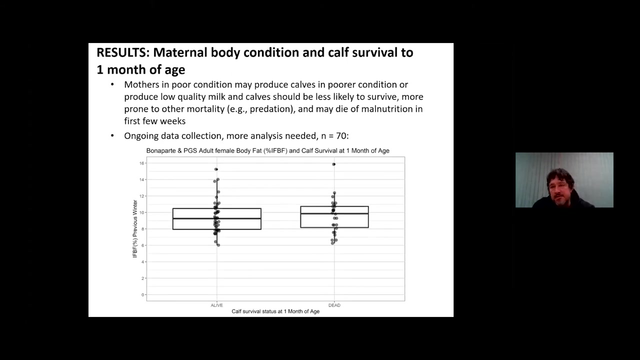 survival. and finally, the last parameter affected by condition would be adult female survival. so these these data do not indicate any glaring concerns with the condition of moose, although it seems like they could be fatter than they are if we compare that to their calves survival the following year. the idea being that mums that go into winter in poor condition produce smaller calves in poor condition, more prone to all kinds mortality predation and may even include direct mortality due to malnutrition in the first couple weeks. we've not seen great evidence of that to date. these data are still being collected. it's ongoing. this is data. 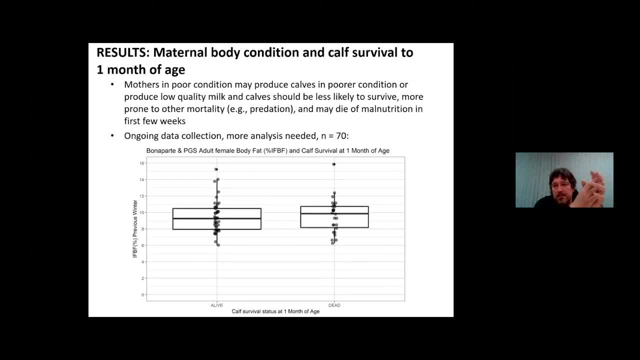 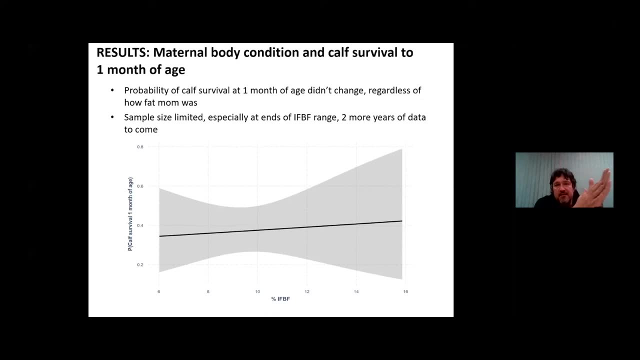 from 70 females and then they're following following summer's calf survival through the first 30 days, and they're not that different if we calculate the probability of those calves surviving as a function of how fat mum is. there really is no change over those individuals. 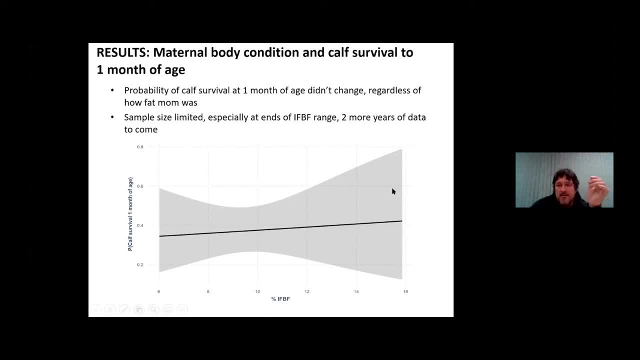 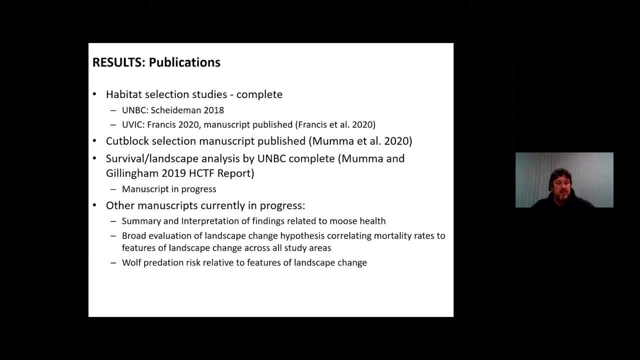 we're a bit limited by sample size, um of real fat moose, so we'll- uh. there's two more years of data coming in on this, so we will see what happens in terms of our results. we have. we have a lot still outstanding. the habitat selection studies are complete for all study areas, both by unbc and uvic. 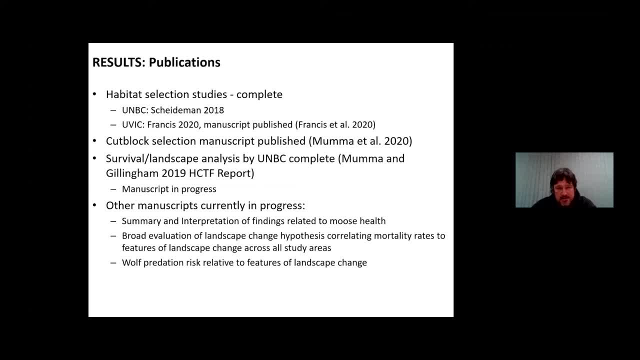 one manuscript has been published from one of those theses. we published a manuscript last late last year on cut block selection, um. the survival and landscape analyses are done and currently being written up, and we have three others that are currently being written up right now, like i already mentioned, a summary and interpretation of findings related to moose health. 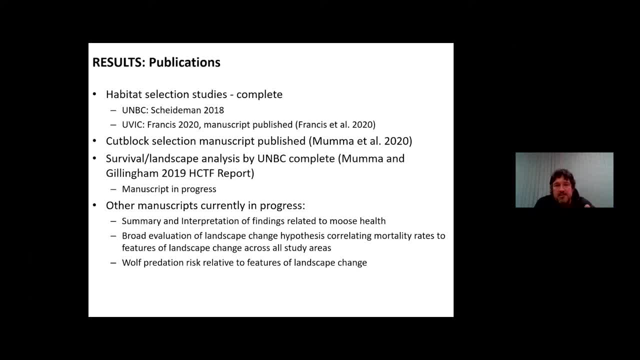 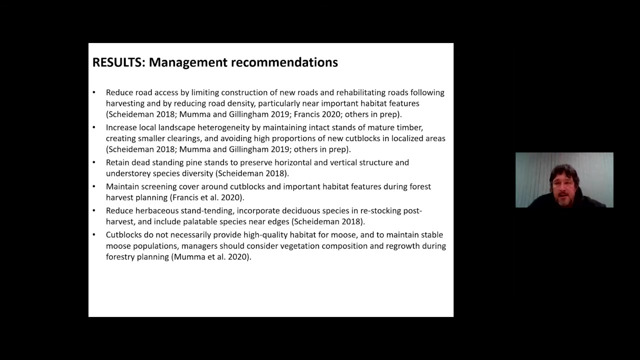 a broader evaluation of land, of the landscape change hypothesis, trying to correlate mortality rates, cause specific mortality rates, with features of landscape change across all these study areas, and then, finally, an analysis of wolf predation risk relative to these features of landscape change. these are the recommendations generated to date in those publications or theses. 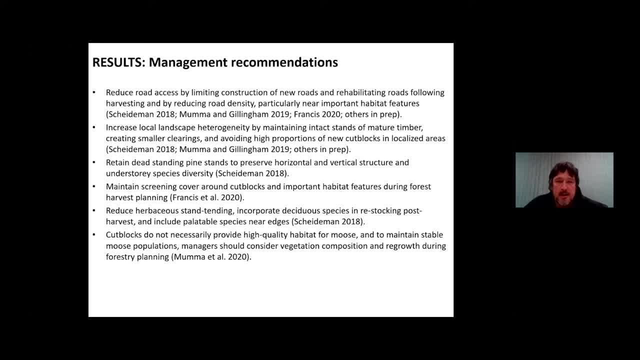 i'm just going to read them out here directly. i've kept, i've made them more concise here for this presentation. if anybody's interested in the context or additional details, let me know. i can send you the papers. um, so here we go. um reduced road access by limiting construction of new roads and rehabilitating roads following harvesting. 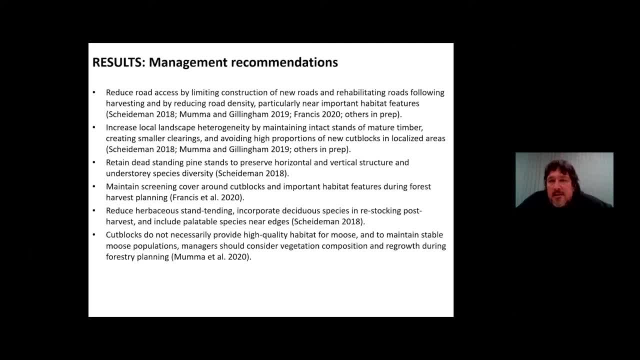 and by reducing road density, particularly near important habitat features. increase local landscape heterogeneity by maintaining intact stands of mature timber, creating smaller clearings and avoiding high proportions of new cup blocks in localized areas. retain dead standing. preserve horizontal and vertical structure and understory species diversity. maintain screening cover around cup blocks and important habitat features during forest harvest. 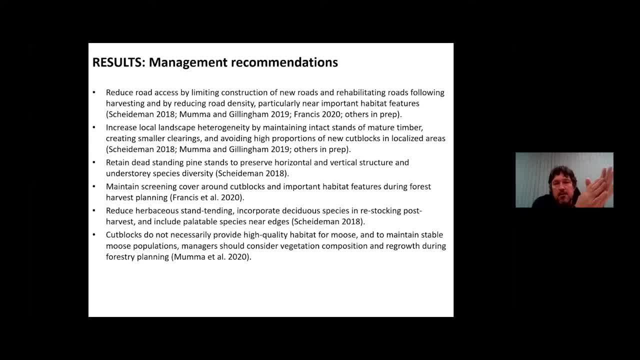 planning: reduce herbaceous stand tending, incorporate deciduous species and restocking standards post harvest and include palatable species for moose near edges. and then the next slide, please. and uh. cup blocks do not necessarily provide high quality habitat for moose, and to maintain stable moose populations, managers should consider vegetation composition. 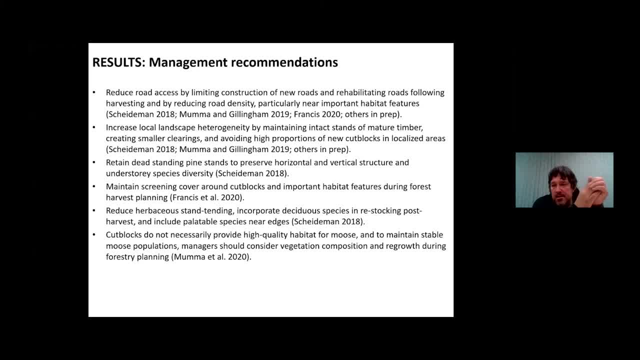 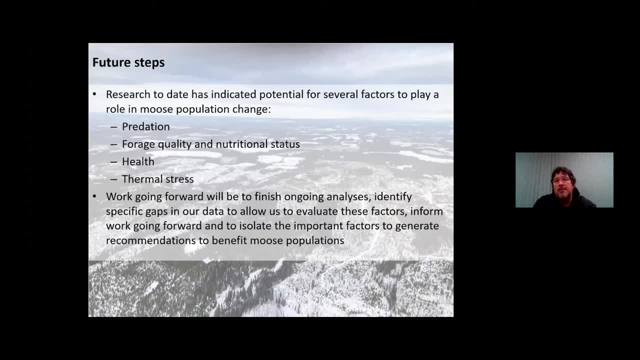 and ability to regrow during the planning stage, our future steps. um to date, we have some level of indication that several factors may play a role in moose population change and we're going to continue to work on that as we move forward with the next slide. 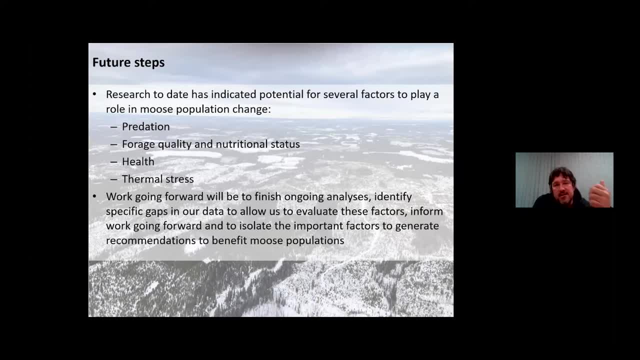 and the first step of the year is to demonstrate the import and disposal of these faeces and the use of these faeces to produce different types of faeces. firstly, if you're interested in these faeces, and пожалуйста come to moose population change. 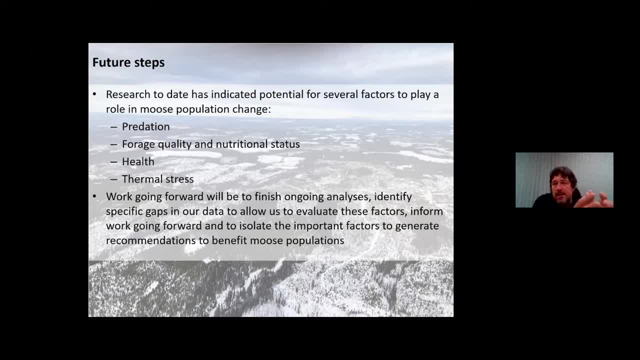 if you've not done so by the end of this year, we're going to introduce a vision for what. you know- that most of our faeces will be considered as faeces in our data, so we're going to try to evaluate these factors to the extent that they play a role in an endogenous monitoring of the. 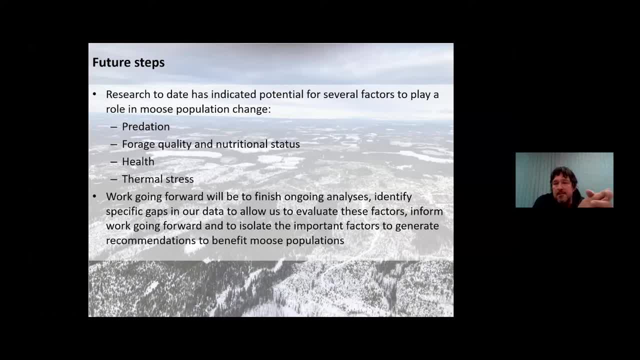 population as well as the activities of the faeces. we're going to start with the two first things is to identify the species or species that would be most important for thelamation of faeces, including soil and soil production and the education of faeces. it's important that we think about the 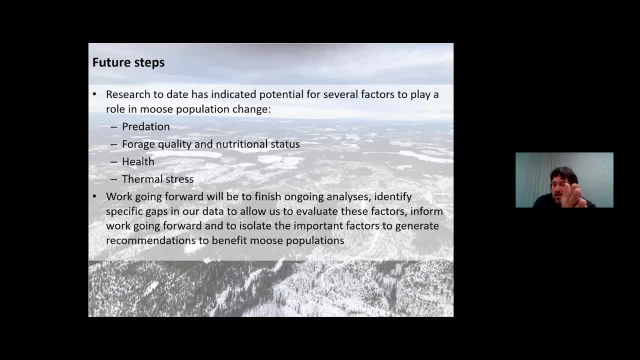 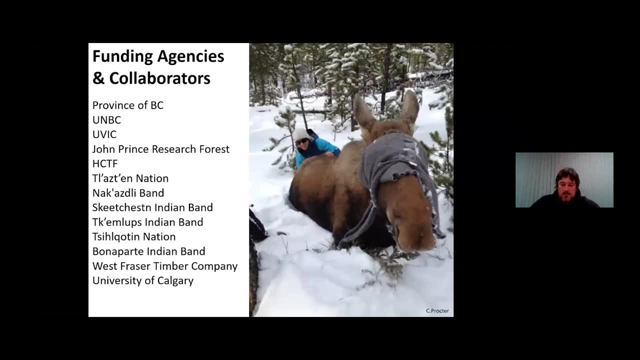 benefit moose populations in the province. That's ultimately where we are going. We've had a bunch of partners, funders, collaborators- they are all listed here and with that I will take any questions. Thanks, Chris, Awesome. appreciate the update. I've got a number of questions here. I'm going to try. 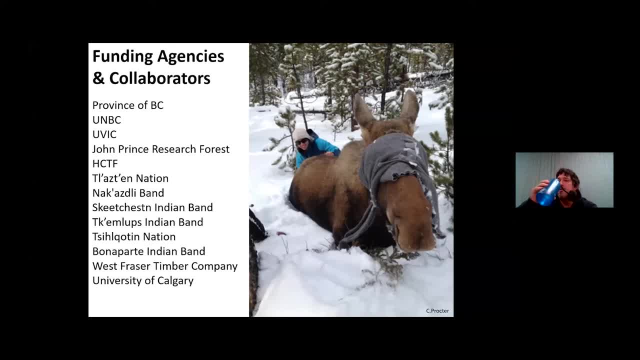 to kind of organize them a little bit around themes. There are definitely a number of questions related to health effects and parasites. Has anyone looked at differences between moose tick infestations in forested areas Versus areas that have had fire recently, or is there any literature around that? 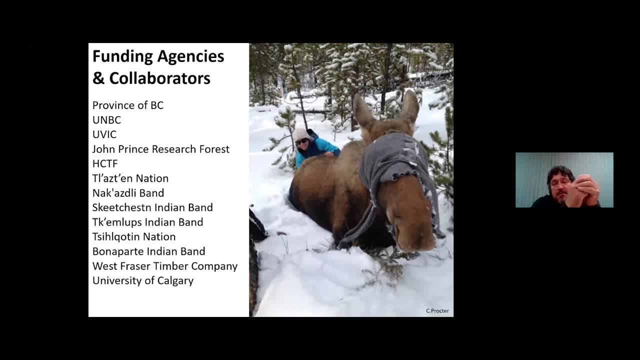 Well, there is literature out there speaking to that. I think that for a period of time following wildfire, you are going to see fewer ticks in those areas. Like I said, probably a little difficult for us to evaluate because we have not seen high tick loading on these moose, Probably the biggest. 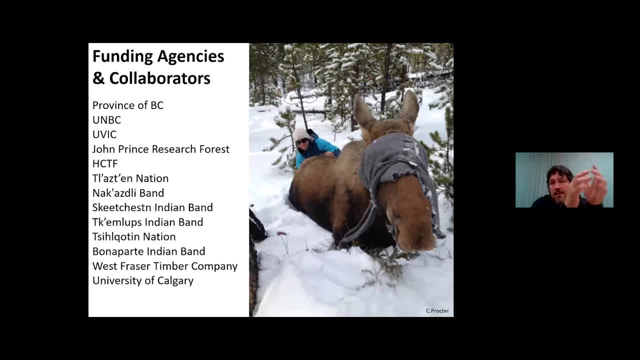 factor that we've seen that relates to the number of ticks that we've seen on moose is that early spring conditions. So a winter tick. if it falls off a moose onto snow, often it's dead. If it falls onto bare ground it's able to, you know, burrow down, lay their eggs. If you have a bunch of successive 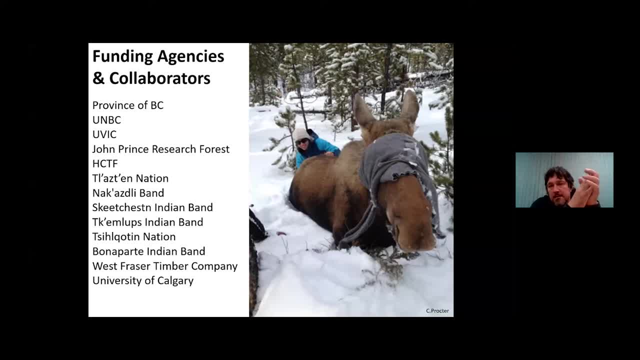 early springs it seems that we see more ticks. That hasn't been an issue a lot of the time Last couple springs. they've been later, but there was a couple springs a couple years ago where we started seeing a few more ticks, it seems following a couple of those early springs. 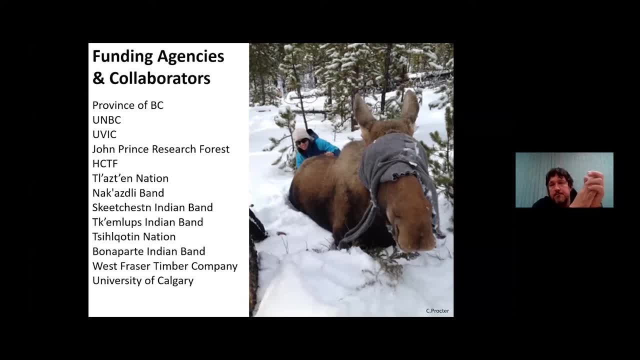 Great thanks, Chris. Got a number of questions related to glyphosate. So the effects on deciduous, Any recommendations that have come out of those papers that you talked about around suppressing deciduous, Anything broadly that you can talk about or share or discuss. 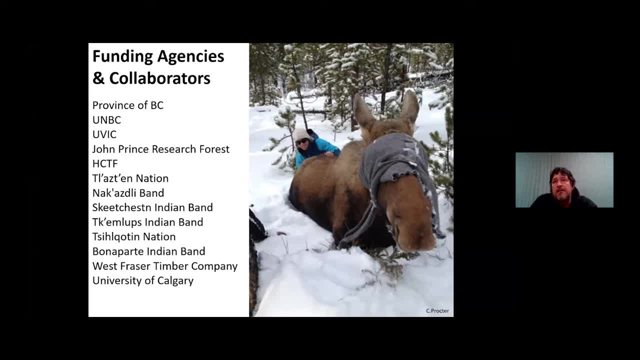 Yeah, so we have not myself, but we've had UMBC. look at this a little bit. I think it's being looked at more right now by some of our, my counterparts in Prince George. We have not found, I mean I think I can't remember the numbers off the top of my head, but 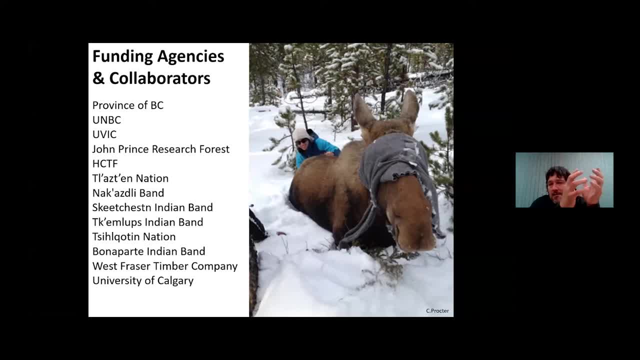 I think about five percent of the area in Prince George South has been sprayed since the late 80s or something like that. We've not seen evidence that it's at a high enough spatial extent to really affect moose numbers or their level of forage. 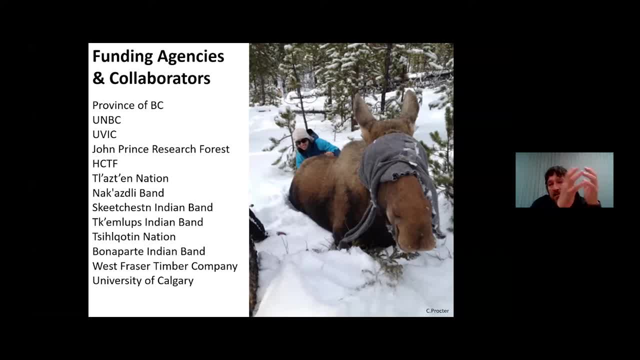 But there is more work going on in that arena, Obviously not a good thing to be doing. I mean, Hey, Yeah, Yeah, Yeah, Yeah, Yeah, Thanks, Just got a pile of questions here. Is there anything around sight distance ie cup blocks? 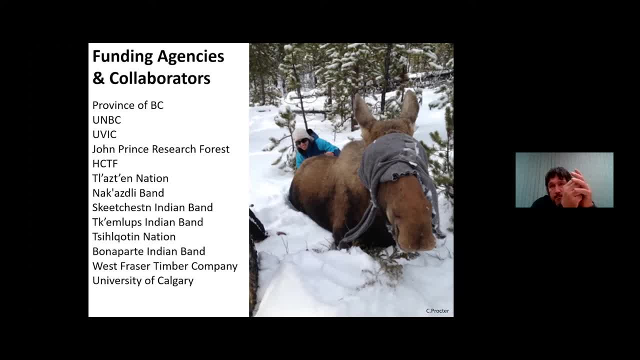 linear features, roads, increased moose predation by wolves or other species? Yeah, Certainly a relationship. that's established in the literature And we are working on that right now, So there will be some results about this coming out soon. Okay, 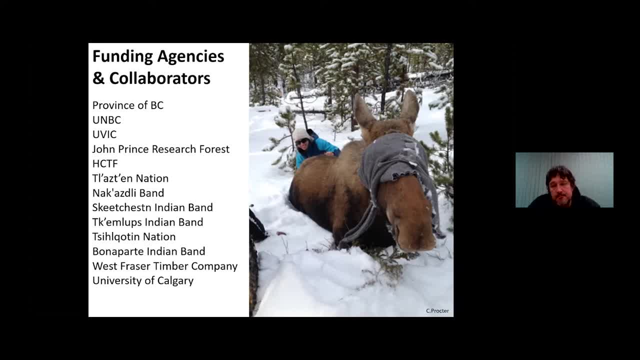 is there a chance or is there any discussion about similar work up in the piece in 7b? um, no, we did. there was some similar there was. there was a moose research project done up there for a couple years, um, and i do not have those data handy, um, but i'm sure i think there is a. 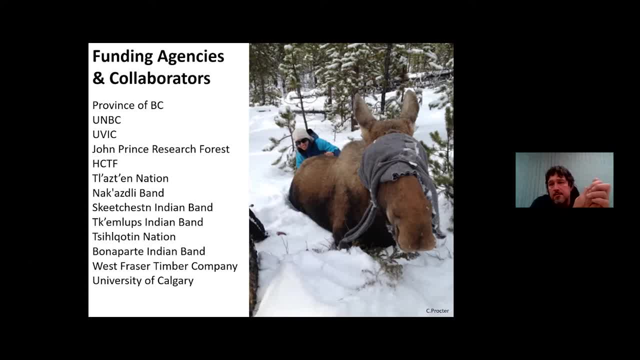 report about it online somewhere um. nothing being talked about right at the moment, though that i'm aware of. okay, thanks, uh, this is around the collaring piece. do you ever collar the same individual over multiple study years? we have um some of those um cows that we monitored earlier. 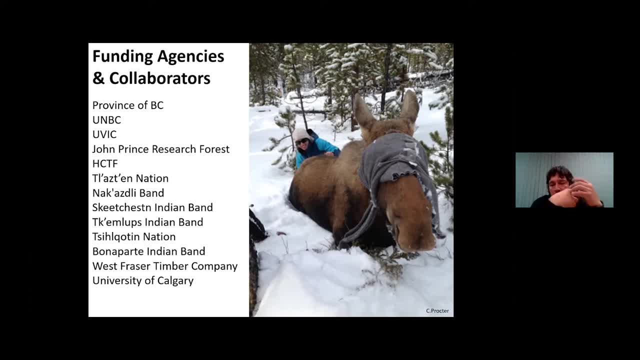 that lost their radio collars or we released those radio collars when we were finished. we have certainly caught them randomly in future. um, Yeah, it's happened a few times. okay, awesome, uh. a few more health ones, and i'll kind of put them together: anything around in the literature that you found around: tapeworms, liver flukes. 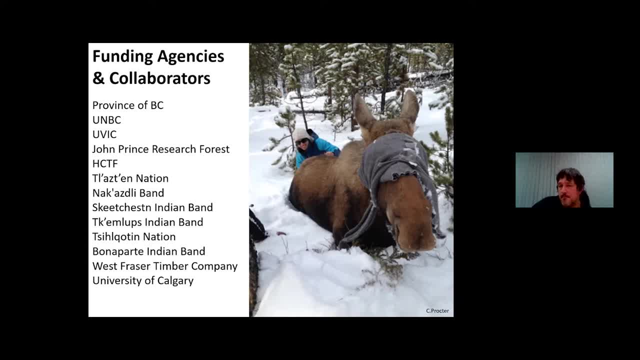 and the other one that isn't in here that i'm sure they'll get asked- is brainworm as well. um, we've not seen brainworm in british columbia. there are liver flukes in some wildlife populations in british columbia. we've not seen it in any moose. 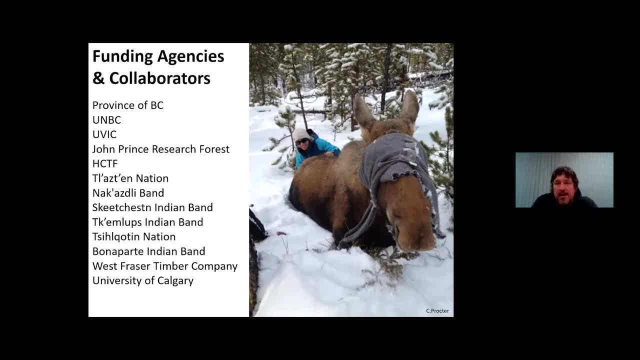 in this research, although we have seen it- and i've just recently actually, in region three, had a case of liver fluke and a moose, um, but we've not seen it with any of these study animals and tapeworms. yeah, i mean, it's a pretty common parasite for moose, so we've definitely seen that. 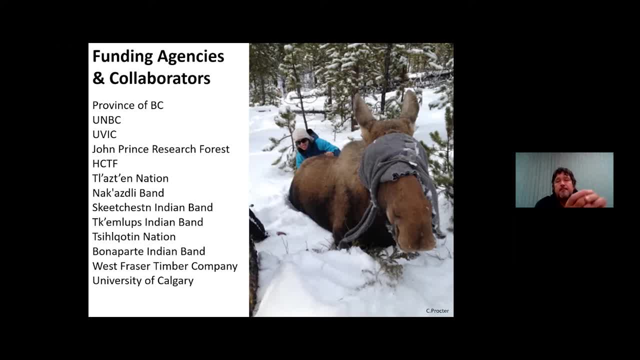 okay now i don't know if you want to venture out on this one top three factors related to declining numbers- any recommendations? I think we need to. yeah, I mean, predation is going to be up there, but I do. I do think we need to get some of these results wrapped up before we. 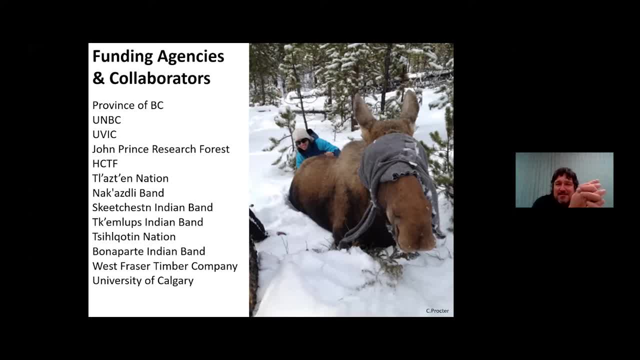 answer a question like that, Gotcha. here's one. in the second slide, side by side, aerial shots were labeled dead and alive. can you elaborate on what those photos illustrated? Yeah, good question. I don't know if I explained that well, it was just an example of what we're. 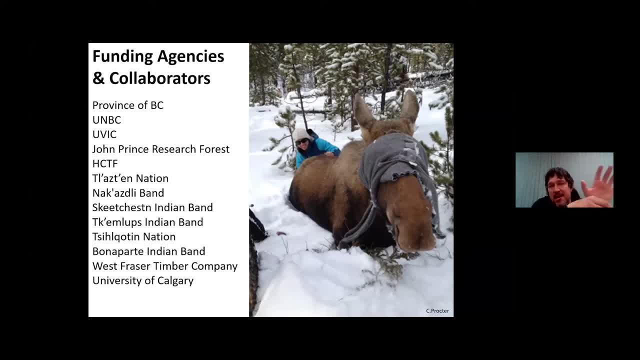 looking for with this research. so it was an example of a moose and what she did for a year and ended up dead, relative to a moose and what she did for a year and was alive, right it was just. it was just an illustration of of what we're looking for. 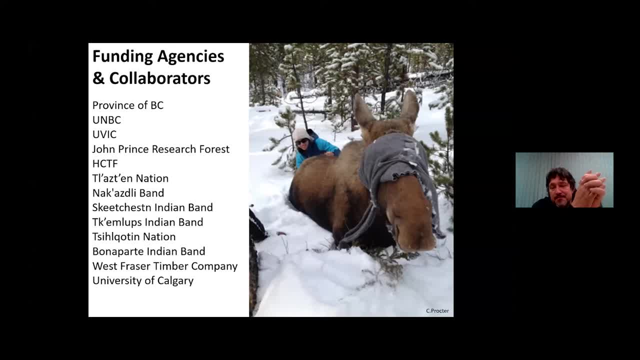 Thanks. any theories or work on why the hair, the cortisol levels vary so much? Yeah, well, they can vary with a range of conditions. environmental conditions may cause moose to be more stressed. we did see, for example, moose, even though we didn't see winter ticks to be a big. 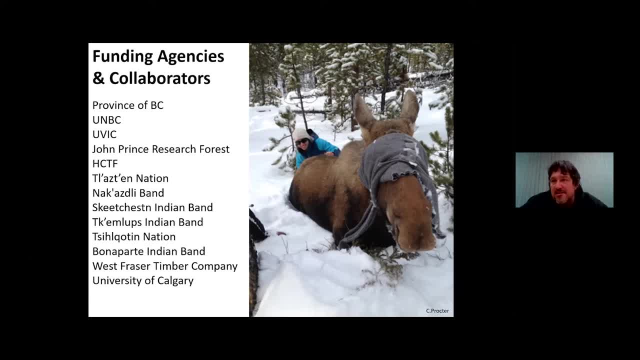 big factor here- a moose that did have more winter ticks on them than another moose, to be of higher levels of cortisol the year, the precipitation condition. there's a whole bunch of things out there that that contribute to those stress levels, and that is something that we are. 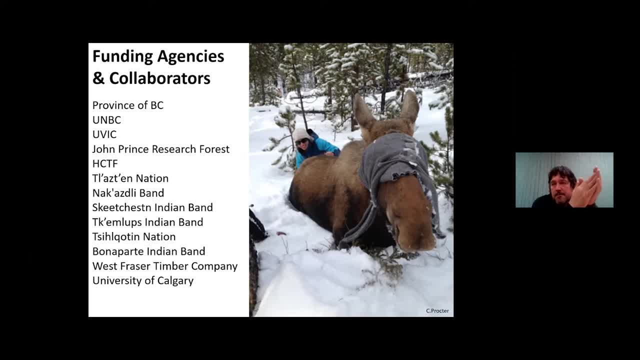 trying to interpret right now, in that people that write it, even whether a moose has a calf or not, can change their levels of stress. Okay, um, shifting a little bit to neonates and young calves, I'll lump a few questions together. uh, what's the the general thought of the literature? you covered this to a certain extent around calves. 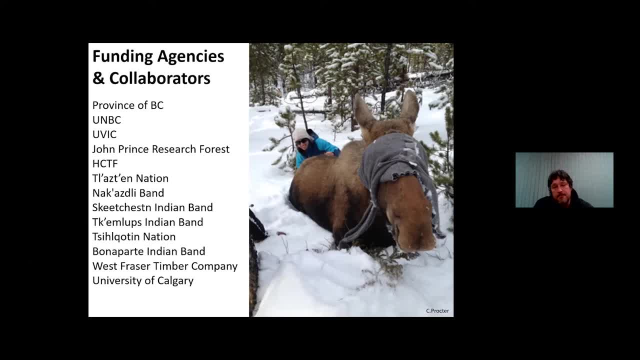 before they're eight months old. um, and then discussion around the effects of bears on calves and neonates. um, is there anything in the literature that you can that comes top of mind around dealing with neonate survival? and and bring that into the discussion? Okay, thanks. 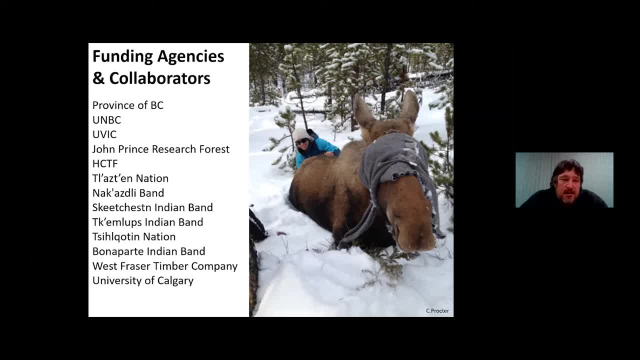 particularly bear harvest. Yeah, it's a great question. It's probably one of the reasons we've avoided doing it right now. There's been a bunch of studies looking at causes of neonate survival across North America. In every case, predation has been the dominant factor. 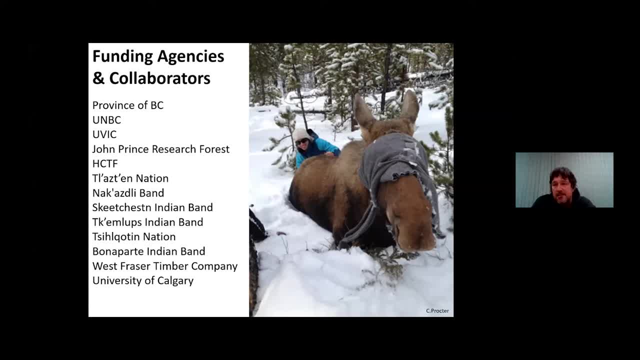 In most cases, bears are identified as the dominant factor, although in the latest one from Minnesota I believe wolves were the dominant mortality factor for neonates. But yeah, I think we struggle with that a little bit. It takes a huge effort, a bunch of money, a bunch of time. 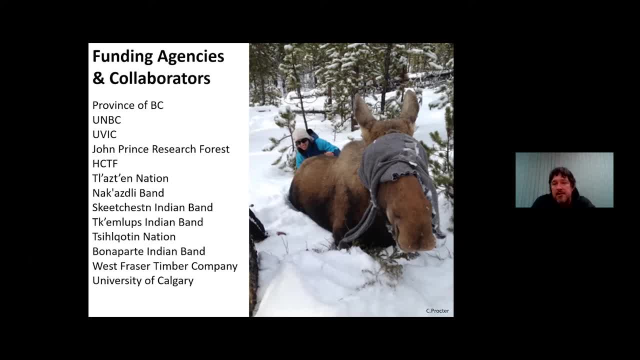 just to learn the same thing here. right, I expect that that's what we would learn. So I don't know what to tell you- whether we're gonna do it going forward or not. but yeah, those are some of the things that we're thinking about anyways. Thanks. Whether bear harvest from hunters can deal with that, that's hard to say. I mean, I think that there's probably- I don't think all bears are eating moose, calves or deer fawns for that matter. It's probably a handful of them doing a lot of it. And I don't think random hunting. you're likely not gonna kill those individuals that are responsible for it, but you might if you get lucky. There's probably a relationship with overall bear harvest rates and neonate predation rates. Thanks, Now do you have data? 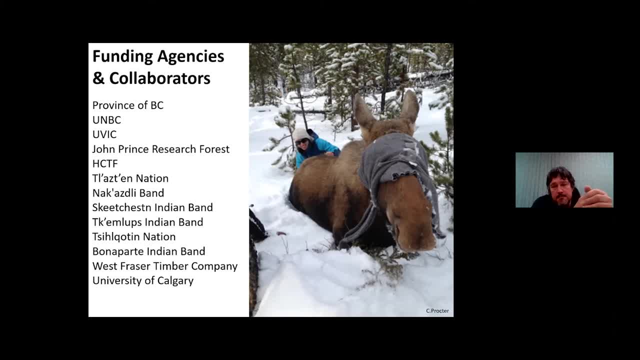 The data. I guess what they're saying here is: the data seems to start after the population crash, And of course that's why we have the project. So I guess I mean it's not there's a question, but there, well, there isn't really a question there. 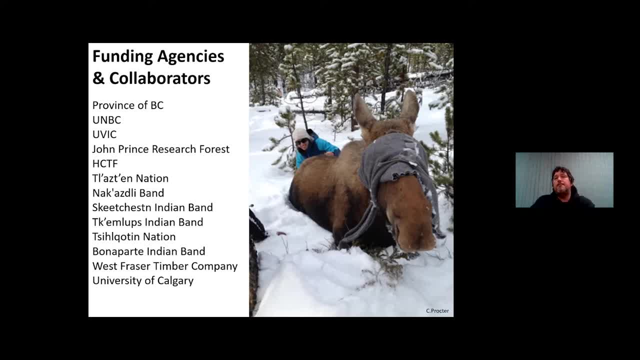 but really I guess the research started as a function of the population declining, So we don't have any pre, any really good pre-data, correct? That's correct. Yeah, it's really unfortunate Some of the analysis we are doing though. 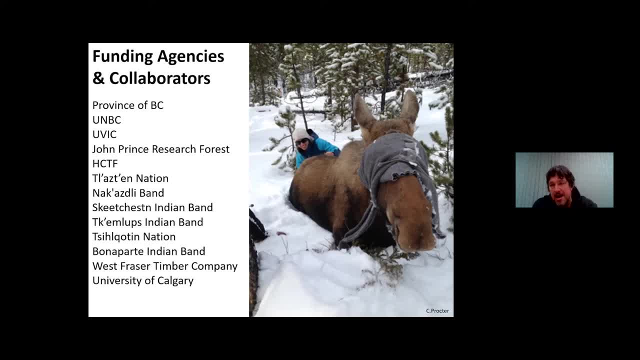 I think apply to you know, back during when the Maine declines occurred. You know, if we were to detect a relationship of landscape change and moose mortality rates, that same relationship likely holds true during the early years of this salvage logging era. 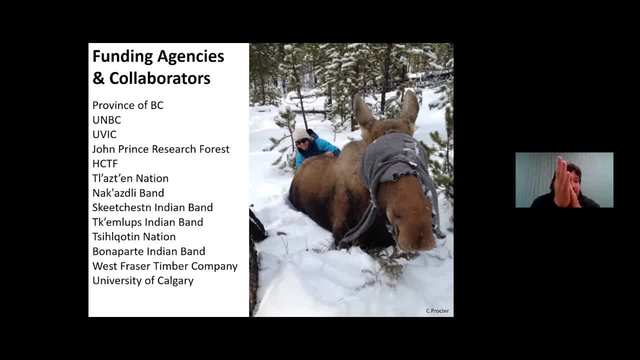 So the other thing to note is that these moose populations continued to decline through this research period. So some of those results are certainly applicable, I think. but you're right. I mean you're chasing around the cause after it's happened. 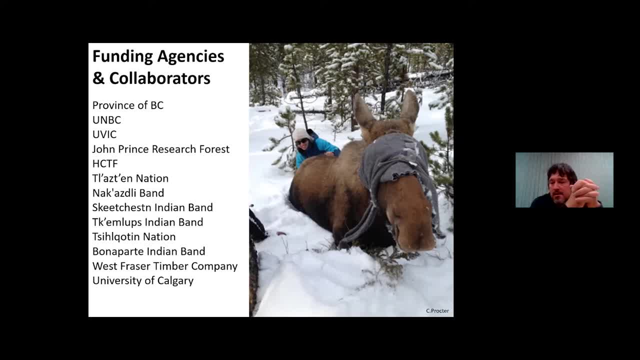 It's tough thing to do. I really wish we had some- you know, like we're you know- some data like, for example, on how fat these moose were at that time as opposed to now, that kind of thing. but, um, yeah, not much you can do about it at this point. okay, um, has there been any known? 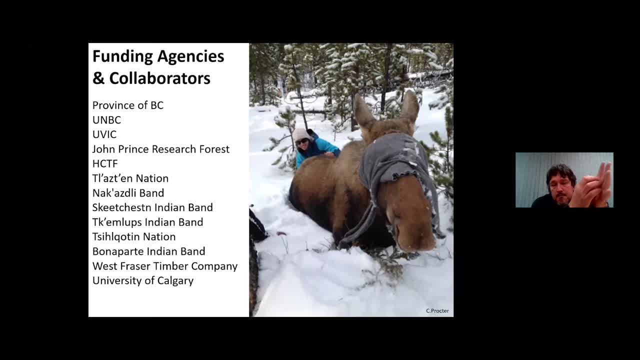 impact in predation levels related to increase in powered recreation during the winter months, or is it something that you're looking at? um? we are not looking at that here, um, in this project i i mean it's been demonstrated, you know, wolves using snowmobile tracks to get up into caribou. 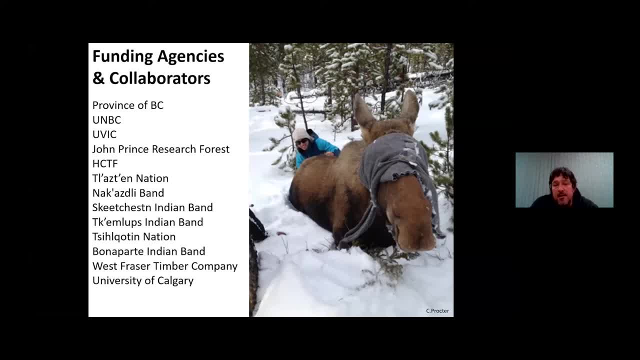 country or wherever it probably happens here too. um, it's a very difficult thing to measure on the landscape and, um, yeah, we're- uh, we're not looking at it here, but wouldn't surprise me if that effect exists. okay, um, this is maybe not one that you have, but it might be in a report. what was the percent of? 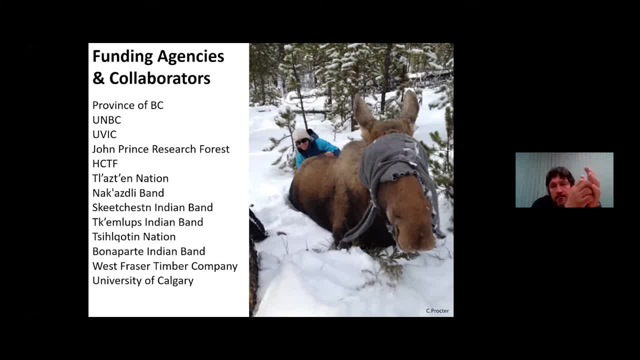 conifers in the study areas. i'm guessing you don't have that handy, but um, yeah, i don't know. um, well, like the percent of mature conifer forest, yeah, i think they're really dry. i mean, these questions drive at the composition of the forest and it's this deciduous versus you know um. 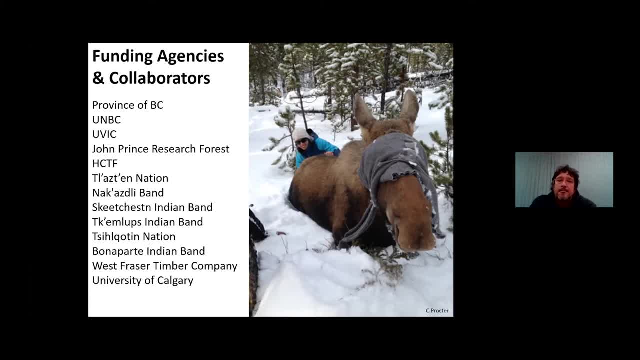 all the other, the trees that are planted. essentially, there's a few questions related to that. so any work done on on habitat in terms of forest composition, maybe is that what they're driving at. yeah, i mean, we've described these landscapes in terms of their proportions of 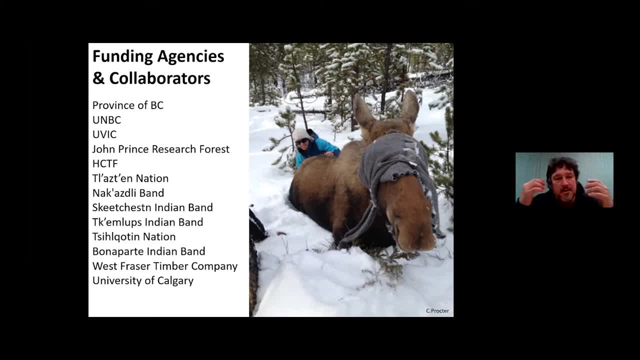 you know, mature conifer forest, mixed conifer, deciduous forest, deciduous dominated forest, that kind of stuff. i don't have those numbers handy, but they are presented in our progress reports. um, if anybody's interested, we'll get links out to the progress reports. um, now here's one around, uh. 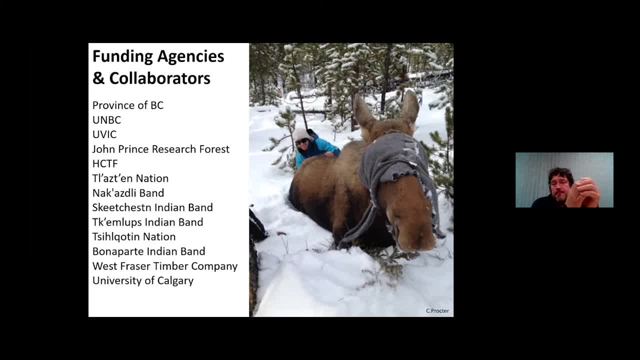 the question is: what was the exact fix rate for the high fix rate callers? and the reason they're asking is around mortality and movements just before death to establish cause of death. but maybe tell people what the high fix rate is versus the low fix rate. yeah well, they've been variable over the years. um, when we first started, like in the bona, 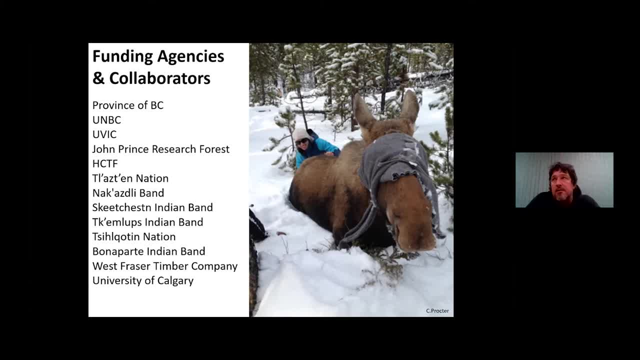 parte plateau study area. we kept that fixed rate pretty low, i think every 45 minutes just to give us more data on what that moose was doing, up until the point that it died. those callers, when you program them at that high of a fix rate, tend to not last that long. 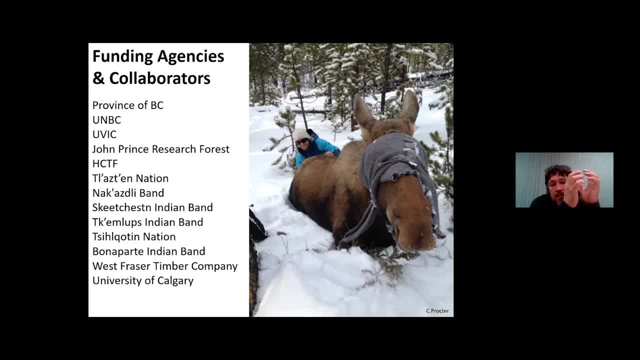 so there's a bit of a trade-off there. um, a bunch of the callers for the the last bunch of years have been at a four hour fixed rate, so six locations a day, and then for a couple years- um, we were we had put some collars on that- we're only collecting two locations a day. 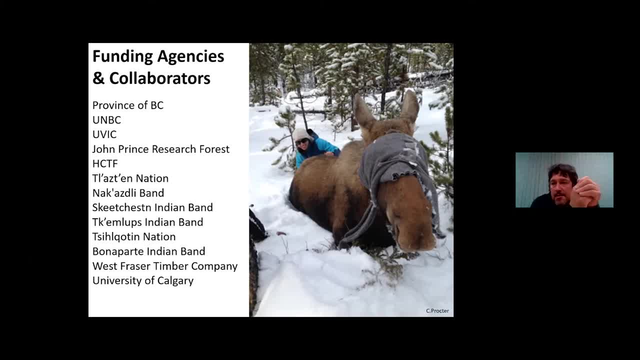 because we were interested in the broad habitat use from those moose and then simply whether they ended up dead or not, and there's trade-off with cost between these collars too. but yeah, any data on relative pregnancy rates in the different study areas? yeah, yeah, that data is in our progress. 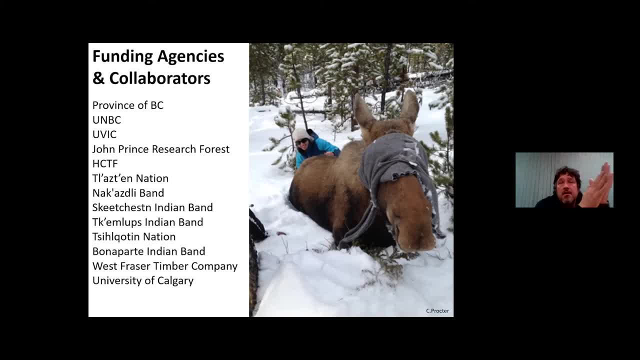 reports too. i did not present it here tonight. um it there has been some the odd lower pregnancy rate in a couple of these study areas. um, it's a bit difficult to interpret because it depends on how many moose we actually collared in that year. so there's some sample size issues there. 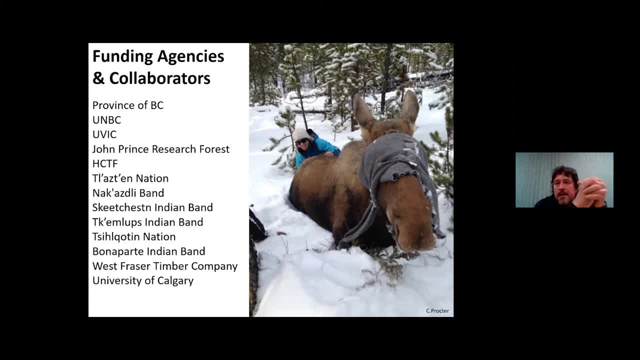 um, but yeah, anybody that wants to look. that data is in the newest progress report which, by the way, was just published last week, so it's available online. okay, we'll get a link for that. um, is there any data- i mean our individual analysis- any data on age of cow moose and its calves? ie is an older, mature cow moose better able to carry? 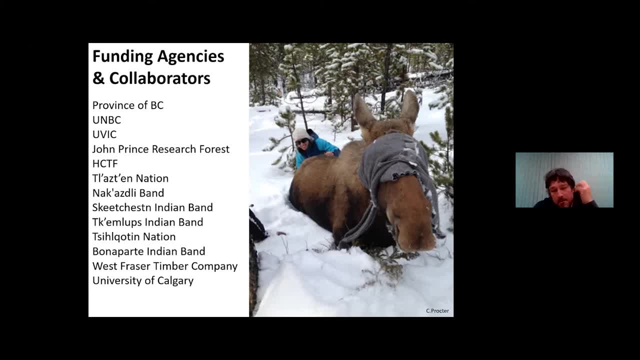 and protect and extend the calves lifespan? have you guys looked at individual demographics and that sort of thing? yeah, the problem is we're not sure if we're going to be able to do that in the future. we don't know um how old these moose are until they die, um. so, but that that deaf in the 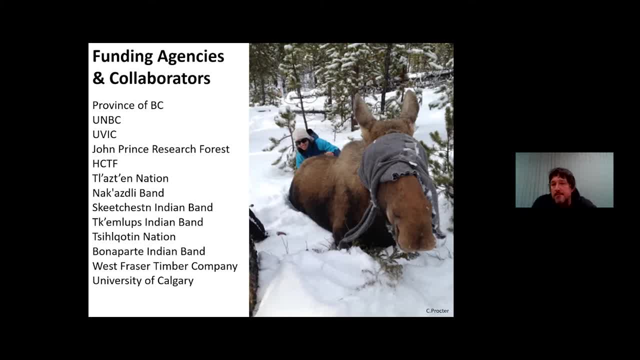 literature. um, we already know that you know a moose, an older moose is a better mother than a new mother, so that relationship definitely exists. gotcha, um, here's one. um, anything on climate change and the different factors, yeah, well, i you know, i think um there is potential for climate change to affect. 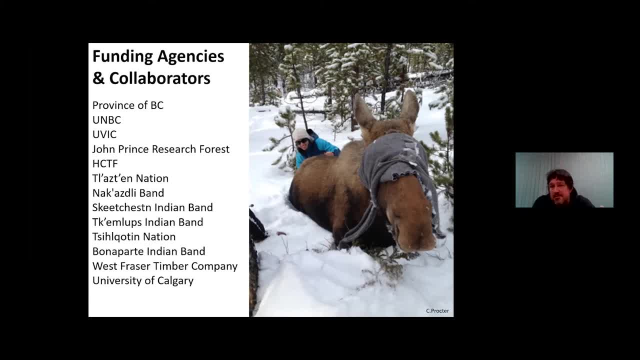 moose, like through thermal stress. so it's something that's being looked at for sure, um, forage quality would be another thing that may be affected by. you know, warmer, hotter, drier summers kind of thing. um, so yeah, certainly on the radar. um and um, yeah, we're looking at it. okay, uh. 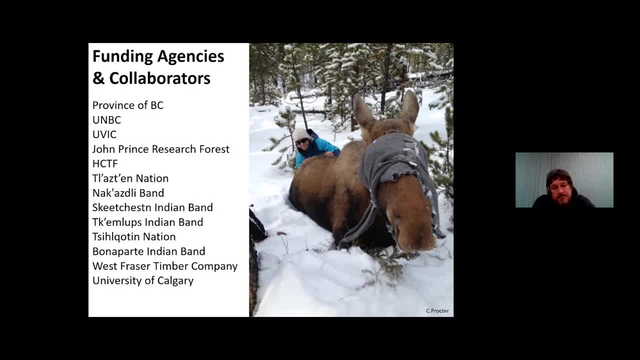 here's a question around the trade-off between food related carrying capacity and and reducing wolves. is there any indication that you're getting close to a food limited system, i guess, and so the question would be: if you manage predators and increase the moose population, would you run into? 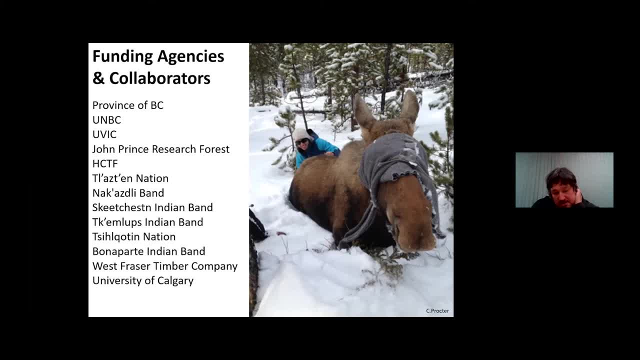 a food issue? yeah, that's a good question. um, you know, it's certainly we thought that these moose may not be in great condition. um, obviously, if, um you know, if predator management was to occur, i don't think there's any doubt that most of these moose populations would respond to that. how far they could respond would depend on. 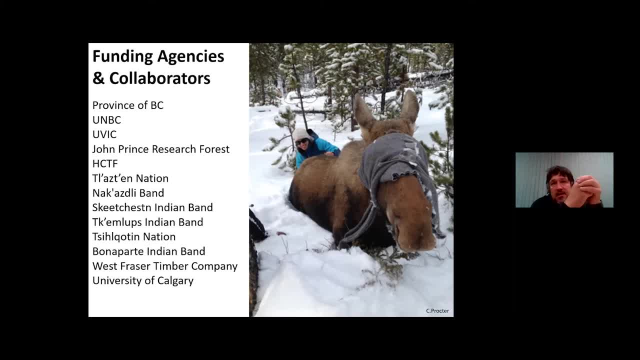 um, you know where how fat those moose are. i mean, obviously, as moose density increases, moose density increases. so i think that's a good question. um, you know, i think that's a good question. the moose density is fairly low in these places right now and, um, you know, our data so far doesn't. 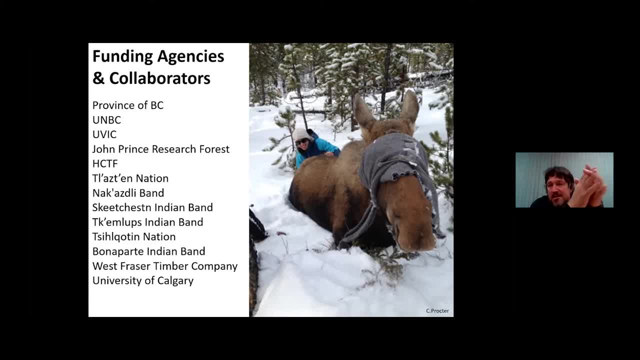 really suggest that there's an issue with their body condition, although, like i said, i think they could be fatter. um, how that might change as density increases is is, uh, something that should be considered for sure. okay, uh, this is a harder one. at what point are we at the point of serious concern, and at what point do we get to the point of no return? 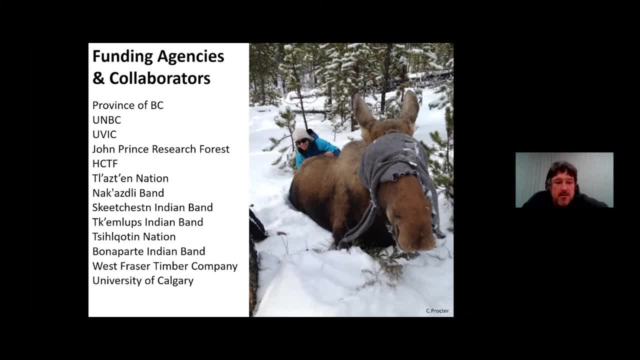 uh, we're a long ways from that. um, you know, in these study areas there's still hundreds of moose right um the bonaparte study area there's, you know, the latest estimates are 800 or 850.. um, certainly, um, you know, prince george, those densities are, you know, half of what they used to. 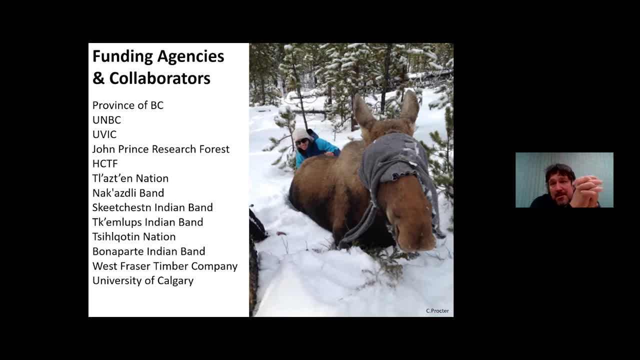 be, but, um, the densities in the past were pretty high. so i think that's a good question. i think they're pretty high, um, so yeah, i don't think we're at that stage here yet and honestly, i'd be surprised if we got to that stage. but yeah, it's hard to say. okay, here's another one for you, and 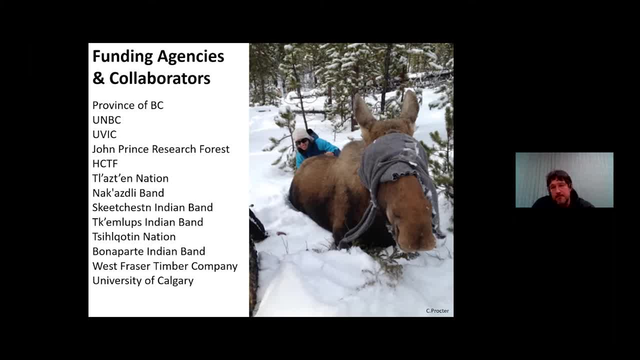 obviously not directed at you, but have there been any um management outcomes as a result of the research today, ie, has the ministry have there been any changes to anything related to access forest management, anything like that? yeah, another good question. um, not yet. i mean there's, there's been. 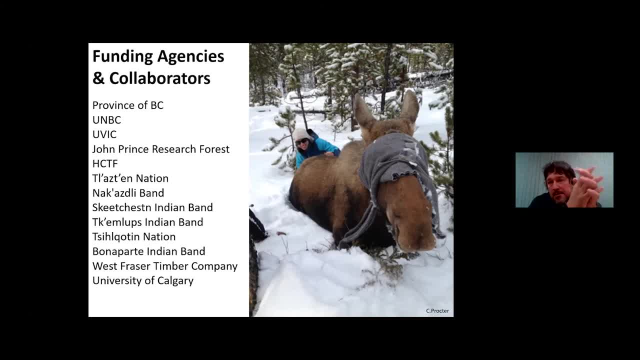 a few things. um, there's been some road rehab on the bonaparte plateau. that's that's arisen from some of this research. there is some habitat enhancement stuff going on in the prince george south study area in response to some of these results. but um, you know, i think um like i suggested. 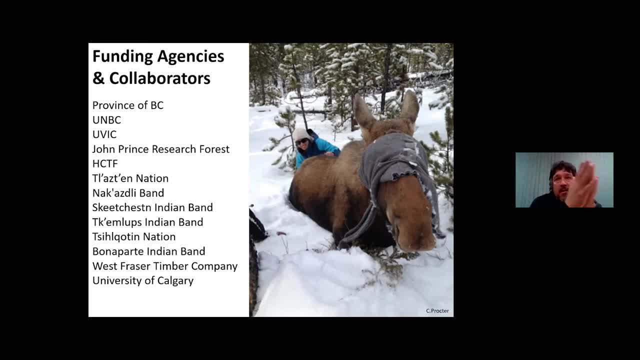 with my last slide there. um, you know, we really got to nail down the important things that are explaining moose population change and then generate those recommendations and and go for it. okay, uh, you mentioned how 85 of the survival rate for cows for a stable population. 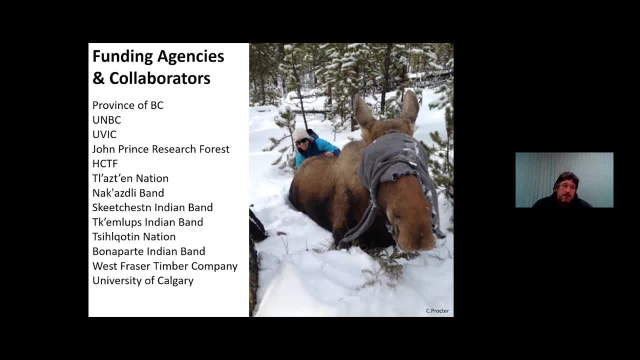 what is the calf recruitment rate and calf cow ratios that are required for a stable and growing population and where are we at relative? yeah, good question. um, generally, if you have a normal female survival rate, you need approximately about 25 calves per 100 cows at age one um. 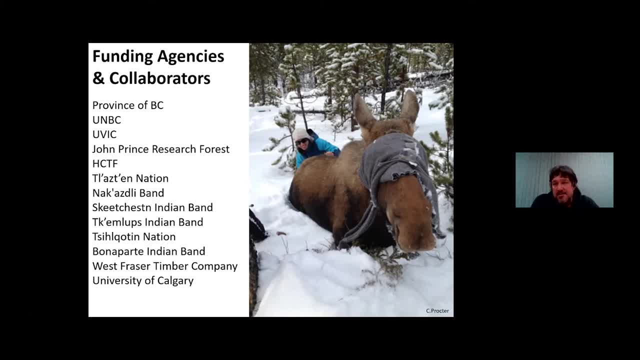 you know, in recent years we've been below that in a lot of these places, sometimes way below that for sure. um, and you know, given what we've learned about that late winter calf survival, you know we tend to see a lot of ratios- doing surveys right around that 30 mark. but given 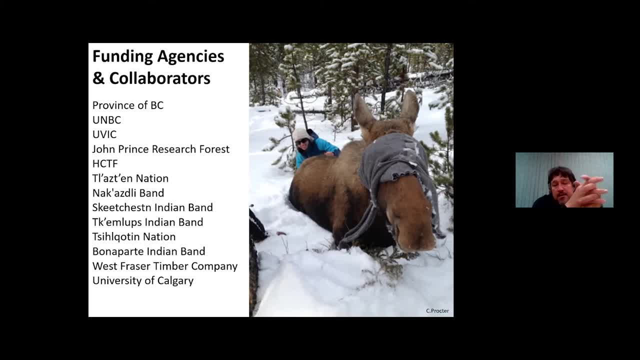 you know high probability of late winter survival. even if you saw a ratio of 30 or even early, you know low 30s mid-winter. you're likely going to be below 25 or close to that by the time they are recruited. so um long-term trend in some of these areas too has been 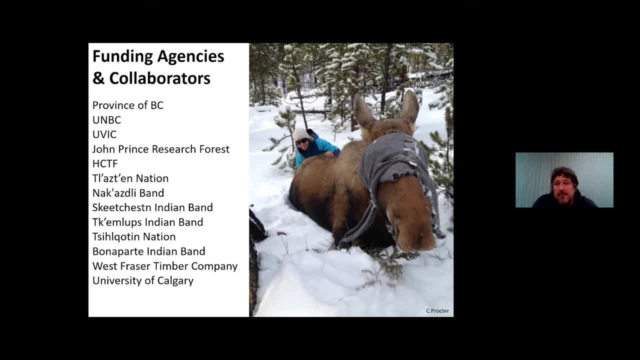 a longer term trend in in lower calf ratios. i mean take in bonaparte plateau for example. you know, back in the 80s, early 90s we would see ratios regularly over 50, mid-winter 50 to 60 kind of thing. lately they've been in the teens for sure, although better the last year or two. so 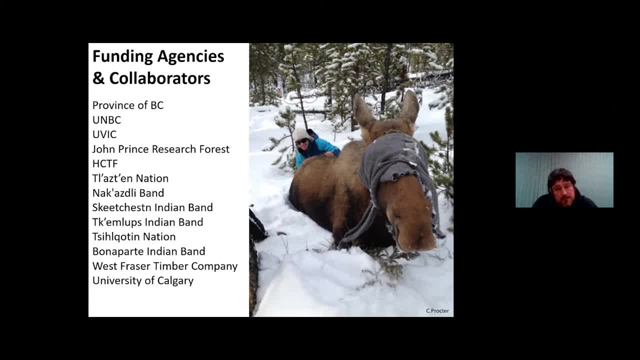 here's a quick one: uh, any discussions or literature around, essentially that pending for uh moose? no, no, we're not. we're not there yet. is there significant differences in the landscape composition from the uh indiaco study area versus the others? yeah, generally. um, yeah, it's been. it's the study area that's least impacted by forestry. 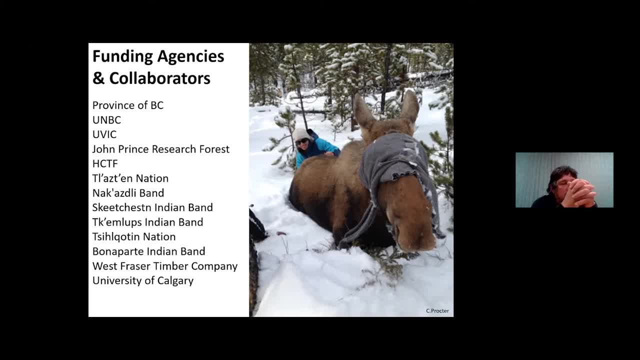 um, you know, our estimates of landscape change there, at least in terms of early serial young cup blocks less than nine years of age, was only two percent um, compared to bonaparte, which was about 13 percent. uh, there's some other fairly big differences there. big wildfire there a. 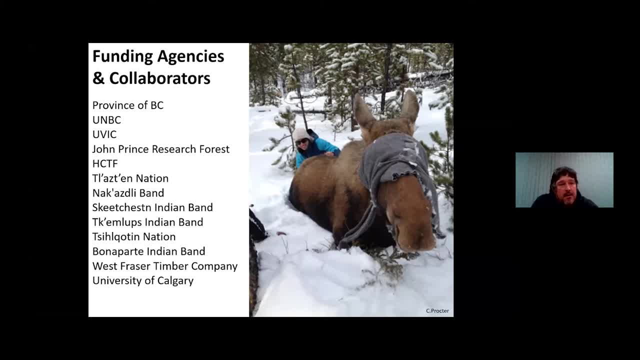 few years back. um, but a lot of it, um is is fairly intact. uh, you know, big provincial park there and um, yeah, quite different than the other study years. great, how long do you have any idea how long the study will continue to run? um, no, not right now. um, i think we have funding for two more years, so this year next. 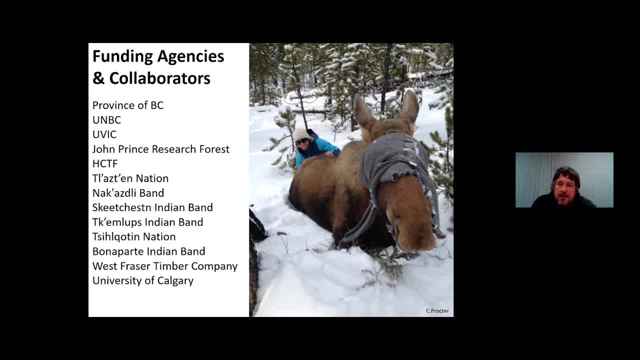 um, but it's something that we're definitely going to be working on going forward here, um identifying if you know what these gaps might be that we should spend our time and effort looking at. Okay, here's a good one. It seemed like the data showed out survival is half high. calf survival was generally decent in the areas where populations were declining, yet adult and calf survival was high. Was there any issues around the bull to cow ratios? 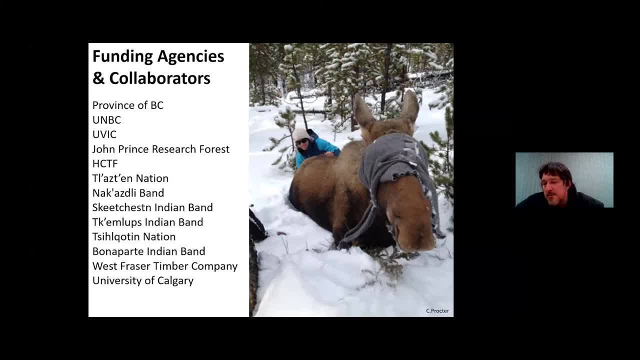 No, another good question. We hear that a lot. I don't know if I can tell you what the bull ratio was in every study area, but I can tell you that it hasn't been below our objectives much in any study area. I think one of the lowest has been the Bonaparte Plateau And you know our bull ratios there over the years are generally in the mid to high 20s. 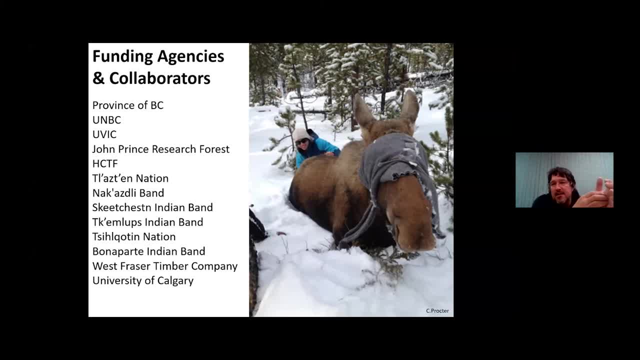 So a little bit below the objective. We've not seen any evidence that that impairs reproduction for moose. The first indicator of that would be the rate of second estrous pregnancies, And it's been really low: 5%. over hundreds of calving events over the last, you know, over the years that we've been doing this project. 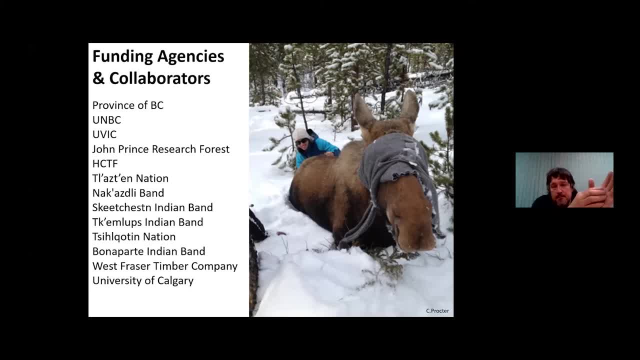 Thanks. Any idea why the capture population Age is greater than the estimated average age? Yeah, another good question. I might not have explained that well. We believe it's related to a long term trend and lower calf recruitment. So as there's fewer young moose coming into the population, the average age tends to go up, And I think that's what we've been seeing there. 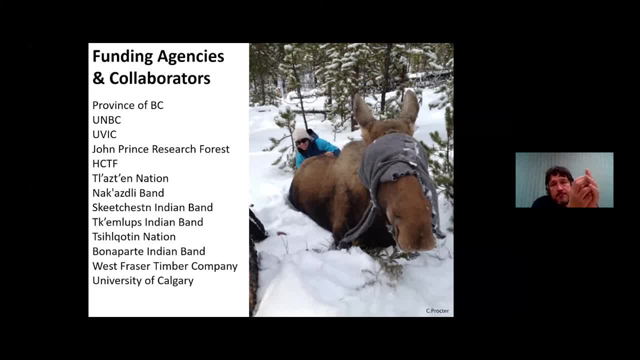 Gotcha, Now you already talked about timeframes around. the studies are getting published. That's good. So have you determined what the average winter range sizes were for the cows And has there been a comparison on how home range size compares to habitat conditions, especially around salvage and forage? 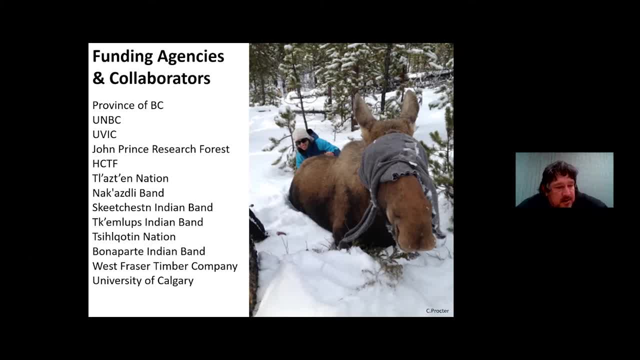 Yep, Yeah, there's been some of that work done and it's reported in those theses from UMBC and UVic. I can't remember what the average seasonal range is. I want to say it's, you know, 10 square kilometers roughly, But that data exists in those, in those publications. So there was a difference across study areas too, Likely reflecting productivity and that kind of stuff. The last forager is on the landscape, the further a moose has to go and find it. 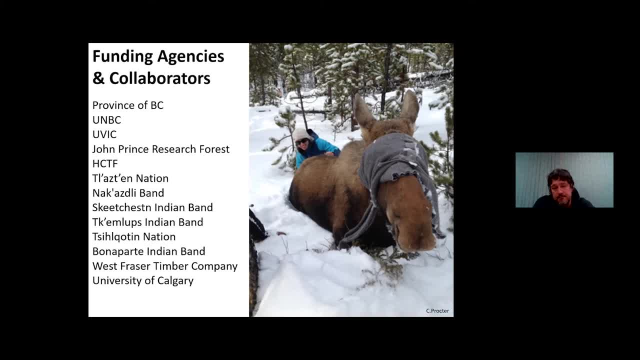 Okay, a few here related to: is there anything around possible competition between uh cattle and moose? uh, they tend to eat two different things. um, most part, cows will eat moose forage if we if docking densities are too high or they're left. 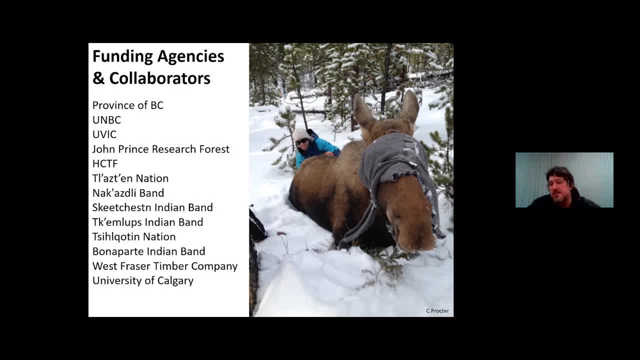 on the range too late into the year, that kind of thing. so there definitely is potential for issues there. we've seen evidence of it in region three. often those issues are associated with road densities too. so cows are lazy- um, you know they- if there's a road that takes them to this patch. 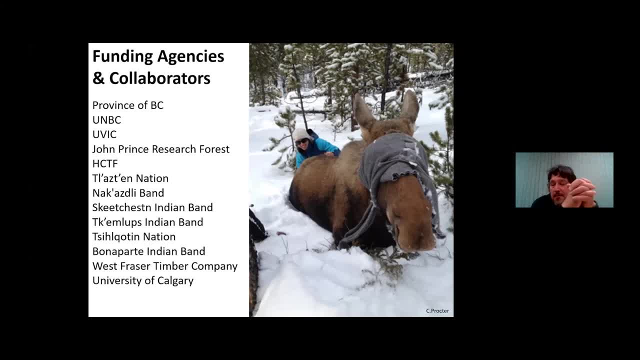 and we sabotage, they may end up there and they may cause an impact, but it's a tough thing to measure on the landscape, um, to do an analysis at the scale that we are. so it's we're not. we're not doing that, okay, uh, is there anything around? predator link to parent competition. 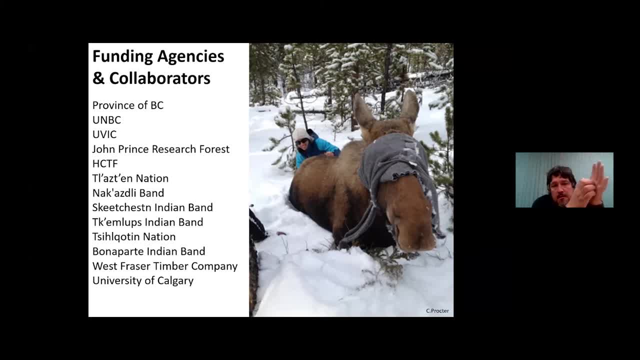 uh, increasing whitetail, deer and predator numbers, that sort of thing. oh man, i mean, if you increase the number of ungulates on the landscape, you probably are going to have more predators, right? so they're. um, i think most of these systems that we're working in are moose wolf systems, though i think that's the main relationship that occurs there. 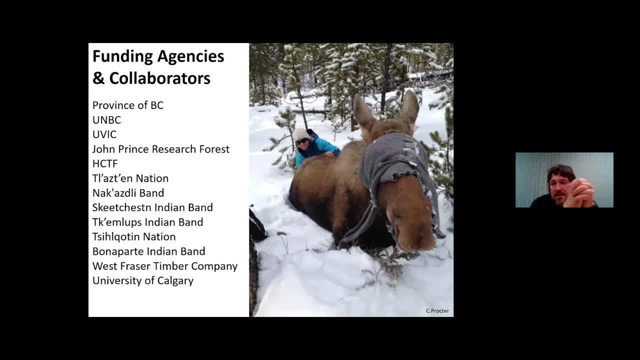 um, and yeah, there's potential for it, i suppose. okay, uh, anything in the literature around the effects of motorized recreation on cortisol or stress levels? yeah, i imagine there probably is, but i don't it's a tough thing to measure on the landscape again, when it occurs, how often it occurs, that kind of stuff. 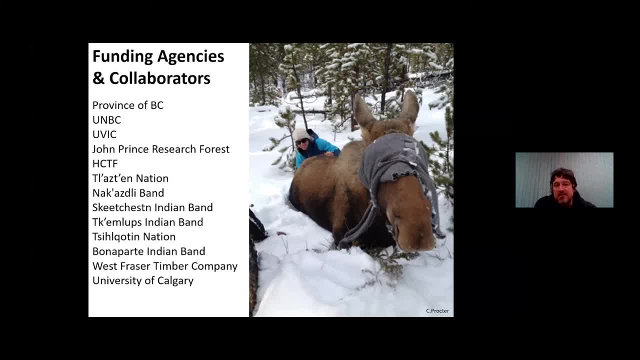 um, but i would bet if you could measure that that relationship probably exists. okay, uh, anything around thermal coverage and snow interception, around logging and lack of mature timber- certainly on our radar. this is some of the thermal stress work. um, yeah, i think it's a factor that we are thinking about, for sure. 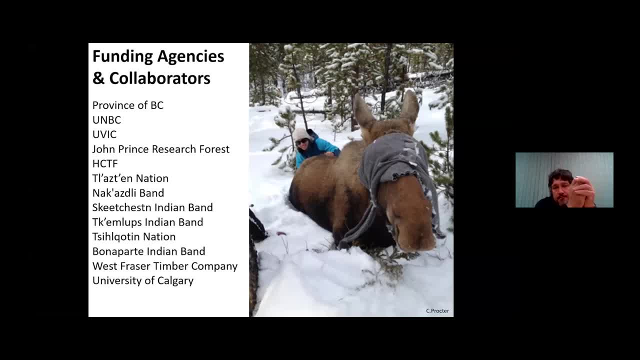 gotcha a lot of wolf specific behavioral questions. any idea around? i mean, do you have many wolves that are collared and how far are they going? you know what's their territory or their home range look like? well, they're pretty wide-ranging animals. um, we do not have wolves collared in most of these study areas, although there are some. 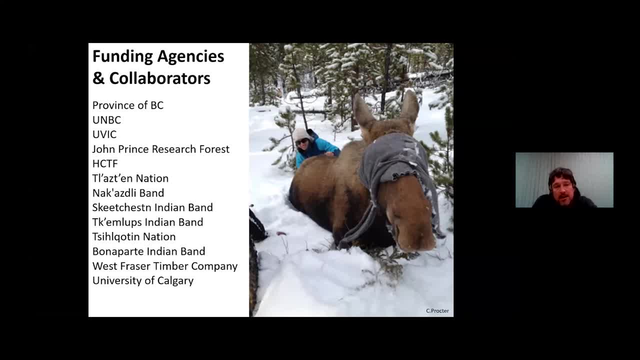 collared in the prince george show study area and, i believe, in the anti-aco study area too. some of those results are going to be forthcoming here. um, not too far down the road, gotcha. can we reverse these trends by allowing more deciduous and regenerating cup blocks? 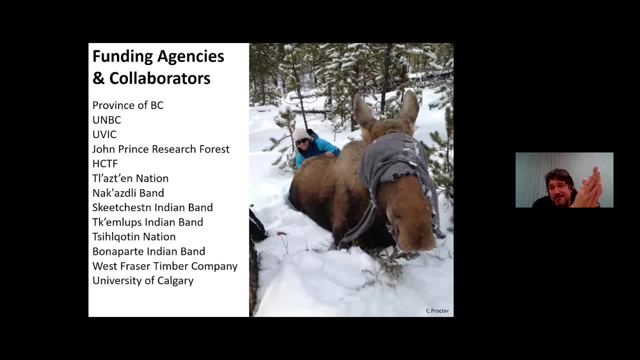 uh, you know what? i i doubt it. i i don't think that's the thing driving these systems, but, um, it certainly may help though. uh, yeah, thanks, uh. now moving over to some more questions, any indication around, or is there anything in the literature around coyotes and neonates? 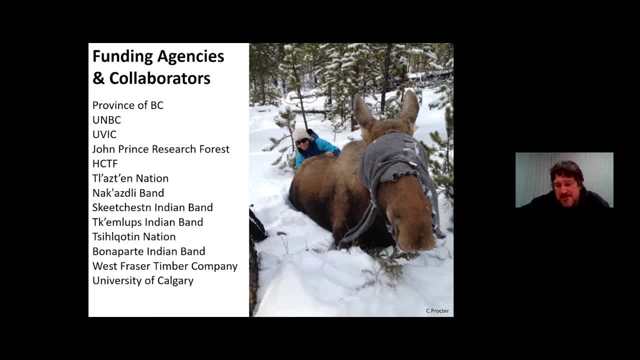 um no, yeah, i believe there's been instances of predation, actually by coyotes. um yeah, it's, i think it certainly happened. i don't think it happens a lot gotcha. uh, do you have any estate estimates on wolf densities in the study areas? um no, we do not, unfortunately. um 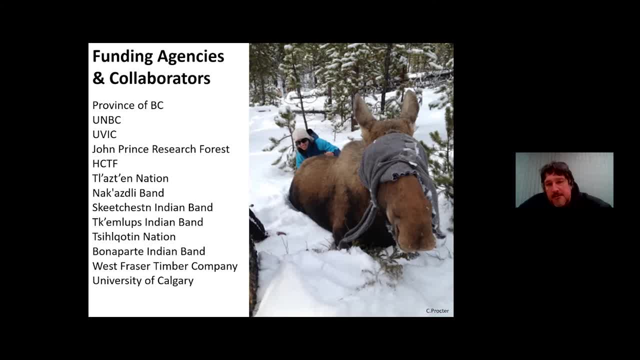 we have rough numbers in some places depending on the wolves that we've seen. i mean, we spent a lot of time in these study areas, um, but no actual survey based wolf density information, unfortunately right, yeah, another one related somewhat to predation, but the question: is there any other? 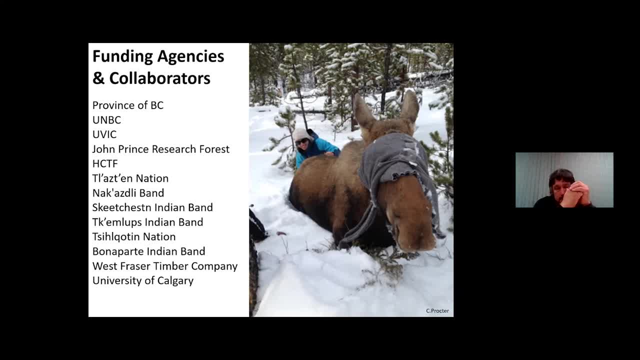 data besides body fat and bone marrow fat that may be predisposing most to predation. uh well, i think age generally- i mean the the three factors that i've that i spoke about tonight- are all potentially may contribute to predation. i you know, i think a moose has to be older. 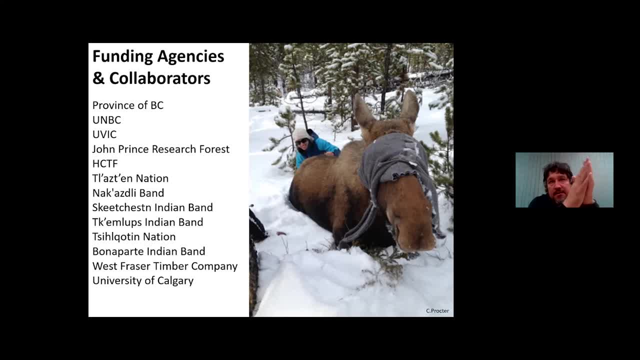 than the age, that, the average age that we've seen generally for that to occur, but um, their health and their ability to escape predation would be another one um, and then their condition is also one um, and i, you know, i think the landscape change um, stuff that we're working on right now. 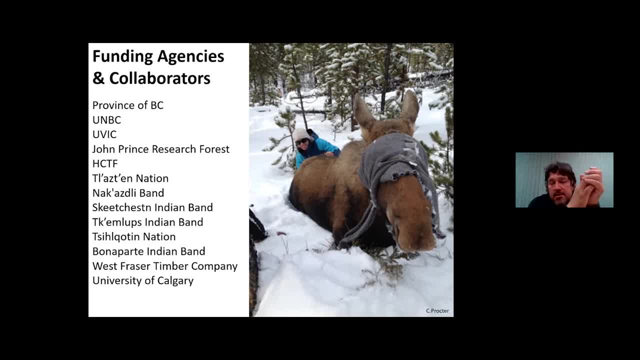 is another factor that may contribute. um, and those, yeah, we're still working on it. so, um, um, okay, uh, this is a good one. any response from the wildfires that you've seen any effect on moose populations in those areas? um, i can't really speak to entiaco, the only two real study. well, i, 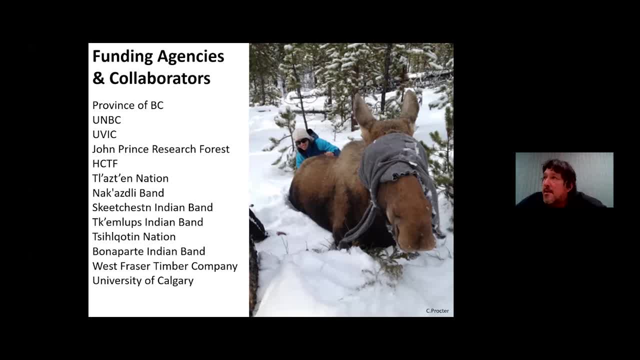 think there's. there's some fire in the pg cell study um in the bonaparte- we haven't seen it yet, you know, with the elephant hill fire which covers a pretty good chunk of the study area there. um, we've not seen it yet, but it's only been a couple. 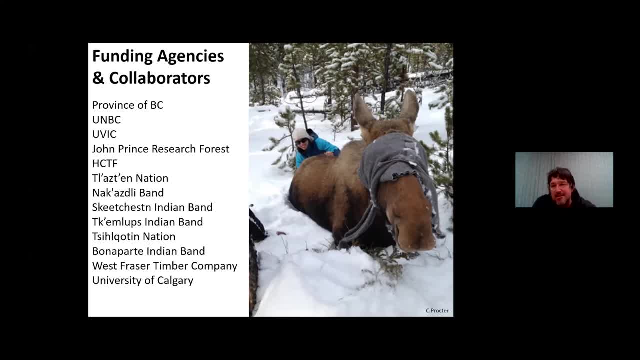 years, so i can't really speak to the other studiers gotcha um, here's one uh talking about a deactivation project on west fraser and in the jameson um. is there any indication that that that deactivation is yielding uh response yet? yeah, it's something that i think we're going to be looking at. 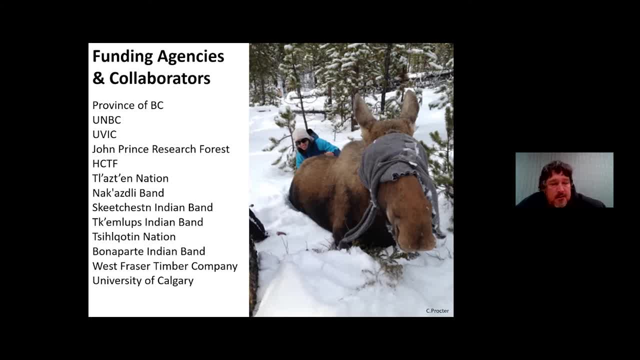 here because we have data from collard moose prior to that road rehab stuff up in that area on the bonaparte plateau, um and following. i certainly have seen moose use places there where i have not prior um. so i think that they are, i think it's it's. i think it's helping for sure. 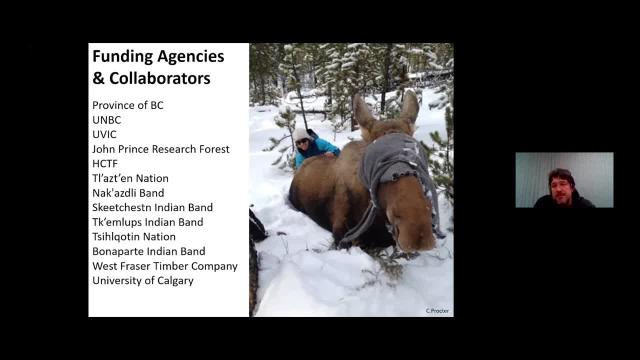 um, but we got to do the specific analyses. yeah, awesome. uh. now there's some talk uh questions around uh competition or issues between moose and feral horses, i guess in the chill colton area, anything on that or anything in the literature. well, i can tell you that moose do not like those horses. 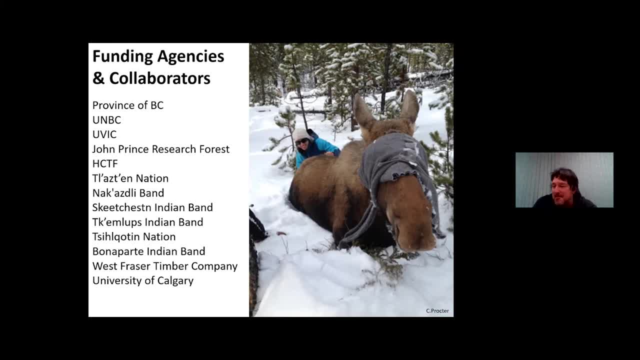 um, i, i think they're. you know, i think there could be some displacement issues there for sure. um, i've done a bunch of the moose captures in the big creek study area where there are a couple thousand or more feral horses, and they're not really good at that. they're not really good at that, they're not. 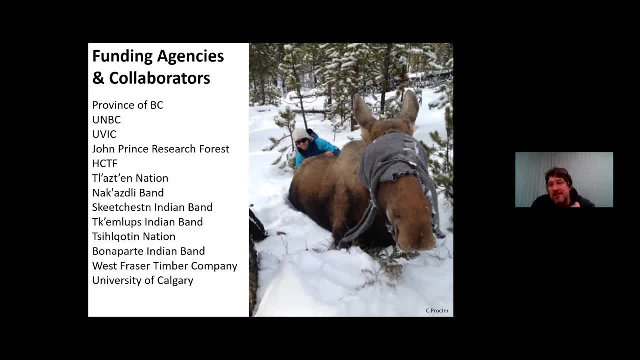 actually, one of the issues i think we need to look at is whether there's a place within the um genre where there's more bad produce to pass the system down to, when people can't do that, or where they can't do it by outstandingist means and um, then we'll what jim may need to improve. 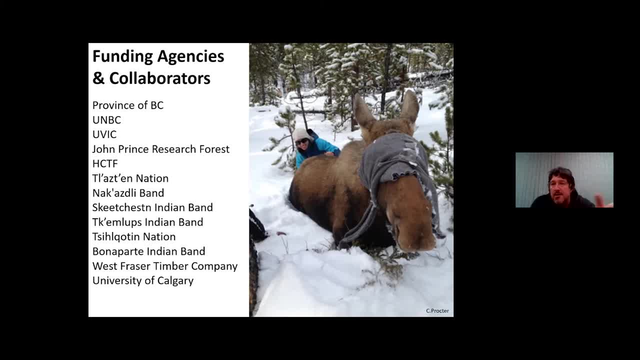 on is the use of these e Потому es eine der rescuevillen und um consequ auf shearpflege. um that means, can you have these spaces, you build them up and put up it in nil by retraining that it does some work um. we spent three or four years. we were spending a ton of time on these. 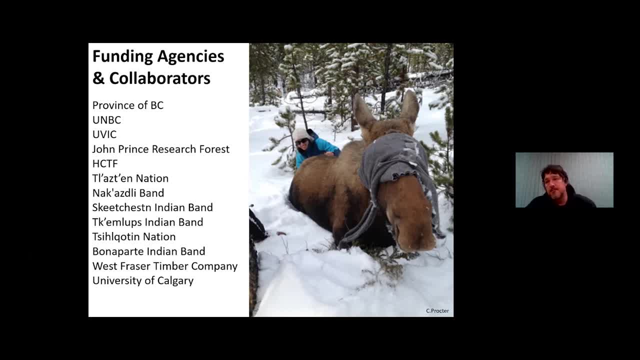 one. the length of the time was about 50 to 60 meters. i mean almost an hectare a day, and it's sort of a range. that was救iker怎麼 возaner i? i guess it was something that you can. you know. four years had you. 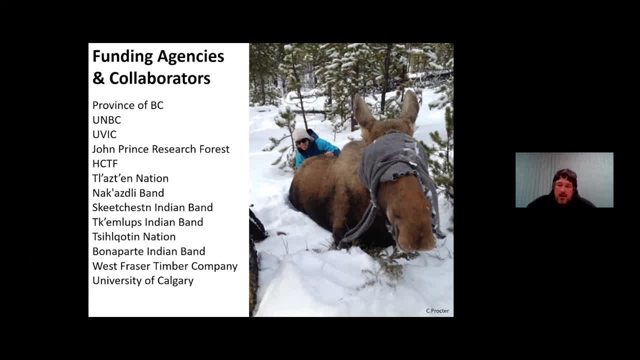 you know 40 year old cattle and just creamy, clean and color was 10 years ago. you know 150 or 90 degrees of the second estrus. Oh yeah, another good question. So moose most ungulates moose in particular. 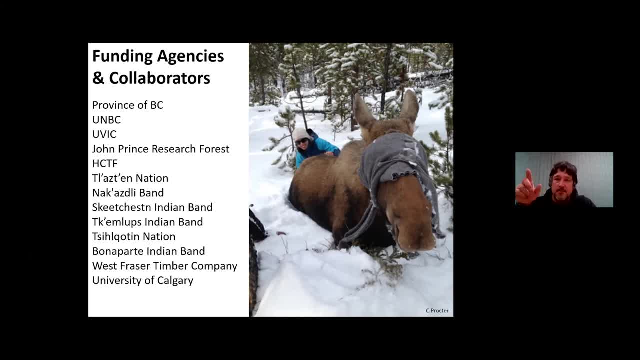 if you analyze their daily movement rates through the parturition period, it's pretty evident when a moose has their calf, Often, you know, you'll see a moose doing its regular thing, you'll see a long distance movement to some calving site and then you'll see a reduction in movements. 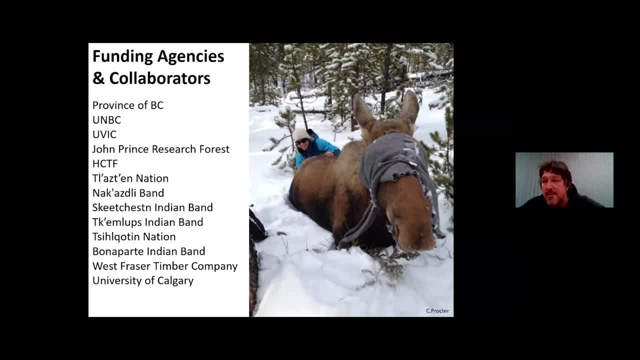 to almost nothing for a period of days up to a week or more. So we have estimated the birth date of every cow that we've monitored since 2012 in the Bonaparte study area, and then it's just a matter of looking at the date. So, like I said, of 100 calving events or several, 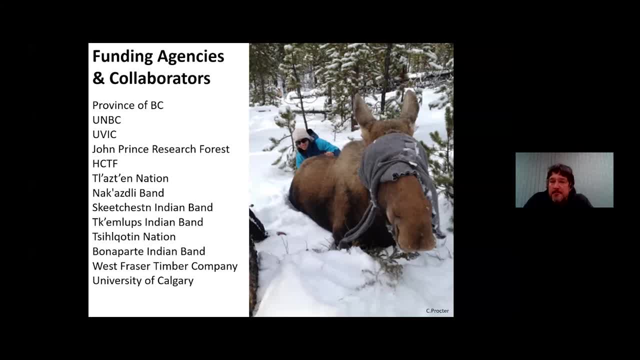 I can't even remember the number, a couple hundred anyways. Yeah, I think we saw like five, maybe six second estrus events. Thanks, awesome. A couple of questions now we're on the last slide around funders and collaborators. I guess the question is what kind of participation or 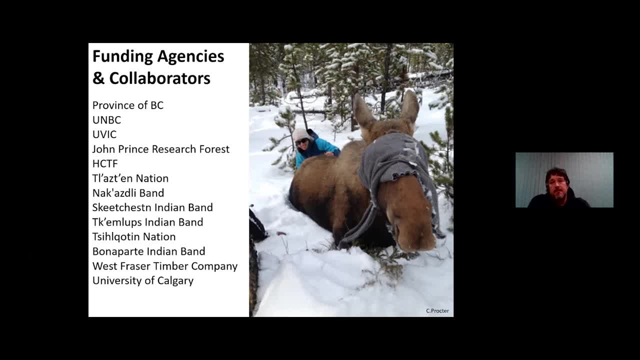 work has involved the First Nations around the project? Yeah, good question. I know they've been out working in the field in some study areas In the Bonaparte at times. for sure They've contributed funding to this, which is the case for to Kamloops Indian. 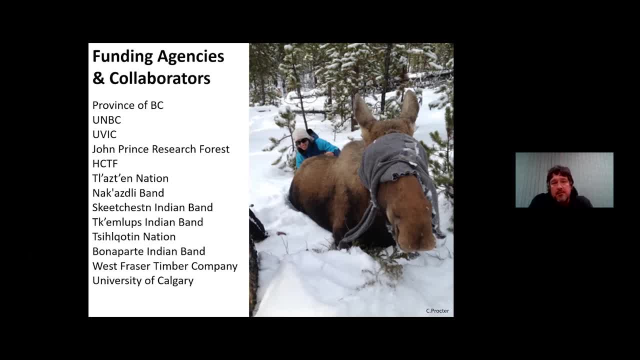 Band and Skeecheson Indian Band in the Bonaparte study area and I'm afraid I can't speak to the level of collaboration in these other study areas. Right, yeah, What so? what is senescence? So what mean age? do cow moose generally stop reproducing? Yeah, so they definitely do senesce. I think it's after you know. pregnancy rates start dropping after about 11,, 12,, 10, 10 to 12, somewhere in there. Yeah, They wouldn't stop. The pregnancy rates generally get lower as they age, But that's when the main 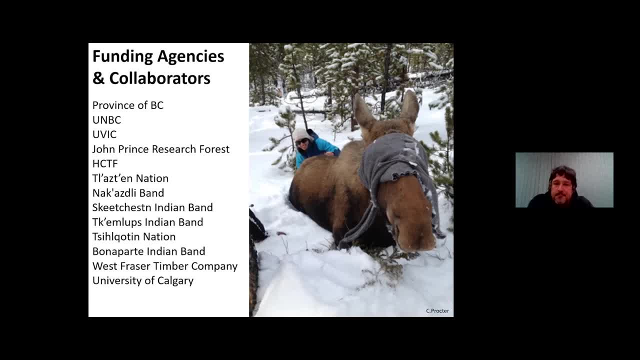 changes start occurring, Gotcha, Okay, well, I still have a ton of questions and questions rolling in. We will get the ones that we didn't get answered answered and we'll get them out, And maybe, Chris, what we'll do is we'll get a.